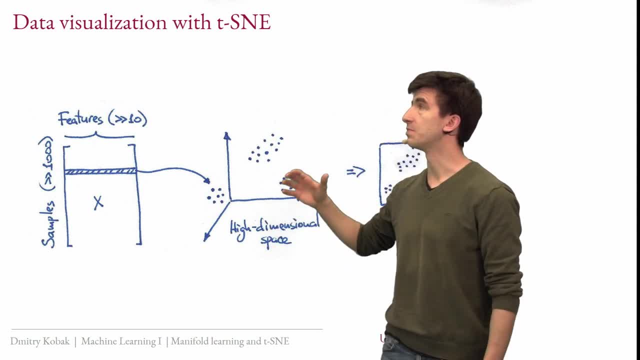 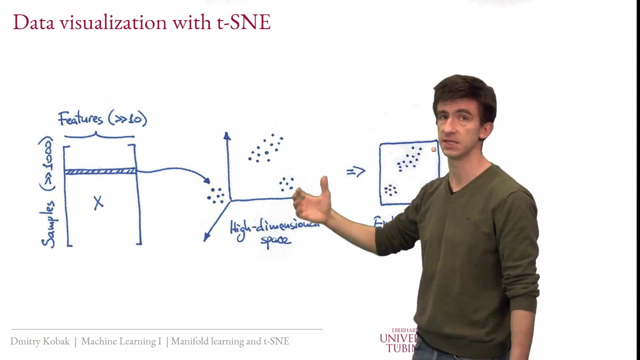 into two dimensions to preserve some interesting structure in this data. So, for example, if the high dimensional data have three clusters- well-separated clusters, like here, then we would ideally want to see three well-separated clusters on the embedding And again ideally. 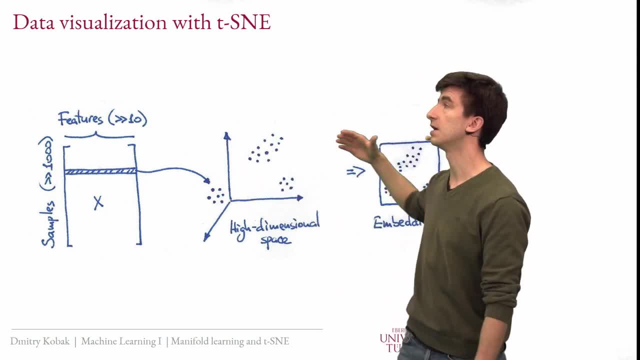 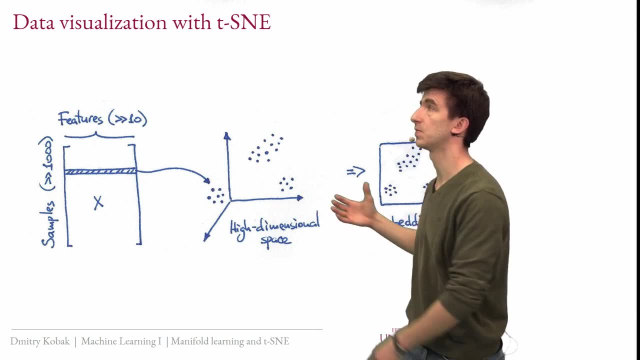 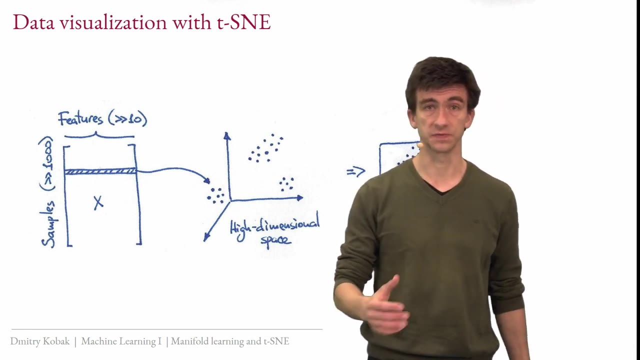 if there are some more complicated structures present in the high dimensional data, we would like to see these complicated structures In the embedding as well. Not everything can be preserved, but we would like to preserve as much interesting structure as possible. So this is the task of TISNI and of today's 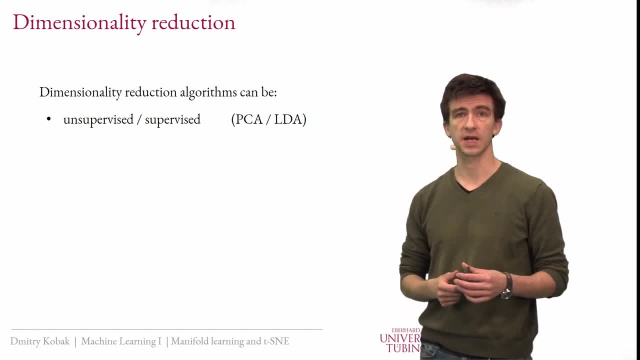 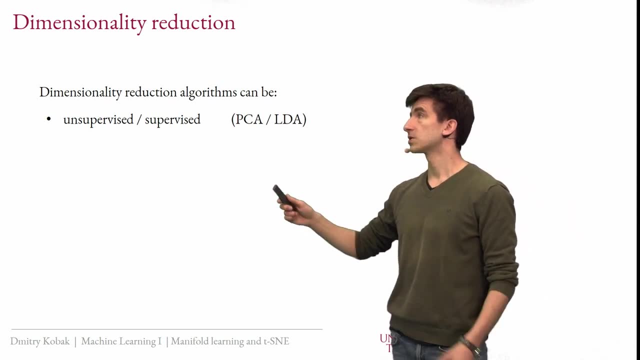 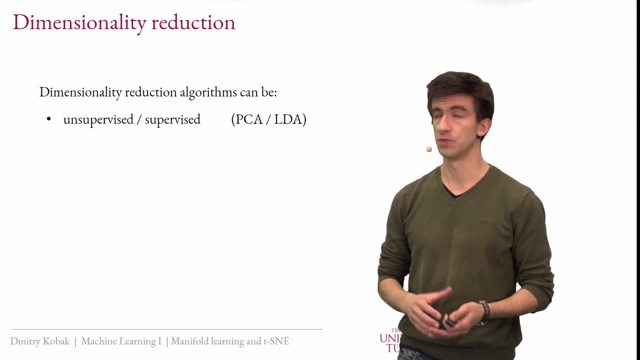 lecture. So let's talk briefly about what kinds of dimensionality reduction there are, how we can classify dimensionality reduction algorithms. So the first possible classification is that the algorithms can be unsupervised or supervised. Most of the time when we're talking about dimensionality reduction, we operate in the 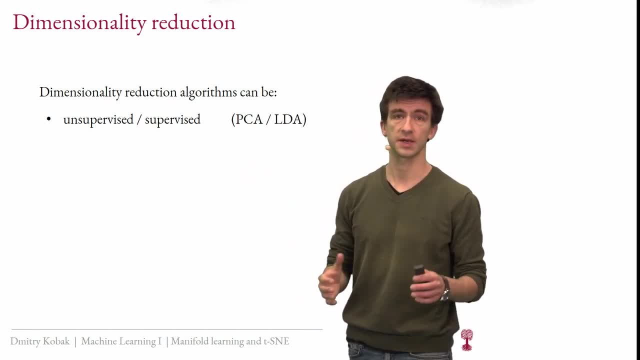 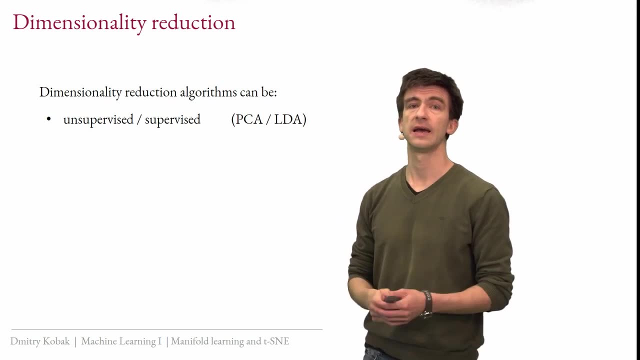 unsupervised setting, for example PCA from last week. But one can in principle consider supervised dimensionality reduction. for example, linear discriminant analysis that we discussed earlier in this course can be understood as finding linear projection that maximally separates classes right. So this is in some sense dimensionality reduction that is guided by the class labels. 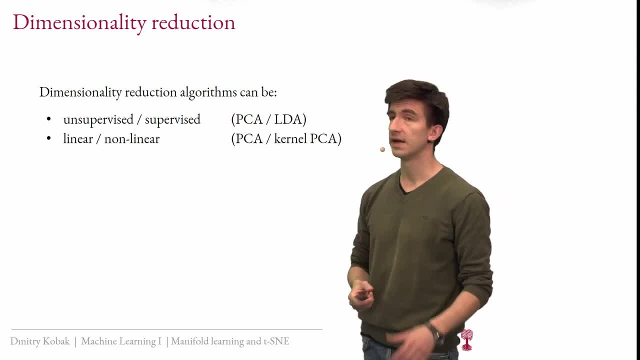 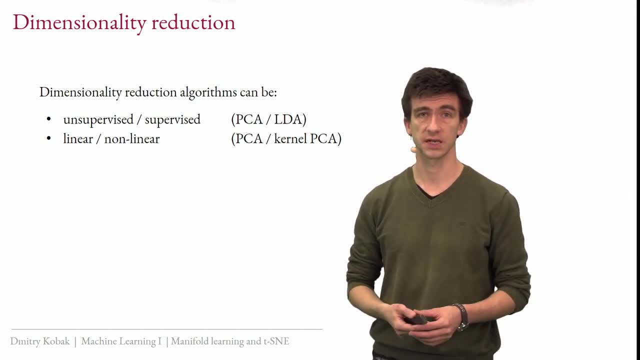 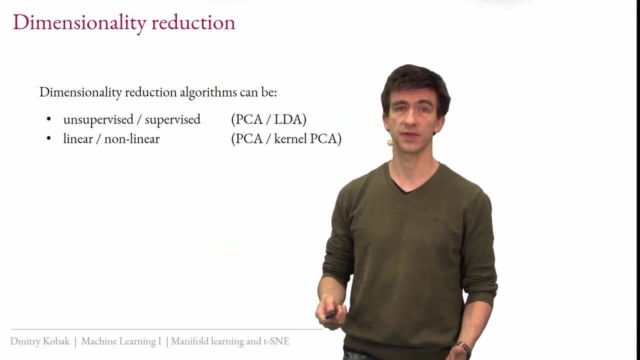 So this is a supervised reduction. Another possible distinction is between linear and nonlinear methods. So PCA is a linear method because in the sense that we're projecting high dimensional data onto a subspace, So projection is a linear operator, as we discussed last time. In principle one can imagine nonlinear. 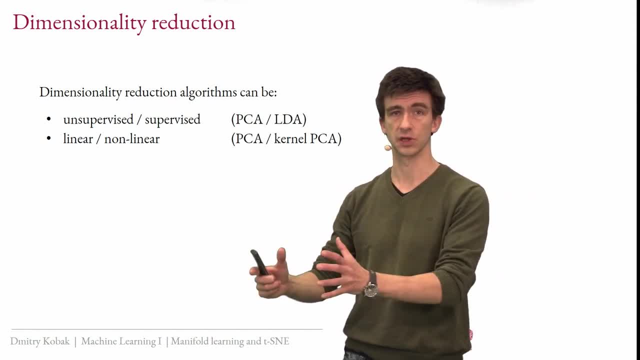 methods where the mapping from the high dimensional to the low dimensional space would be nonlinear. So this is a very specific example of nonlinear mapping and this is something that I'll talk about in the next lecture, but this is something that I hope you'll take into consideration. 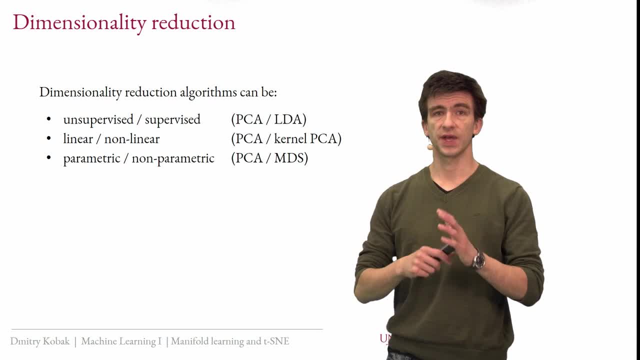 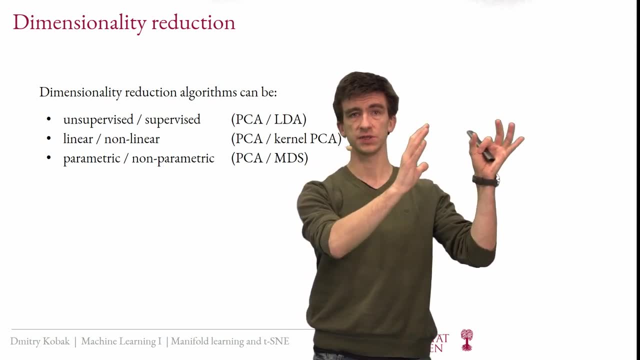 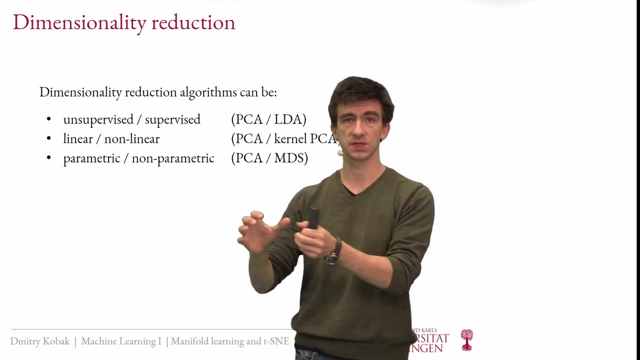 as far as this comes to mind. And finally, there are methods that don't construct any mapping from the high dimensional space to the low dimensional space. So imagine you have all these points in the high dimensions and you're trying to position the points in two dimensions, such that some important 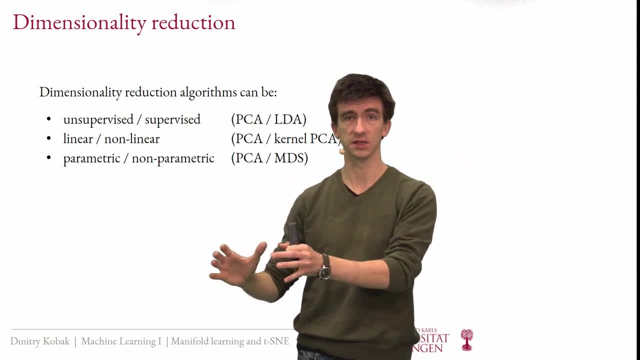 structure in the high dimensions is preserved in this embedding. This is something that I will be calling nonparametric method. No, we don't have that method. Yeah, Yeah, We don't have that method. We don't have that method. 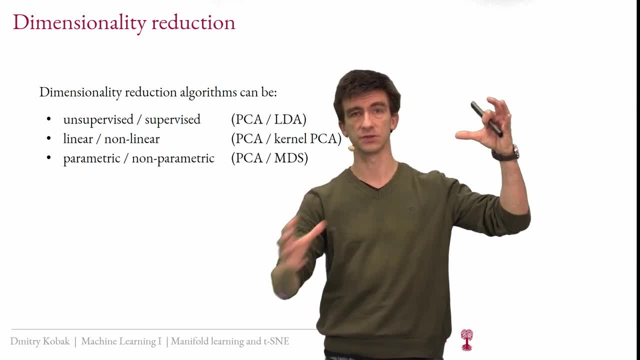 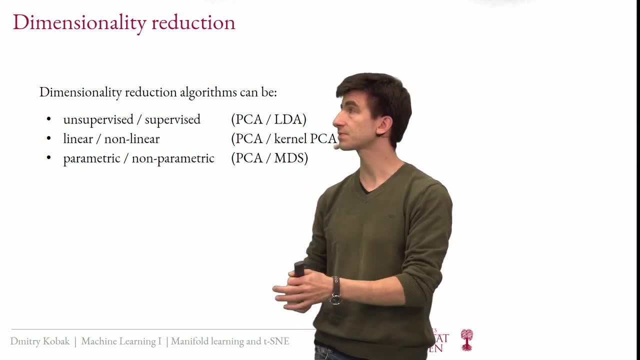 We don't have that method, So we don't have that method, So we don't have that method. never construct a function, explicit function, that maps high dimensional to low dimensional space. Instead, we're just optimising low dimensional positions of the points directly. 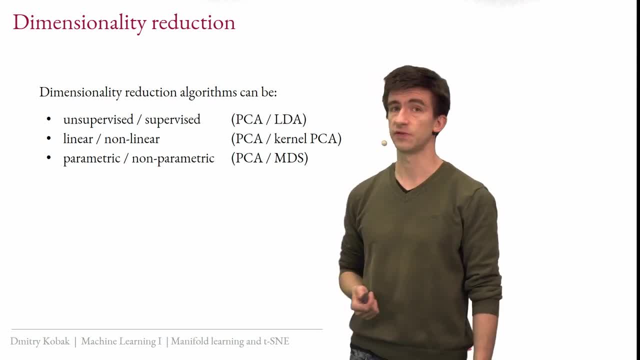 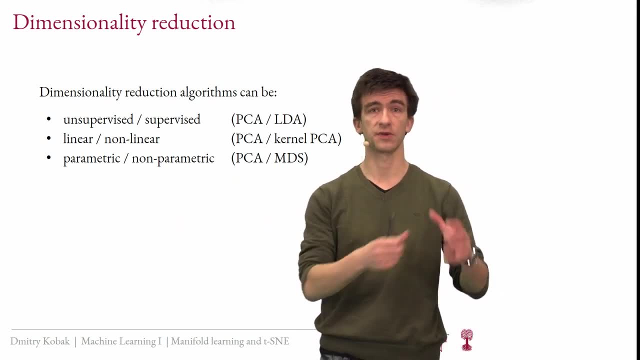 In this sense this is a nonparametric method. so I give here an example of multidimensional scaling, which I will introduce in a minute another example of that. but PCA, for example, is clearly a parametric method because there's a function making high dimensional data to 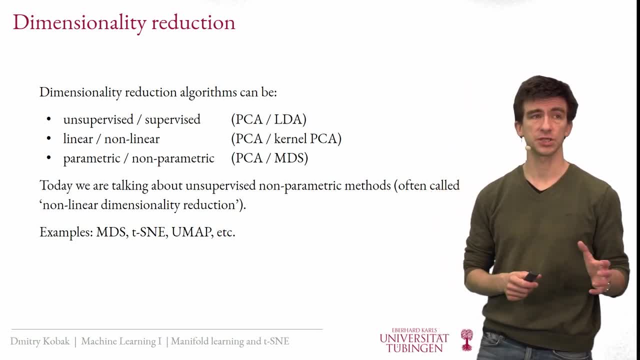 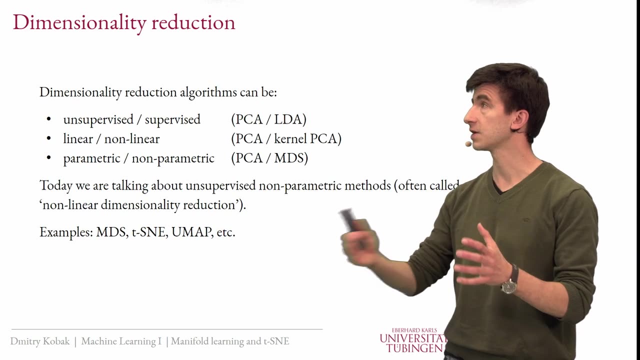 the low dimensional data. Just a note on terminology: often in the literature, these methods that I'm going to talk about today, such as t-SNE, are called nonlinear dimensionality reduction. I find this a bit sloppy, because there's no mapping, there's no function that can be linear. 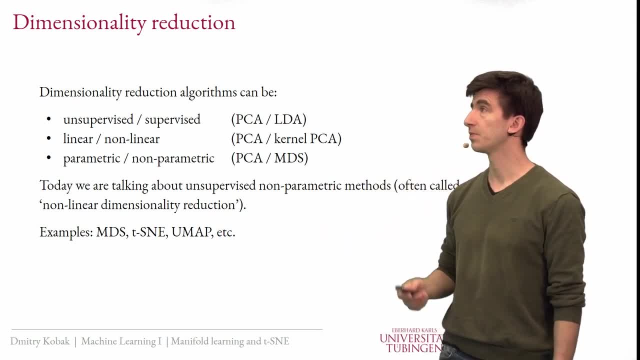 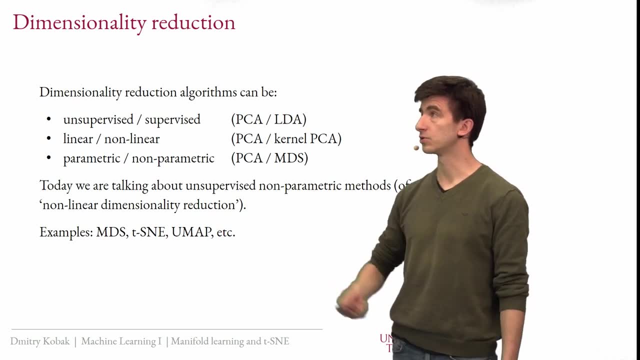 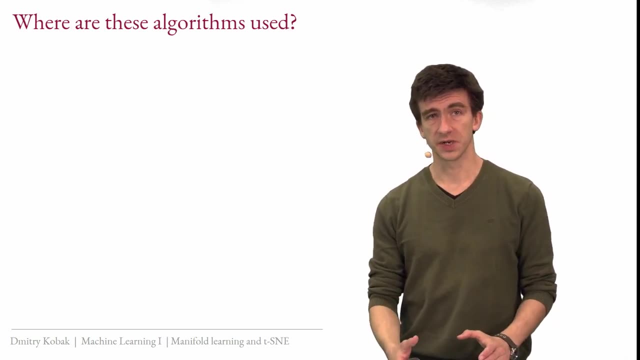 or nonlinear at all, so I'm not a fan of this term, but they are often called like that, And examples of these methods are multidimensional scaling, t-SNE, UMAP- a more recent algorithm- and actually many, many others. And before we really start talking about the nuts and 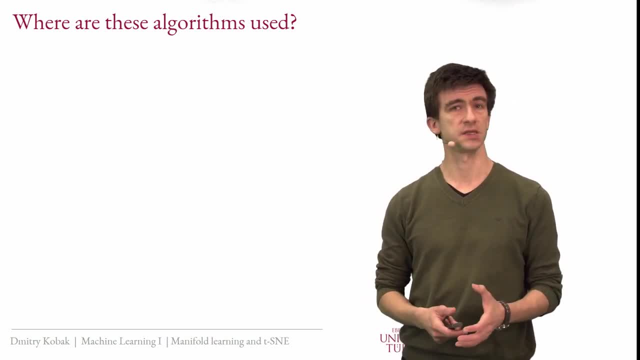 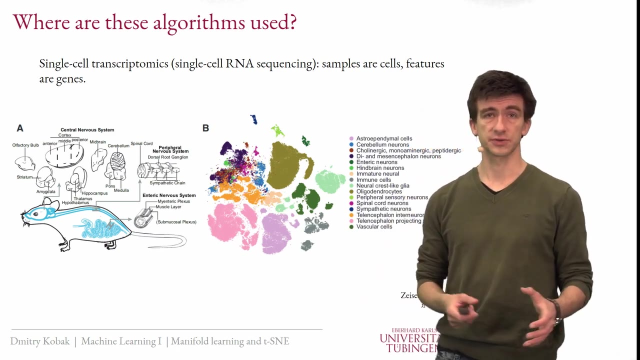 bolts of that. let me just briefly show you where these things are used, why this is of use at all, And actually there are academic fields where these methods have been used a lot and are very popular. So here's one example. it's single cell transcriptomics. 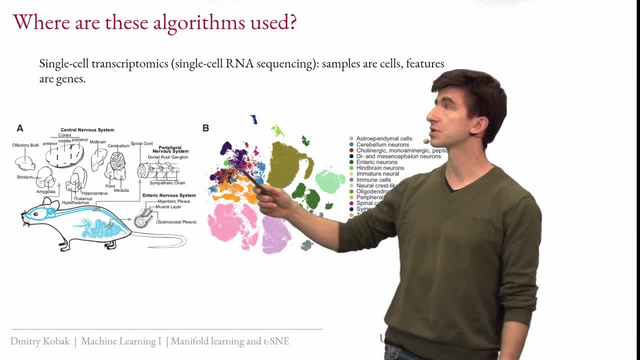 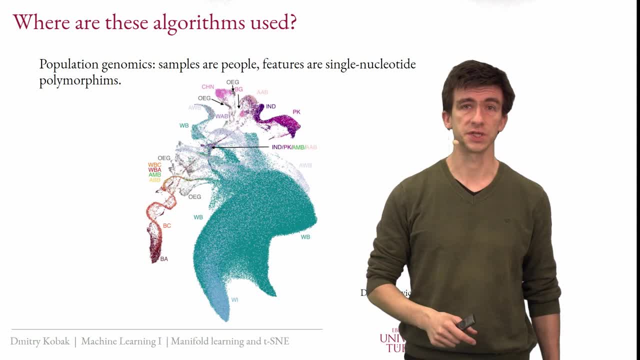 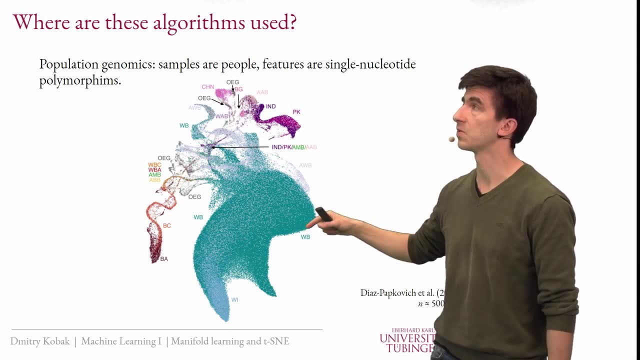 So this is a biologic single cell RNA sequencing. So this is a biologic single cell RNA sequencing. colour, I think, codes here, ethnic origin of the people from the UK, and again this is something like half a million people depicted here, and again one can see a lot of very meaningful. 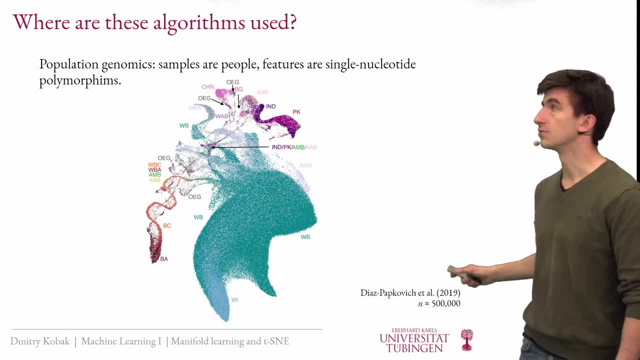 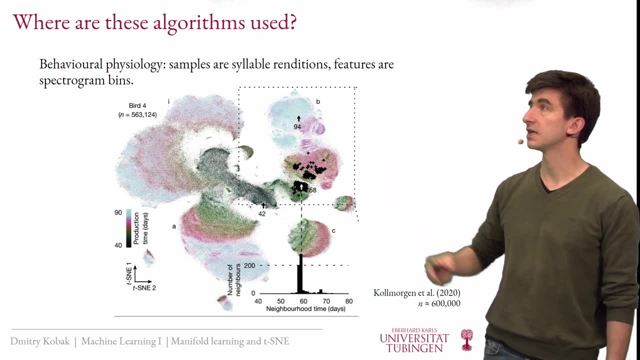 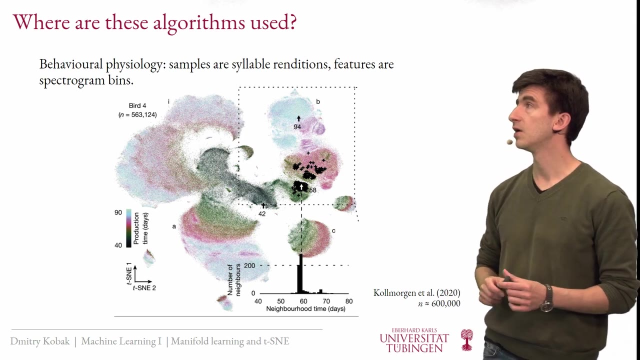 structure appearing on this plot. So here's the reference to look it up, if you want. My third example would be behavioural physiology, where, in this case, each dot is a syllable sung by a songbird, a zebra fish, I think, when they are trying to, when they're learning, 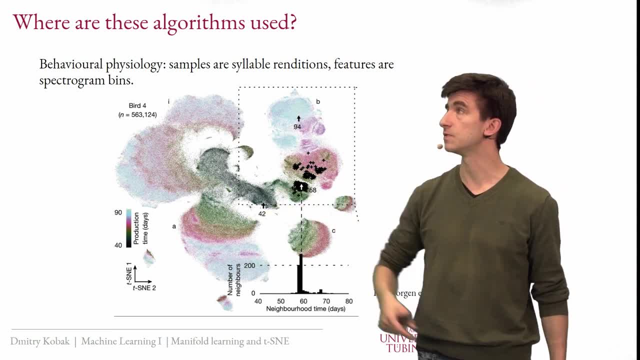 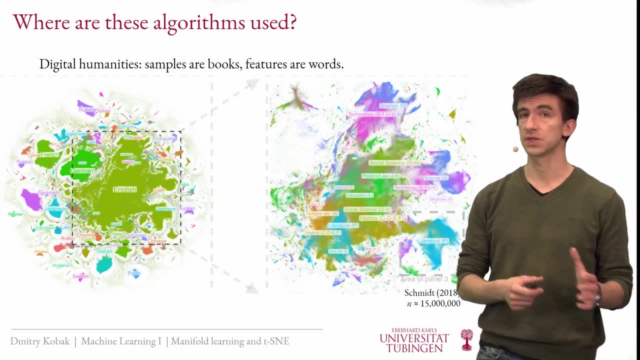 to sing a particular song and one can see how the syllables evolve during training and features are spectral grom bins corresponding to the syllables. And, as a final example, for something non-biological, this is an example taken from this great paper, where there's 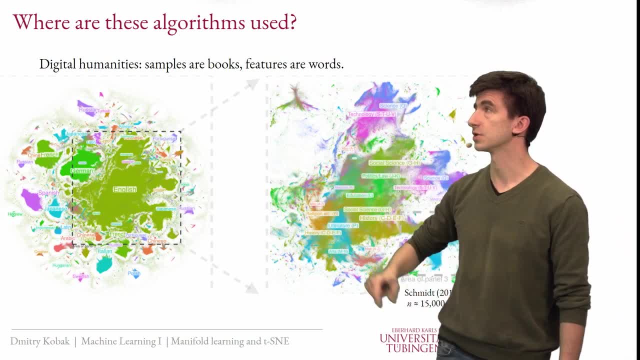 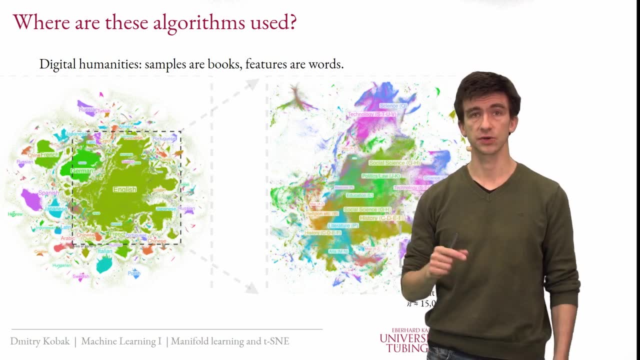 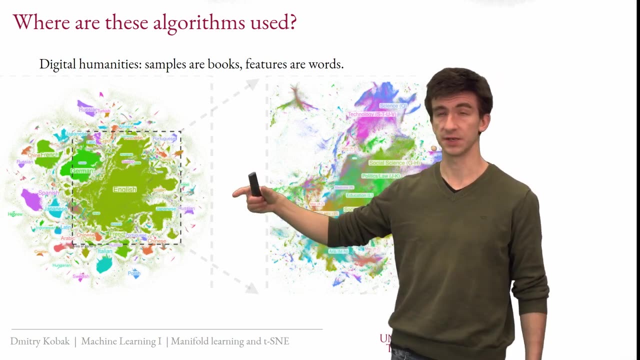 15 million books embedded in these two dimensions. So every point here is a syllable, Every point here is a book from a digital library. Features are words, So there's in fact millions of features here and millions of books. It's a very large and very sparse. 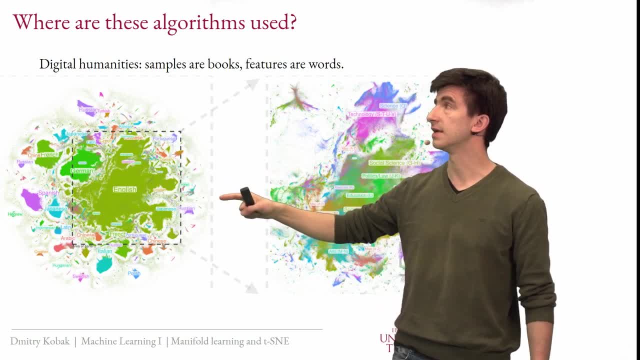 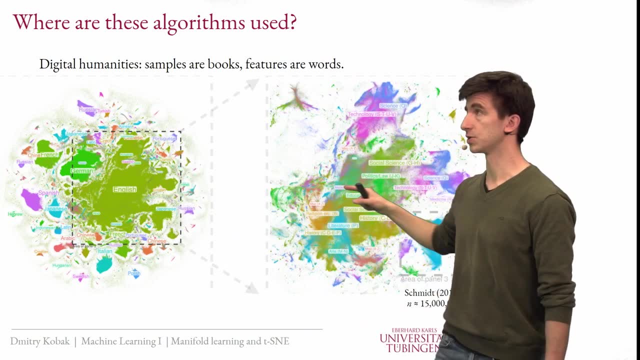 data matrix And you see clearly the books cluster- by the language, of course, because the words are very different. But if you look within the English language books you see that there is a very meaningful structure by the topic and one can zoom in, For example: 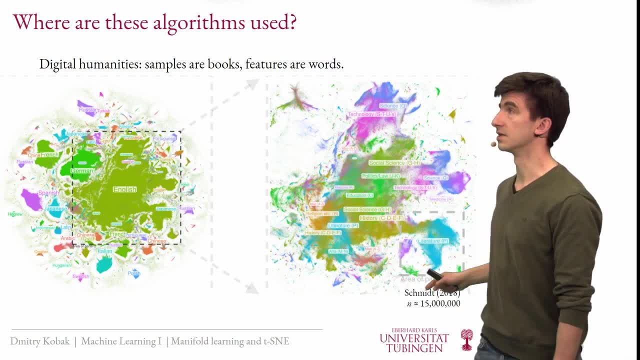 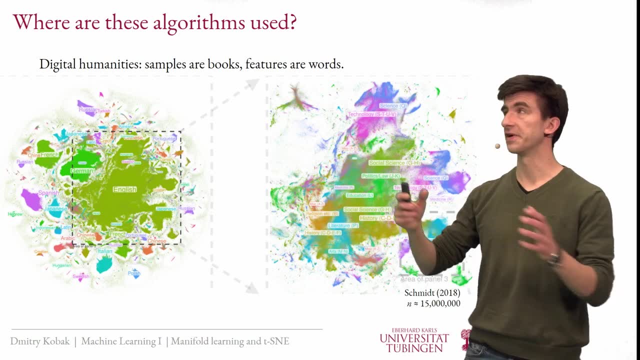 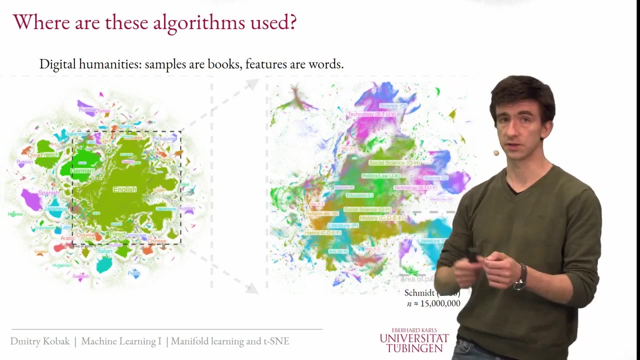 here the literature. The literature is a very important part of the fiction and see further structure down the road. So again, very complicated, very large data set with a lot of complex structure hidden in it, Clearly in the relationship between the books And algorithms like t-sneel. 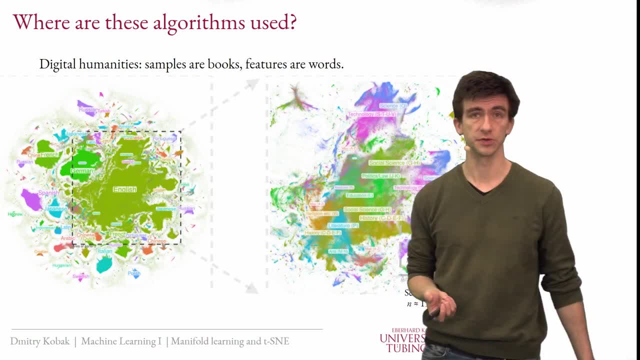 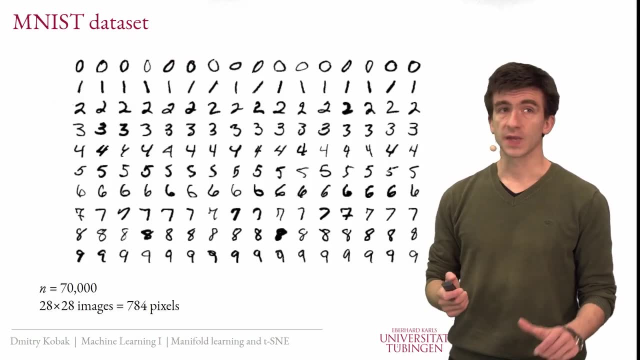 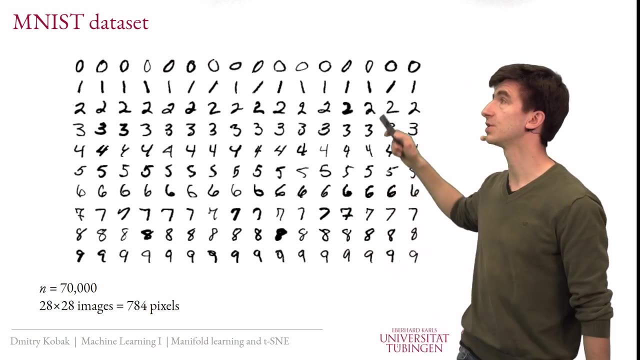 and related ones can make this beautiful but also useful visualization and uncover some data Most of the time. today I'm going to be talking about MNIST data, which is a classic machine learning data set consisting of images, handwritten images, of digits. So there are labels, There's 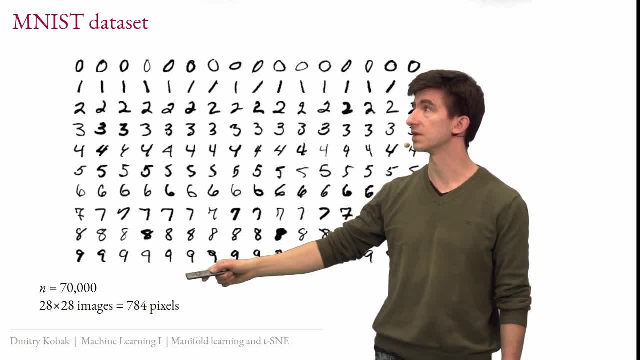 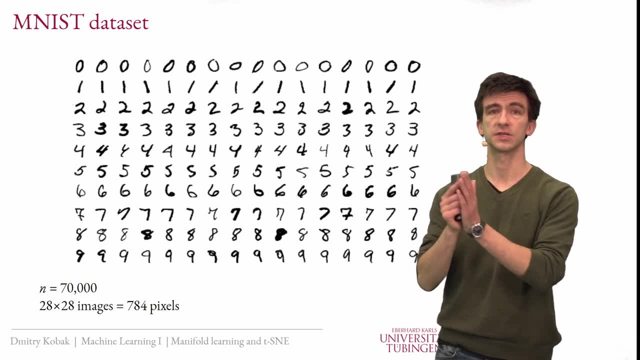 ten different digits possible here. There's 70,000 of them in the entire data. Each image is 28 by 28 pixels, So 784 pixels. So our pixels, the pixels are our features and 70,000 is the samples. 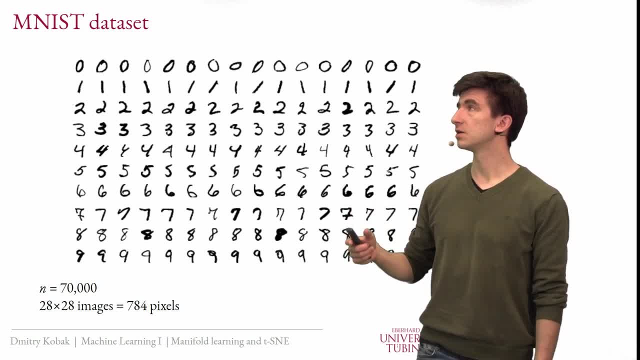 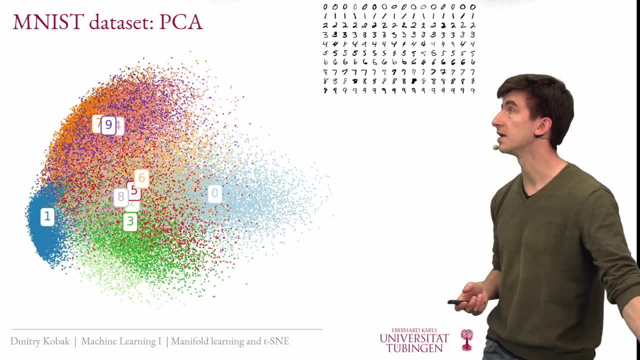 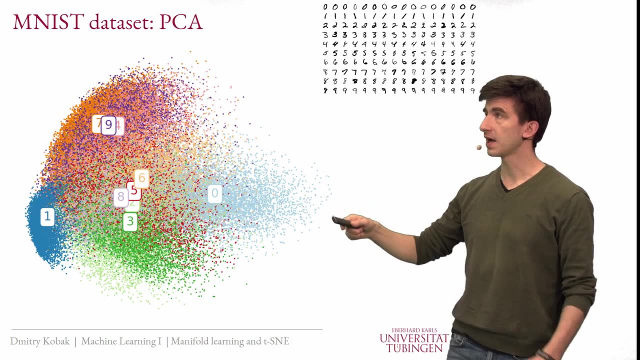 So we want to visualize this in two dimensions. The method that we already discussed is principal component analysis, So I can show you how the PCA of this data looks like. Here it is Right. In fact, quite some interesting structure can be seen here already. So this is for. 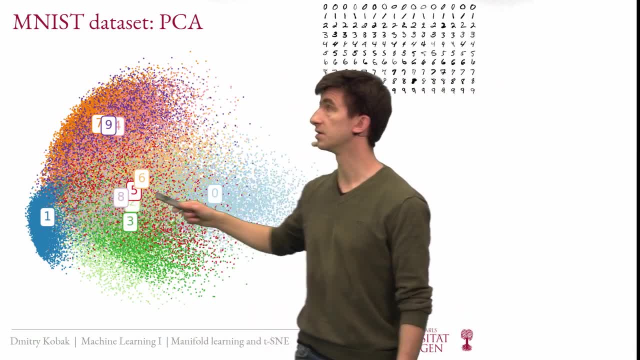 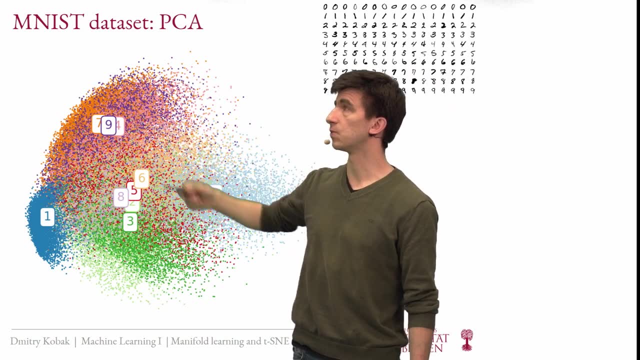 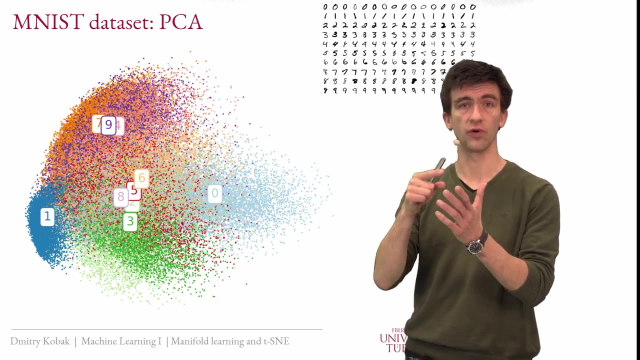 example the digit 1.. It seems to be all grouped out here. The zeros are here on the right. These three digits on top overlap a lot. But if you look close at what digits they are- 7, 9, and 4, and if you think about pixel representation, then actually 7 and 9 and 4. 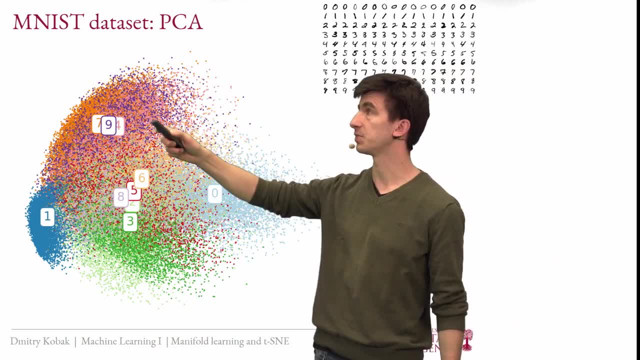 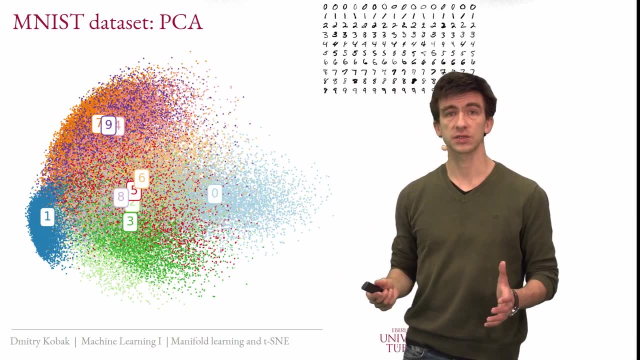 overlap a lot in terms of having the same pixels, So it does make sense that they overlap here. Some of these digits are also similar in terms of how they are written. So we see PCA works. It shows us something that is meaningful, But perhaps one can do better in some sense. 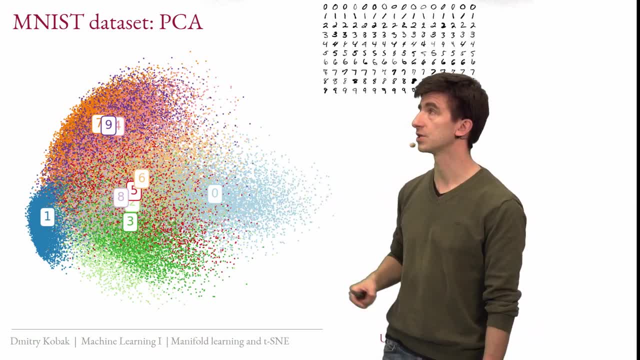 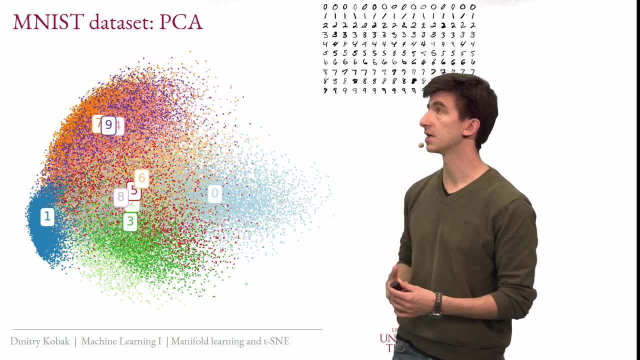 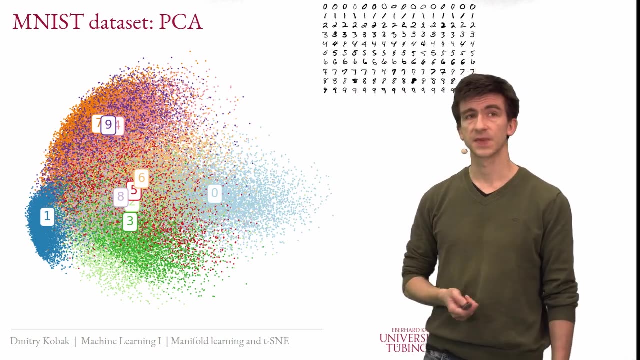 or it would not be possible to look at this and say: ah okay, there are ten different kinds of objects present in this data set. right, It's all completely blurred together, with the exception of maybe this slightly denser cluster of ones on the left. So I'm 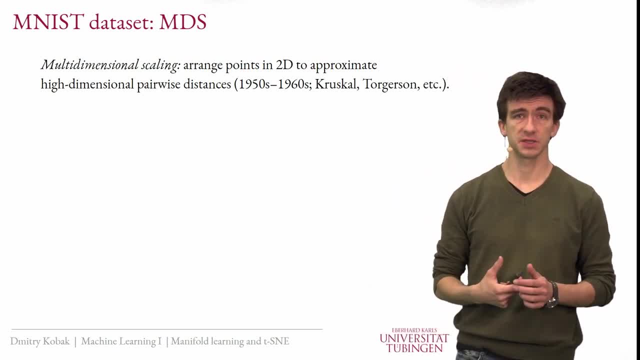 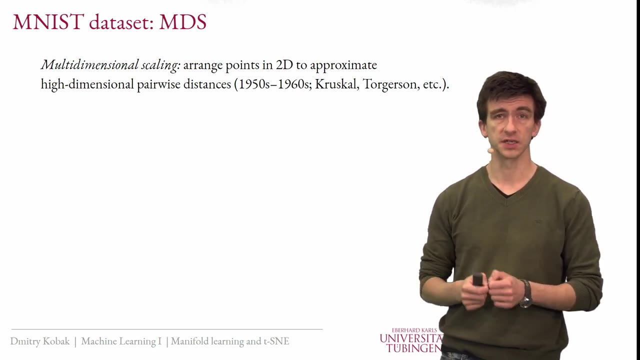 going to start presenting this, what I call nonparametric methods by multidimensional scaling. It's a very old method from the middle 20th century, developed in the 50s and 60s by different people, And the aim of MDS is to arrange points in two dimensions such that pairwise distances. 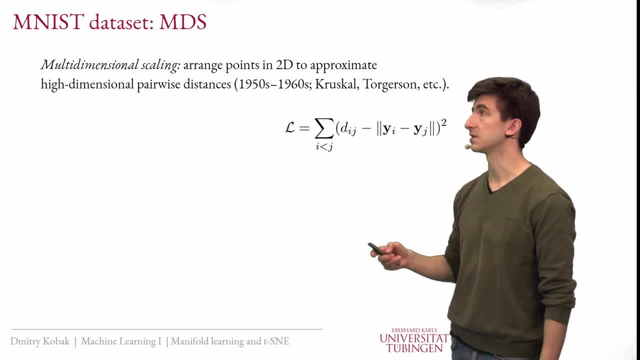 between points are preserved as well as possible. So this makes sense. Here's the loss function of MDS. This seems to make sense. Here's the loss function of the MDS. These are our original pairwise distances. So we compute pairwise distance, Euclidean distance, for example. 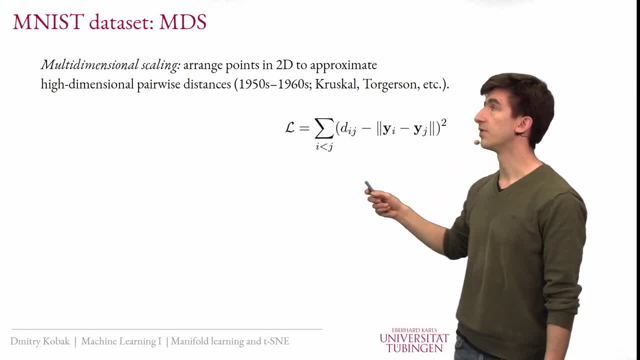 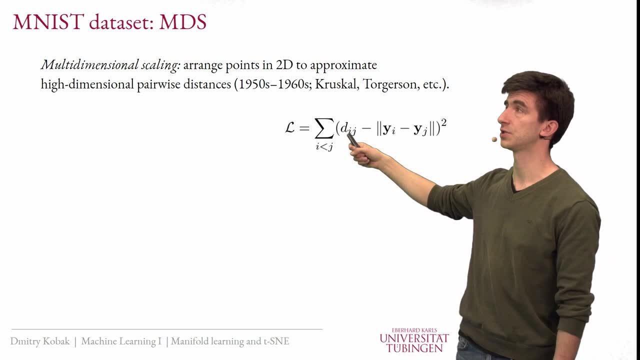 between every MNIST digit. And then we want to arrange points in two dimensions such that Euclidean distances in the embedding over here were as close as possible to original distance, and we just take the mean squared error as our loss. I can show you how the 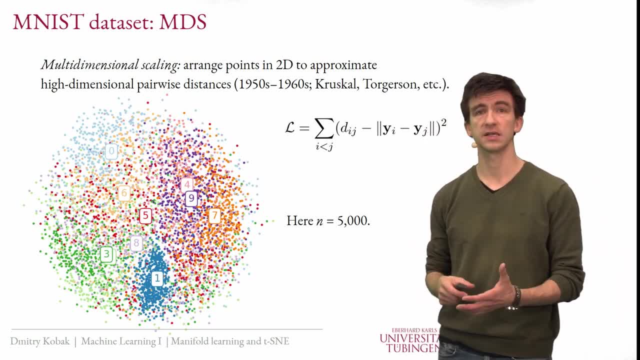 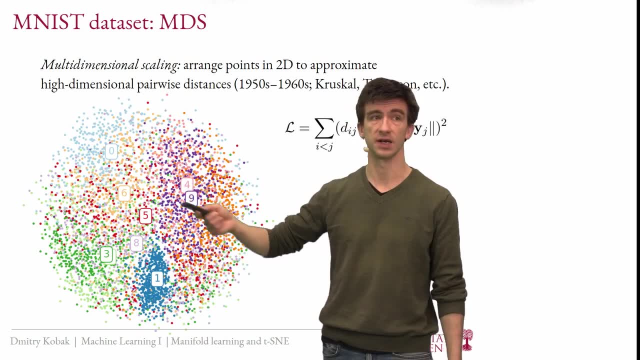 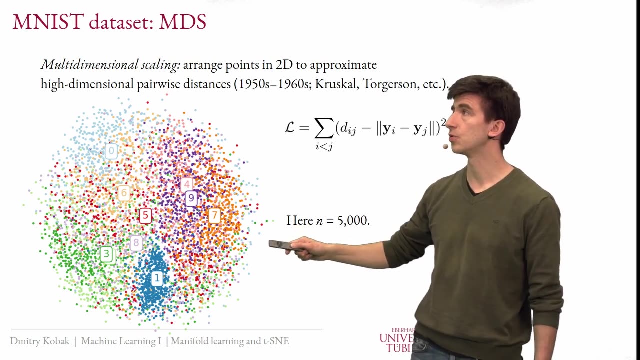 result looks like, and it's not really better than PCA in this case And it's not really impressive. Again, ones are close together here and everything else is basically a mess. One interesting or important point here is that I'm only showing 5,000 points here, Whereas 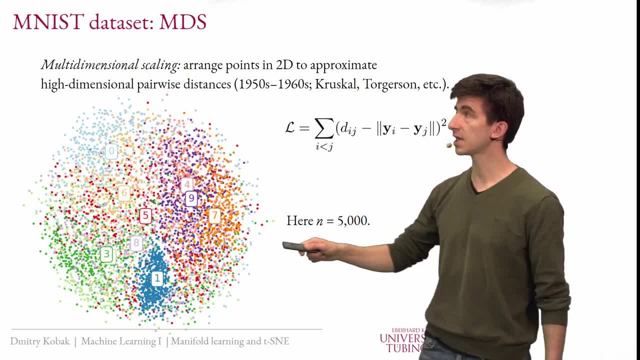 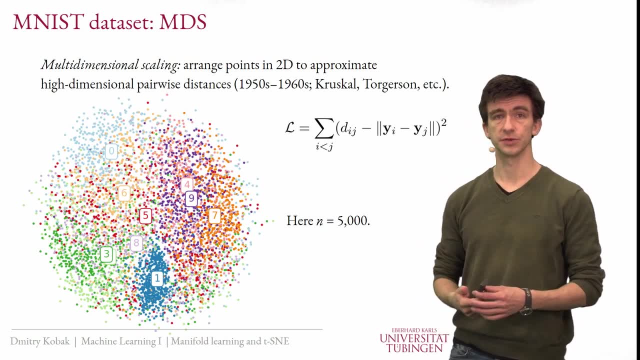 for PCA. on the previous slide that was all 70,000.. And the reason I'm only showing 5,000 is that it is very challenging to produce a multidimensional scaling embedding of a larger sample size, Because to do that we need to compute pairwise distances between: 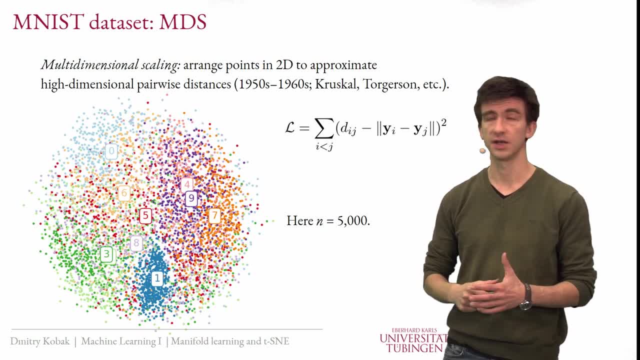 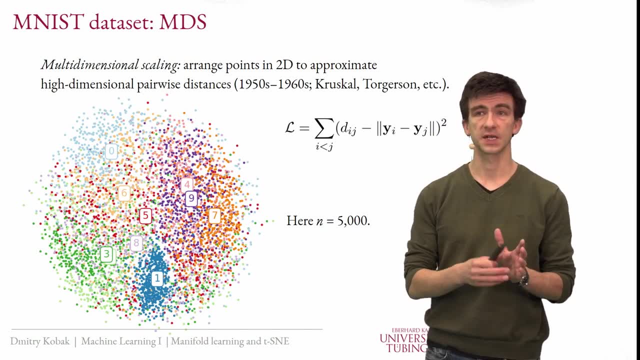 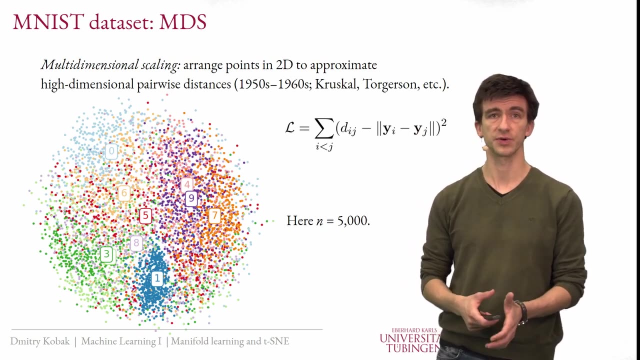 all pairs of points. So this is quadratic complexity in terms of memory and run time as well. So if you take 70,000 images, you need to compute distances 70,000 times 70,000. That's the size of the distance matrix. And even to compute and store in memory this distance. 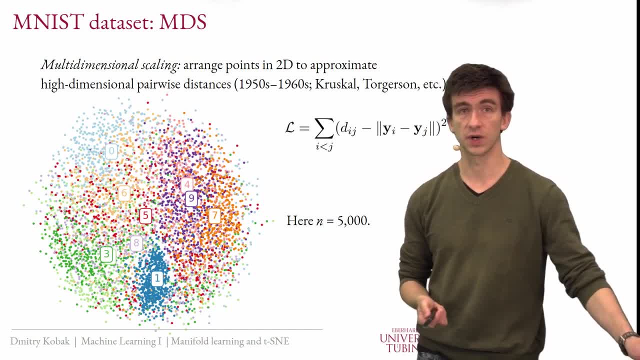 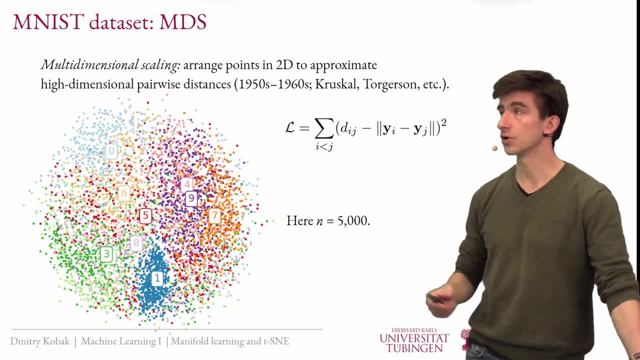 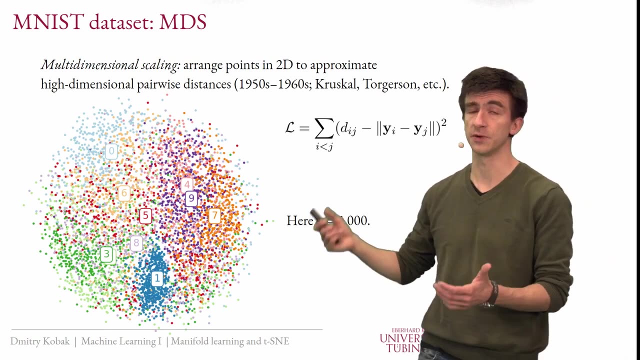 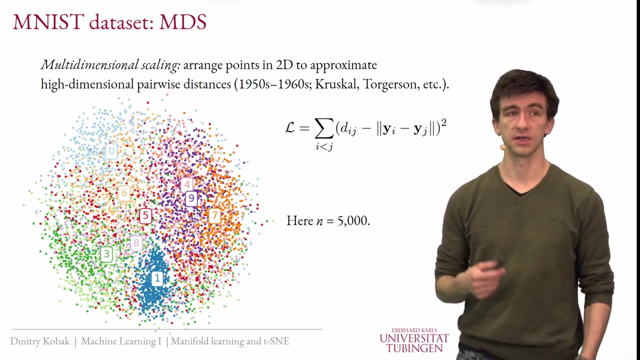 matrix is already prohibitive or at least requires a lot of memory. And then that's before you even started optimization. So it's really hard to scale MDS. Nobody really uses MDS for larger data sets. Probably if we could compute it on all 70,000 MDS images we would see something similar. 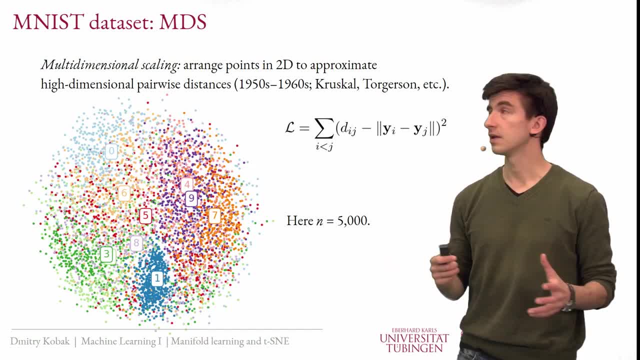 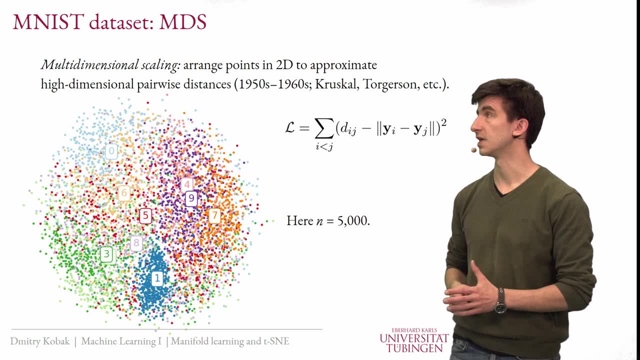 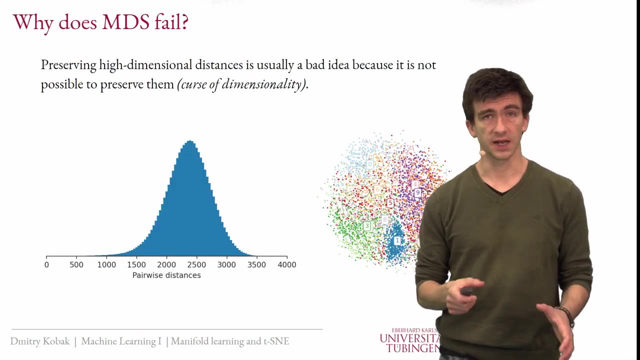 At least that is my guess. So why does MDS not show us structure that I will later show you is actually present in this data. Why does MDS fail in some sense, even though the loss function seems to be pretty reasonable? And it has an interesting and important reason. 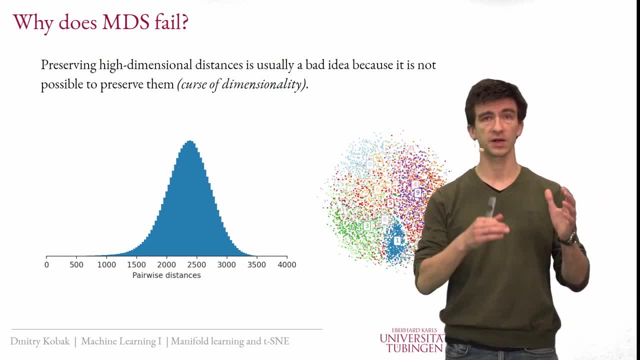 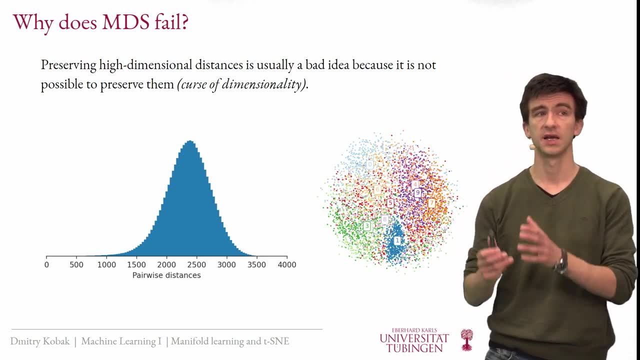 why MDS fails in this case, That preserving high-dimensional distances in the low-dimensional embedding is just a bad idea. It sounds as a good idea, but it is a bad idea in fact, because it is not possible to preserve the distances. There's no way to arrange points in 2D to preserve. 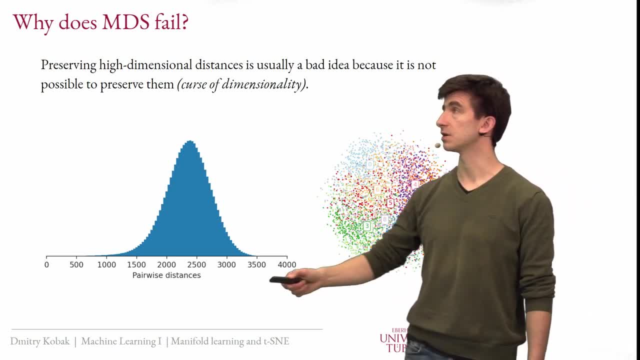 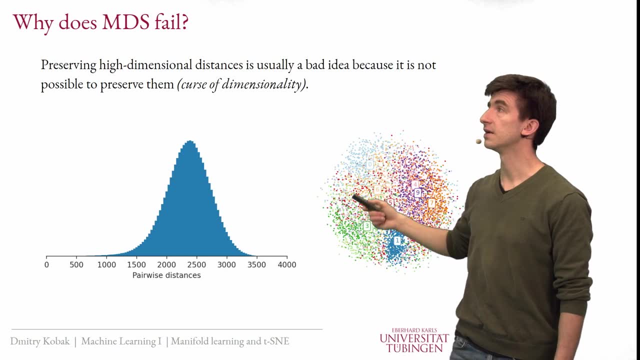 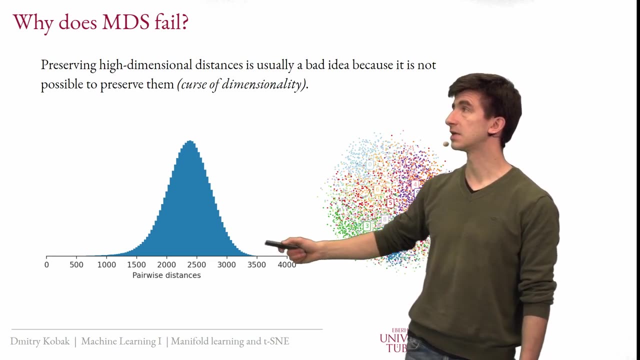 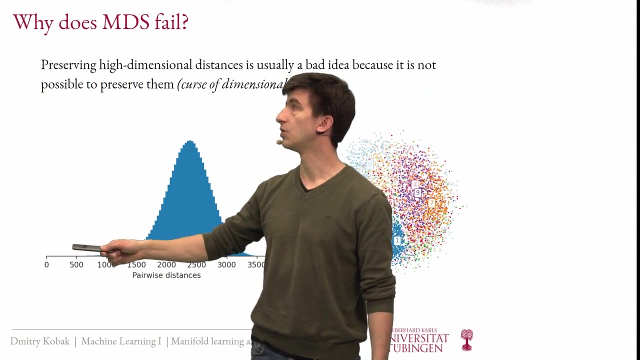 the distances. And let me illustrate here by computing pairwise distances and plotting a histogram over pairwise distances in the high-dimensional space for these 5,000 points subset of the MDS data. It doesn't look striking. probably Some distribution, but note that zero is over here. 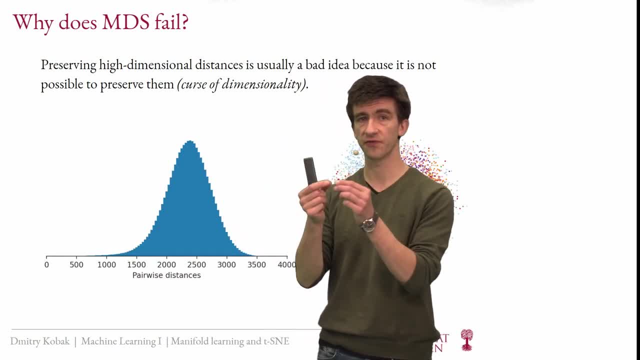 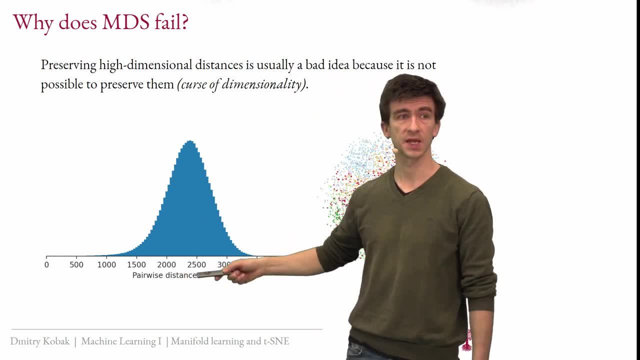 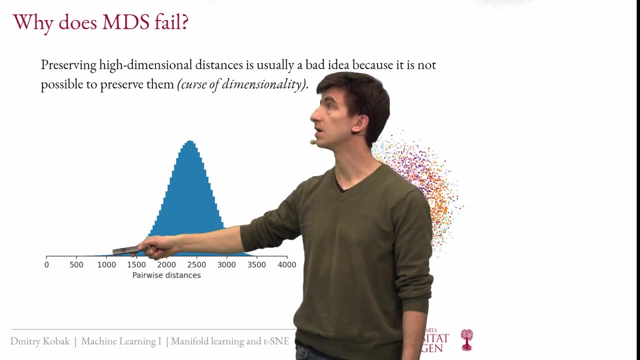 There are small distances. There are no two digits that are very, very the distance is very small between them. in the high-dimensional Most of the distances are around 3,000. in whatever units this is but the smallest over here there may be- maybe go down to 1,000. 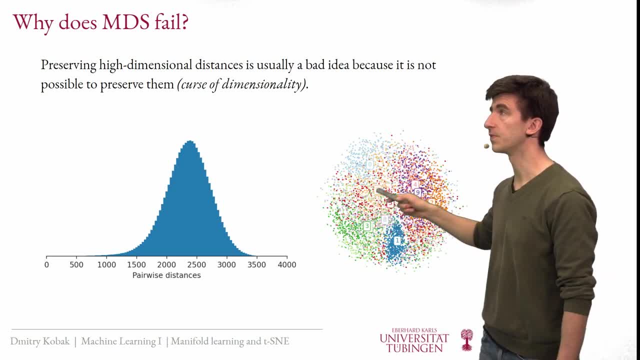 can't put the points in 2D, so that this is true. If you want to have some large distances here between this and this, you can do that, but there will be some points that are close together that will have distance of around zero. It's just not possible to put points. 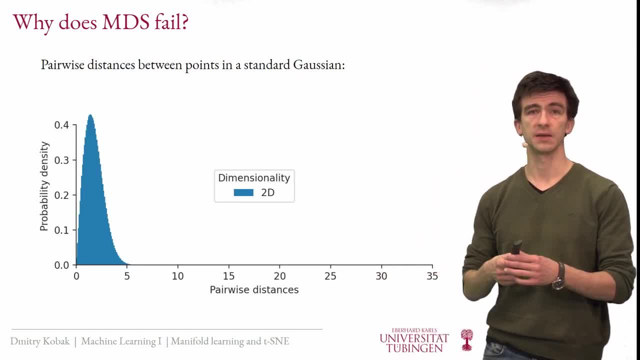 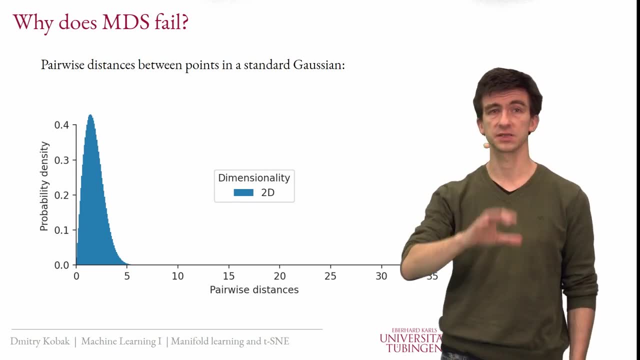 otherwise. Let me illustrate this in a slightly different way. I'm just going to generate a random Gaussian data in two dimensions, so random, uncorrelated Gaussian with unit variance, and compute pairwise distances between all points in this Gaussian And that is the distribution of distances, pairwise distances that one gets in two dimensions And this 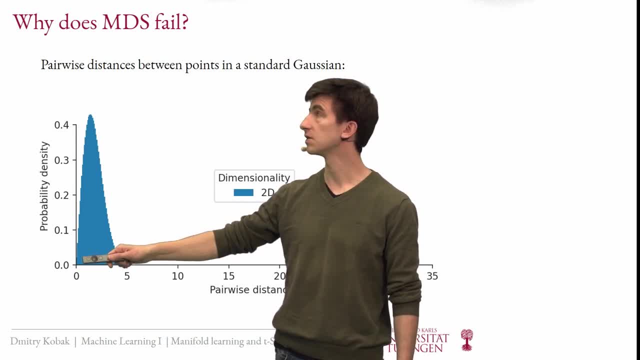 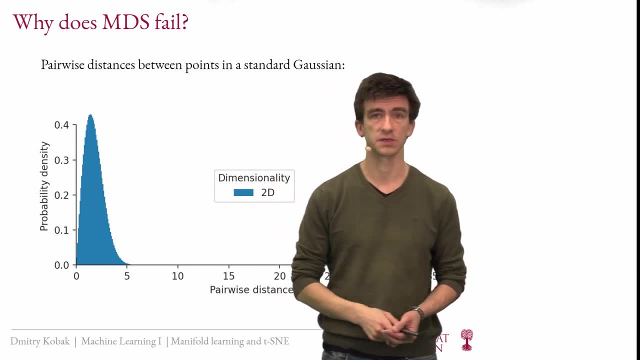 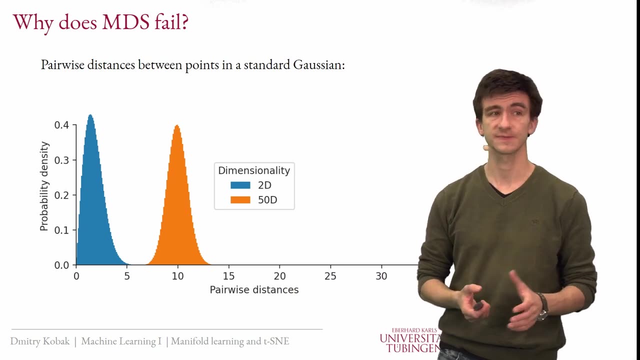 does make sense. So there are some distances that are very small, around zero, or there's some average distance that one gets, and it goes maybe to five for the points on the different sides of this 2D Gaussian. And let me now show you what happens in ten dimensions Again. 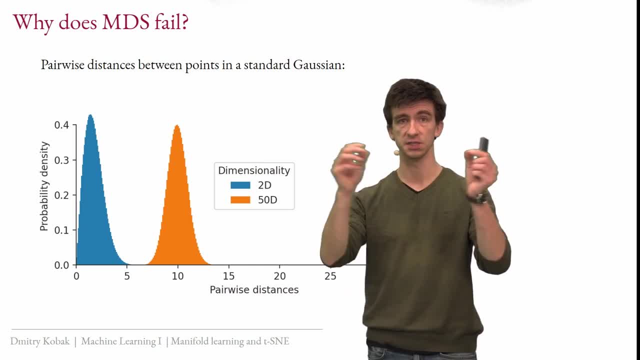 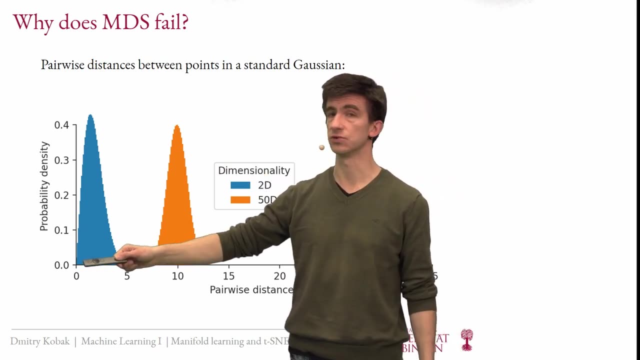 there is some average distance. The distances are larger. Just think about computing the distance now between ten dimensions. No random vectors. But the key point, and the one that is very easy to understand actually, if you think about how this distance is computed, is that there are no points that have very 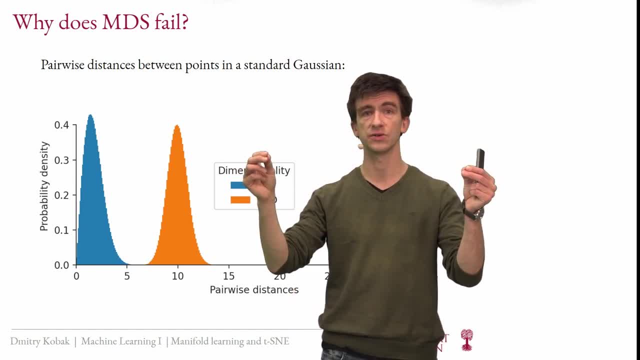 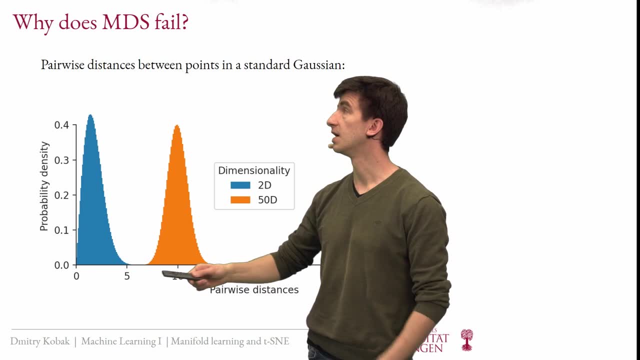 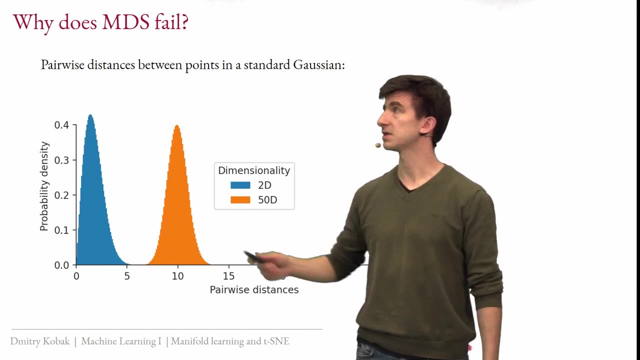 small distances. It would be very unlikely to generate a string of ten random Gaussian numbers twice and then have very small distance between them. That just doesn't happen. So all these distances live here around centred at ten and this thing looks basically a shift. 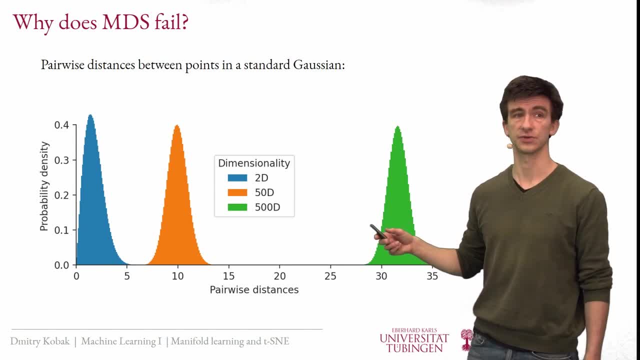 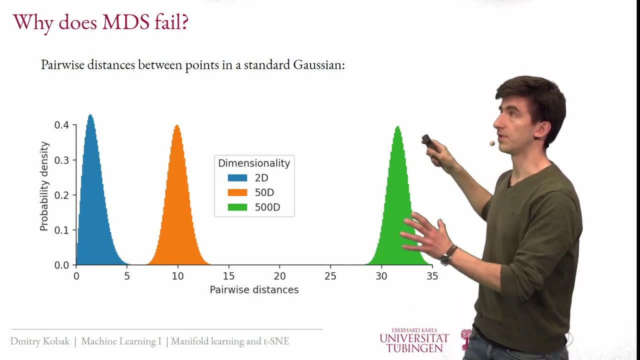 to the right, and if I scale the dimensionality up to 500, then here we are. Now, if this were the pairwise distances in the original data and you want to arrange them in 2D somehow to preserve these distances, this is just not possible. You're trying to fit something. 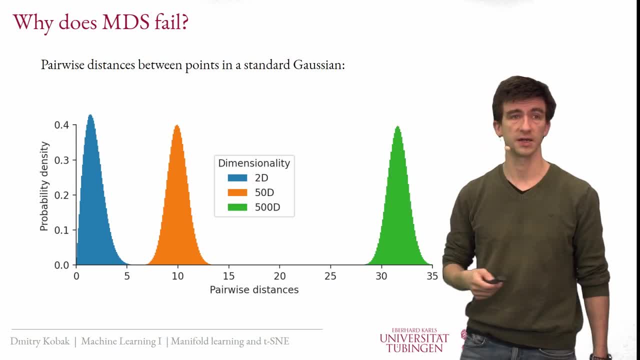 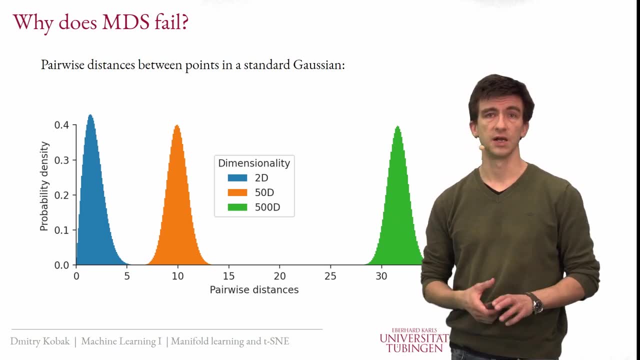 that will look like a blue distribution to something that looks like a green distribution. This, of course, fails, and that's why MDS often or usually fails, and that's why MDS often, or usually, typically does not produce an interesting or meaningful embedding. So the 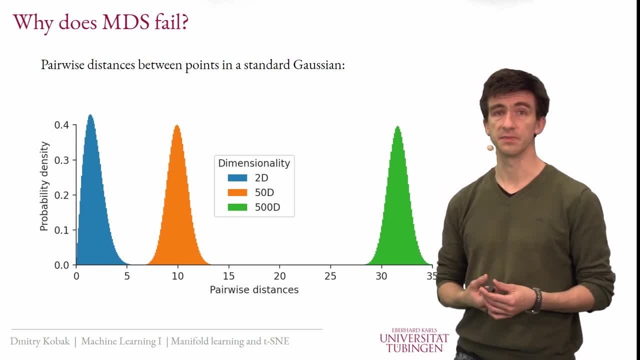 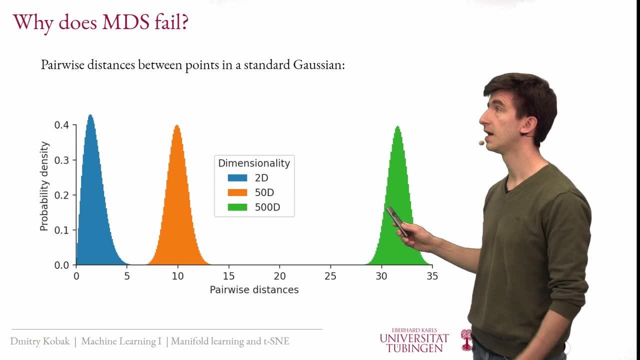 key idea of t-SNE and methods that we can call neighbour embeddings is that we just give up on that entirely. We're not trying to preserve the distances anymore. That's not possible, so let's forget about it. We will try. we will aim to preserve the rank of the distance. 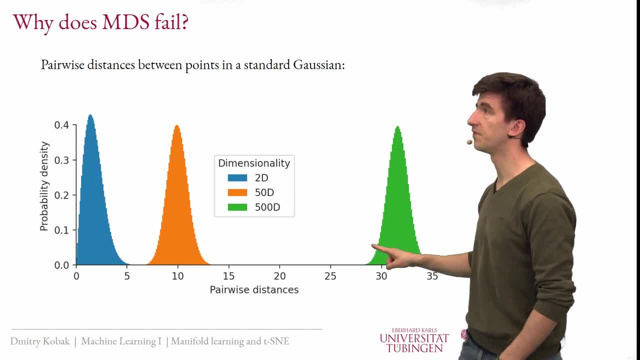 or even more specifically, we're going to aim to preserve this very left part. We're going to find neighbours in the high dimensional data. so neighbours, these are the pairs of points that have small distance, so they live here on the left side of this green distribution. 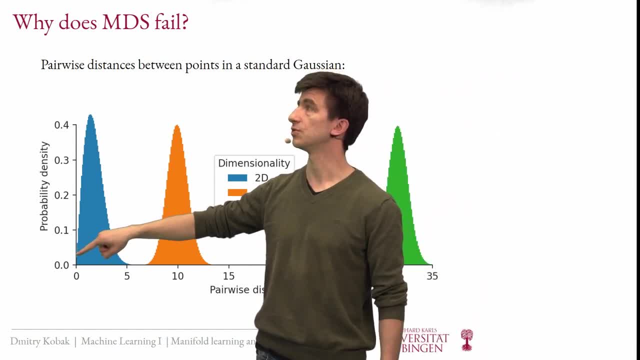 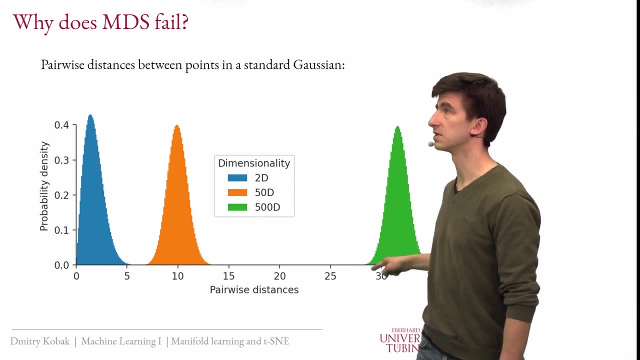 and those we want to make sure that are mapped here to this part. so they are neighbours in 2D as well and the rest should be the rest right. So we want to make sure that this left part of the distribution is mapped to the left part of this distribution and 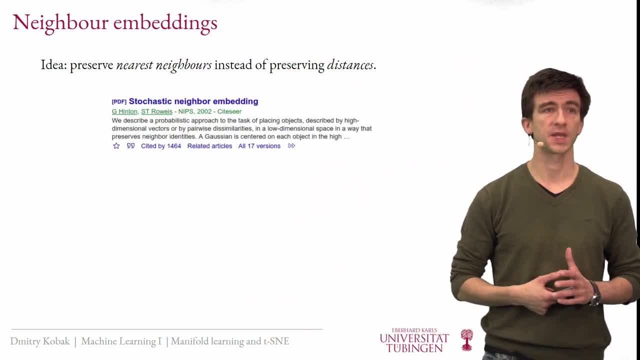 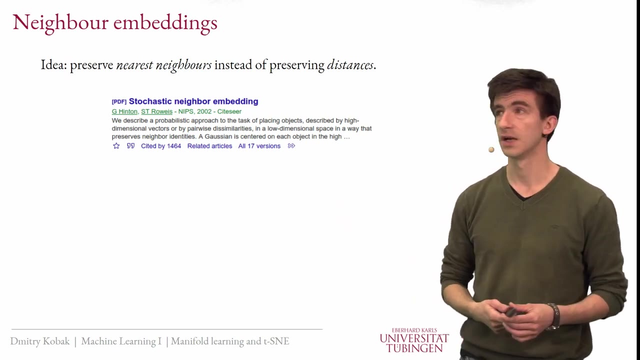 that's what all these methods are doing. So that's the idea of what I'm calling neighbour embeddings, Following this paper, which was basically a landmark paper that suggested this idea for the first time and really was a game changer, I think. so they suggested something that they called stochastic neighbour. 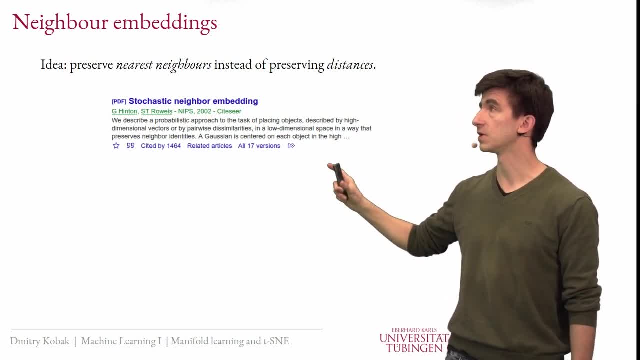 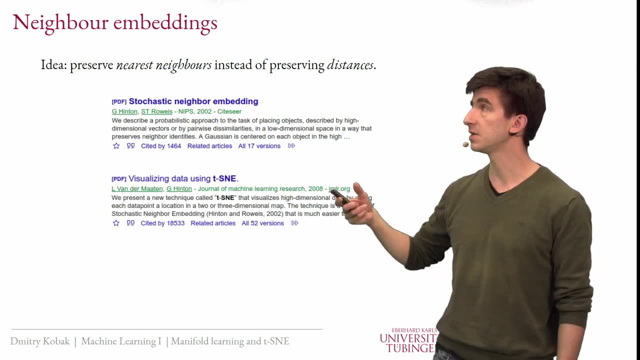 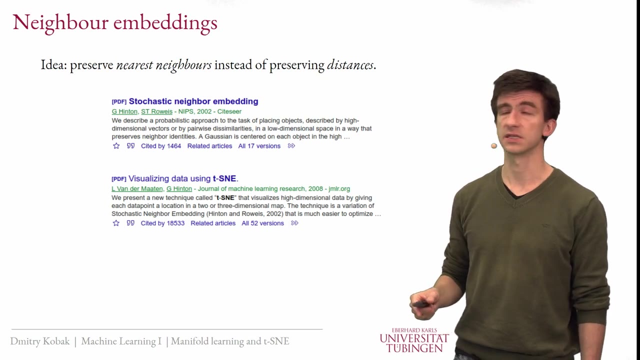 embeddings or S and E, so it's very, very influential, important paper, beautiful paper, In fact. what is much more often cited, though, nowadays is the t-SNE paper, which is the paper, also co-authored by Geoffrey Hinton, that came out later, a few years later, and 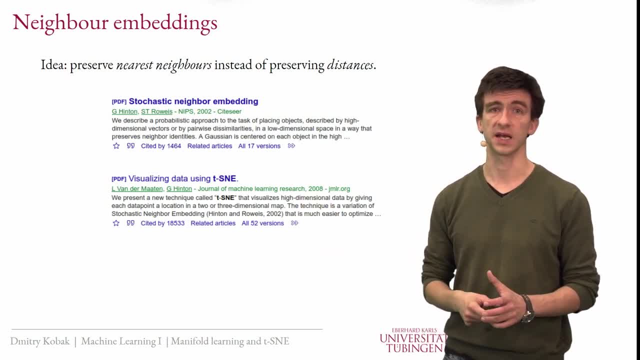 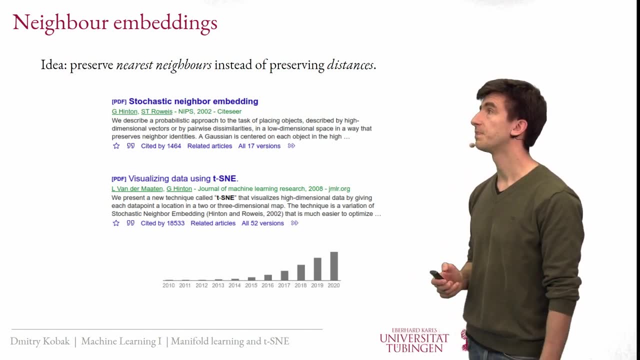 suggested, basically one relatively minor modification of an S and E idea- we'll discuss what it is a bit later- and that's the t-SNE method and you can see that it's cited a lot and actually interestingly, if you look at the citation count, it just keeps increasing. 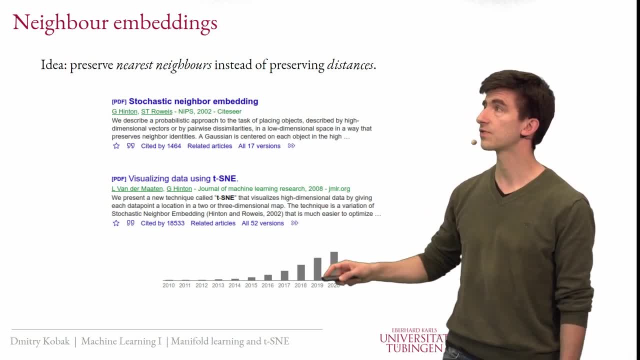 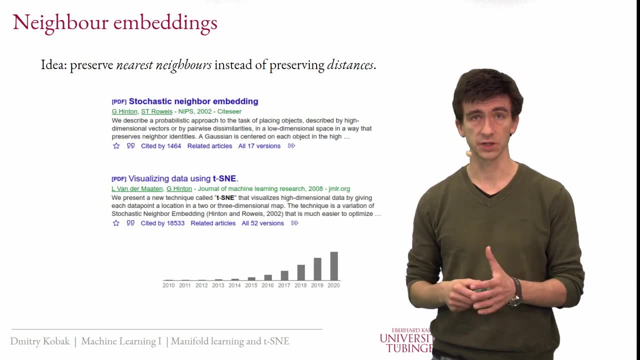 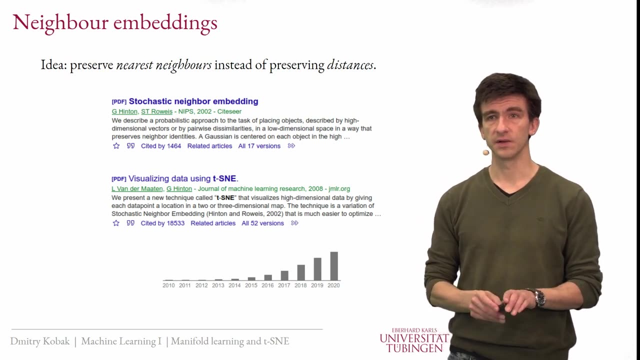 so more than half of these 20,000 citations came from the last two years, and the reason, I think, why this is happening is that more and more people are starting to think that more and more fields, for example in biology, started to generate data that are very, very. 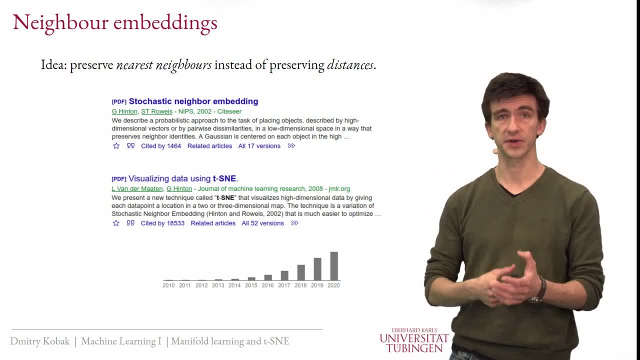 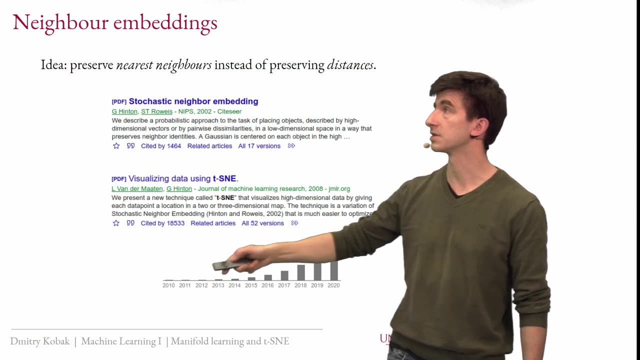 good for very amenable to this kind of algorithm. so very rich data and very large data and people in these fields just like using this algorithm, these kind of algorithms, and that's why it just keeps gaining popularity more and more. And back then 10 years ago when it came out, 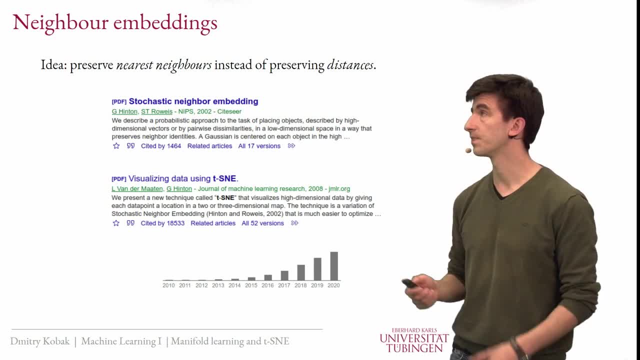 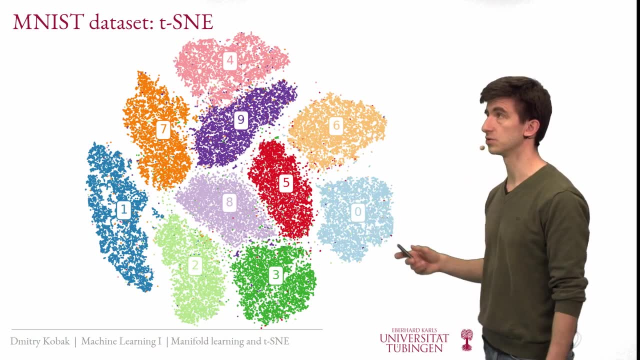 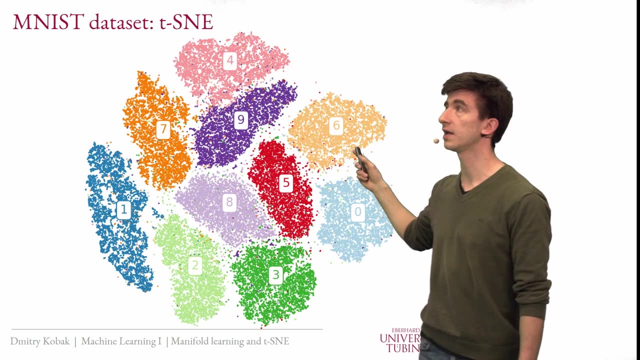 It didn't seem as useful at the time. All right, So let me just show immediately how the t-SNE of MNIST looks like. So this is the default t-SNE picture of the MNIST, and it's beautiful. You see that every digit is actually its own island, right? 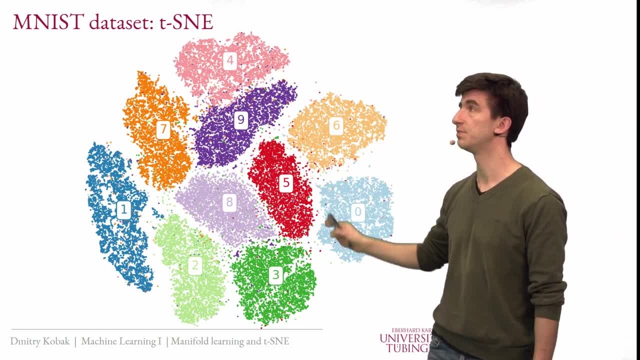 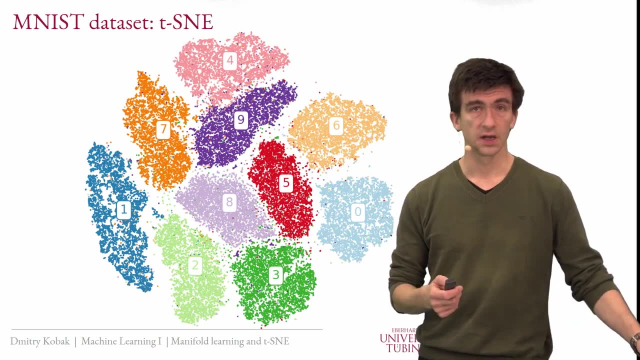 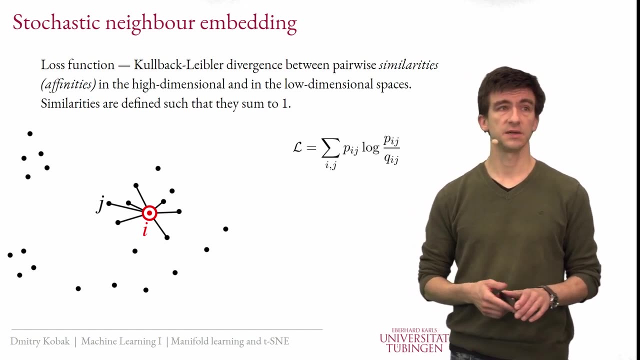 There's almost no overlap between different digits. There's white space in between digits, so we see that there are 10 clusters in the data. Yeah, Just great. Hi, How does it work? So the idea of the Stochastic Neighbor Embedding SNE and t-SNE- is that the so we want to? 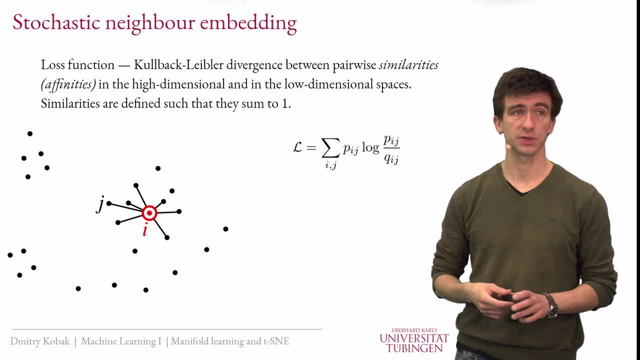 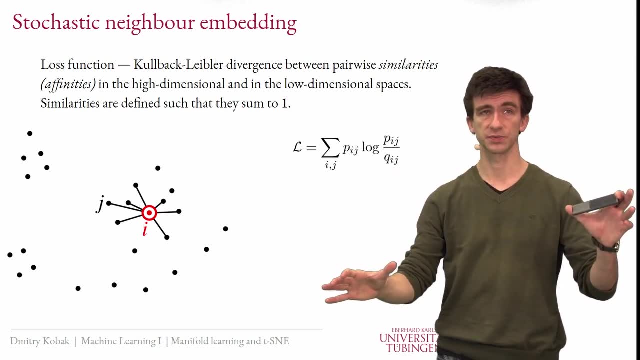 preserve neighbors right. And the loss function is the so-called Kallblik-Leibler divergence between something that we will call pairwise similarities or affinities in the high dimensional and low dimensional space. So similarity is like the opposite of distance. 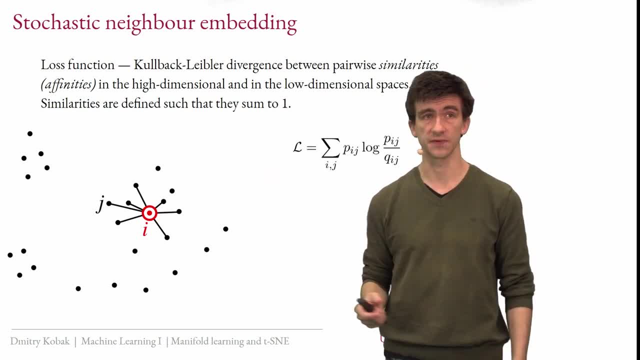 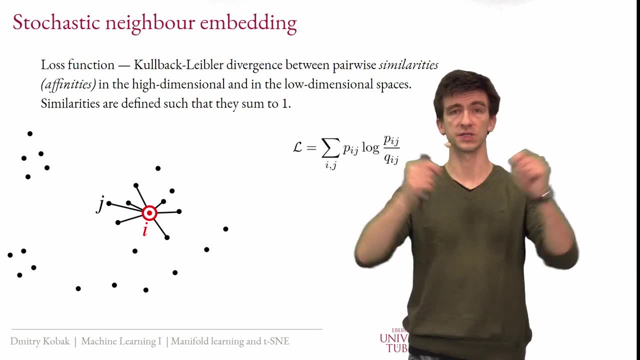 Similarity is large when the distance is small And the affinity the same. for the affinity, We'll say that two points that are very close to each other, they have small distance, they have large affinity. The points that are far away, they will have zero or near zero affinity or similarity. 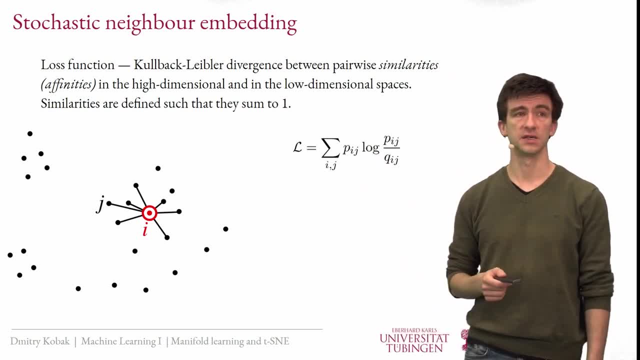 So we will define these affinities between all pairs and we will make sure that they sum to one, okay, High dimensional similarities will be called P's and low dimensional similarities will be called Q's, And once it's done, the loss function is this thing here: 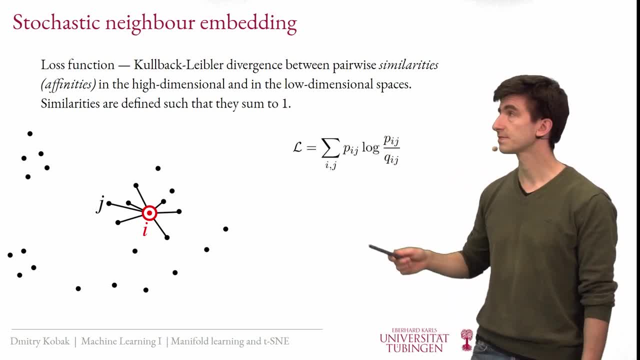 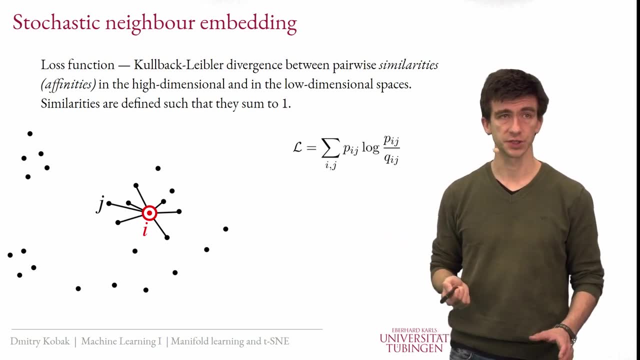 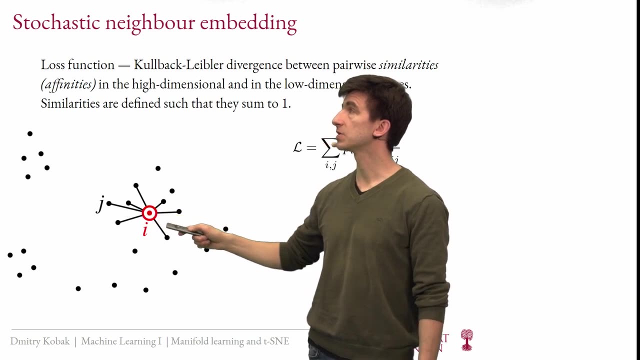 Here, which is known as the KL divergence. So you can see that if all P's are equal to all Q's, then this is zero. So that's what the algorithm tries to achieve. Yes, on this illustration, right? so I found some neighbors of this point. I here and some. 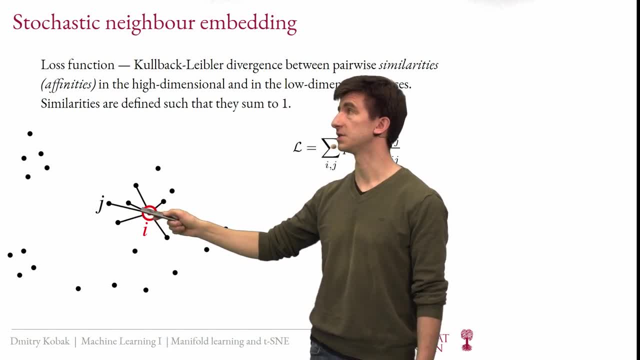 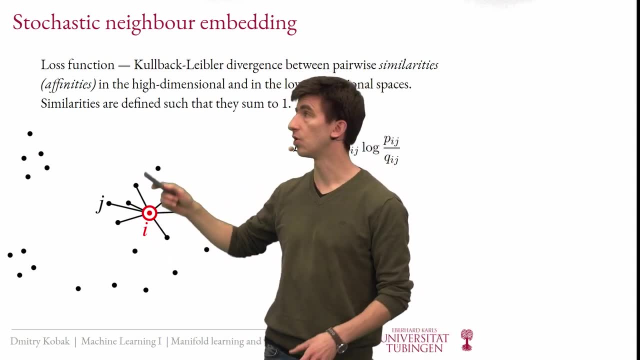 close neighbors. So these will be pairs that have high affinity, And the affinity of this point I to something over here will be either will be very small, It will be near zero, or we can even set it to exactly zero, to simplify things. 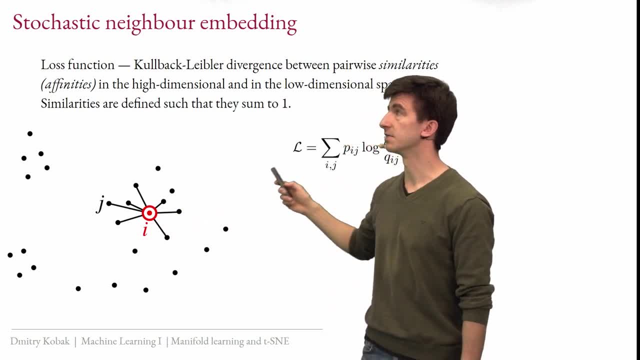 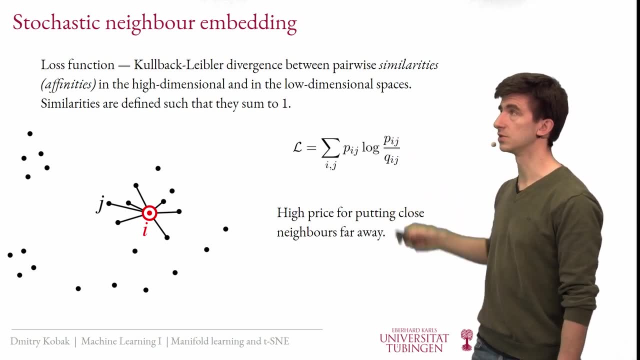 So only these things have nonzero, or at least substantially nonzero, P values. And if we look at this loss, so it's not symmetric here P and Q do not enter symmetrically, But we immediately see that we will pay high price in terms of this loss function if we 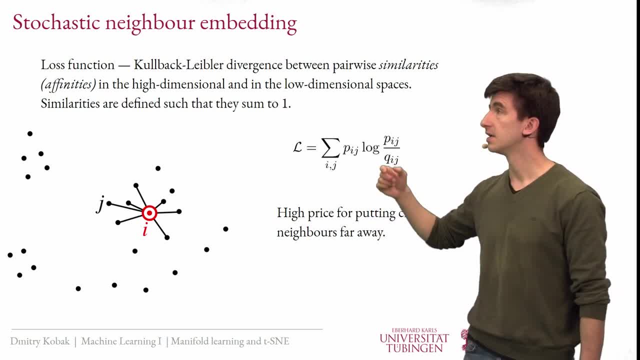 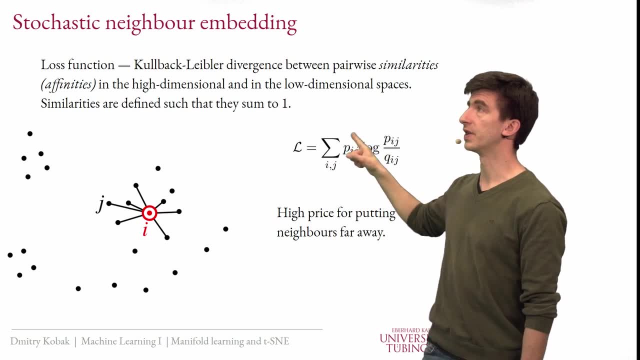 take two close neighbors in the high dimensional space and put them far away. So two close neighbors, some of these pairs, And then we have the loss function. They will have a large P value, right. So this is this logarithm term will enter with this large weight in the loss function. 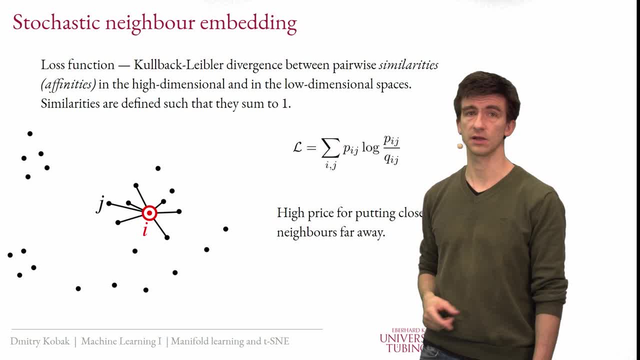 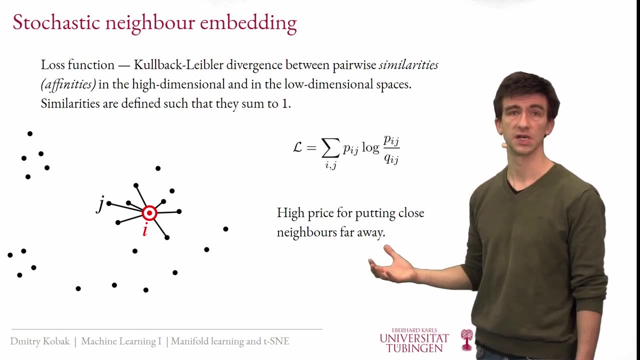 And if Q is small, then that's the price you're paying. What happens with the points that are far away to begin with? Well, they don't even enter explicitly this function right, because P term for them is nearly zero. So you pay high price for putting close neighbors far away. 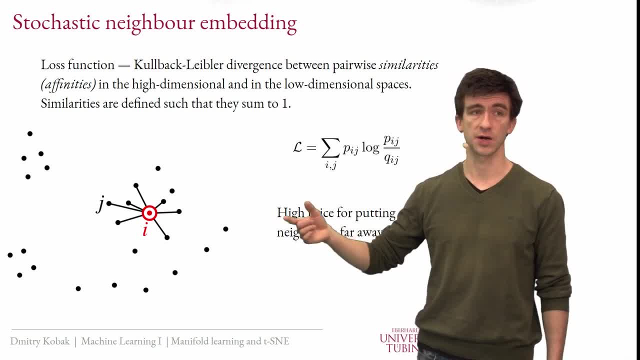 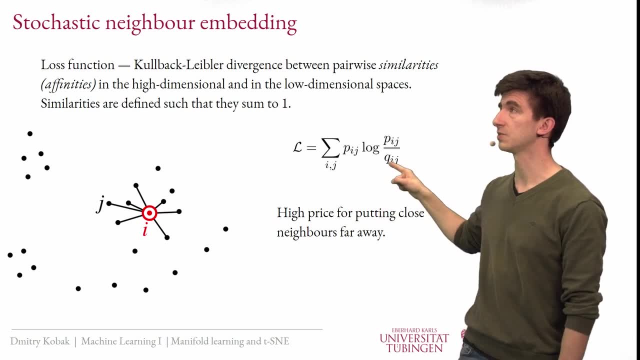 So it's not correct to say that you don't pay any price- the other way around- for putting points that were far away close together. And how to see it here is that Q is normalized to sum to one, as I mentioned. So if you take points that were far away and put them close together, they will get a high. 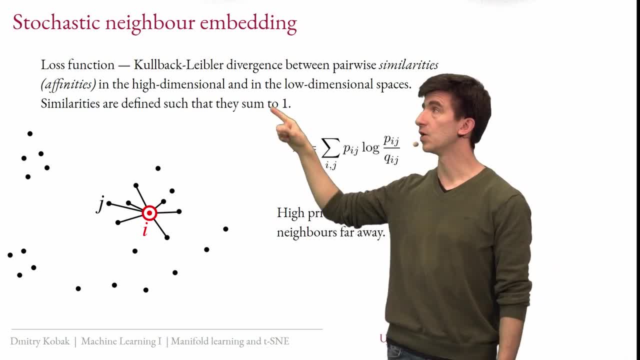 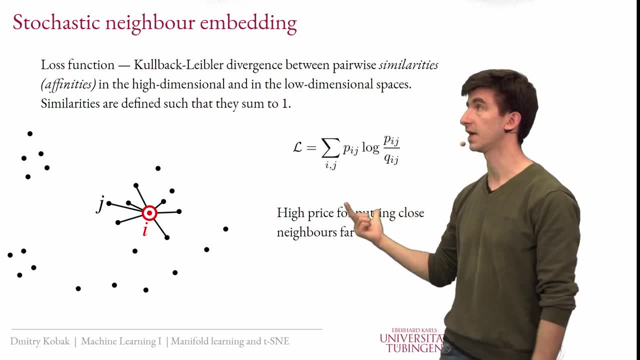 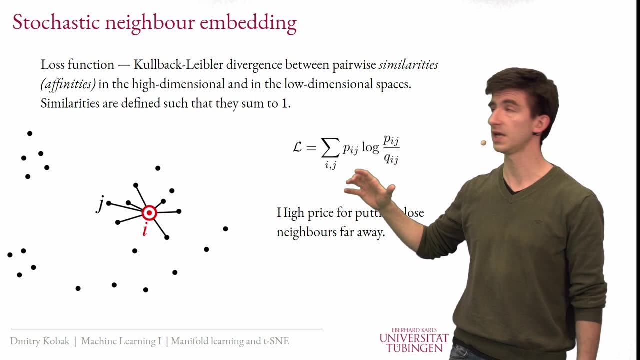 Q value. So you will spend some of this Q weight that you have because it has to sum to one on this modeling the useless pair that doesn't enter this loss function. Okay, So normalization of Qs is actually the part- as we will also see later- is the part that 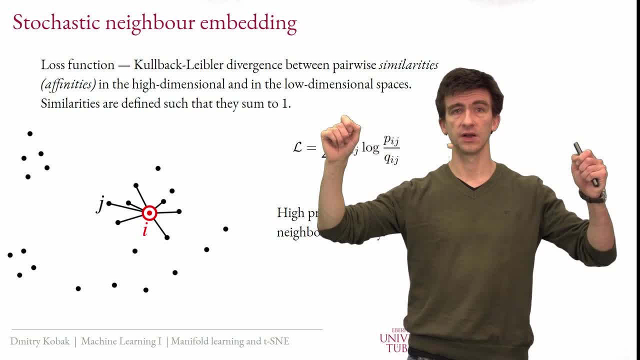 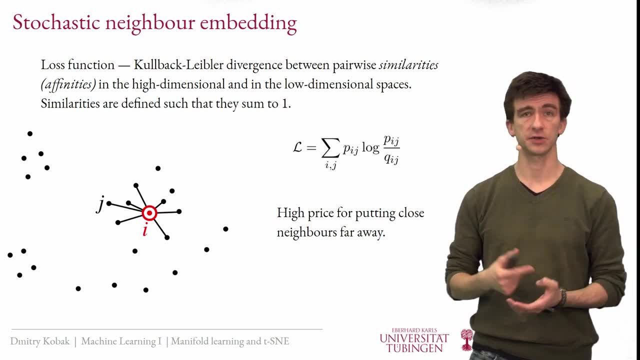 makes t-SNE want to keep far away points, far away. Okay, So we have the loss. What I need to tell you is how to define P and how to define Q, And then I need to tell you how to minimize this thing. 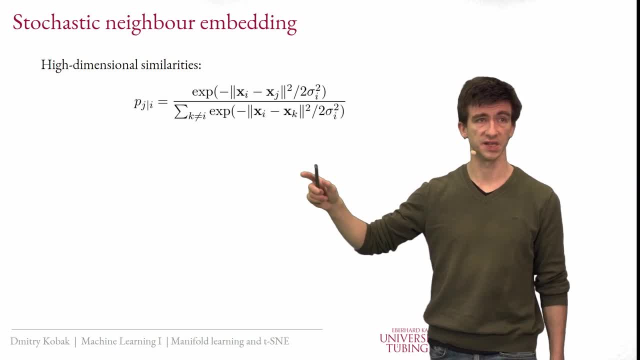 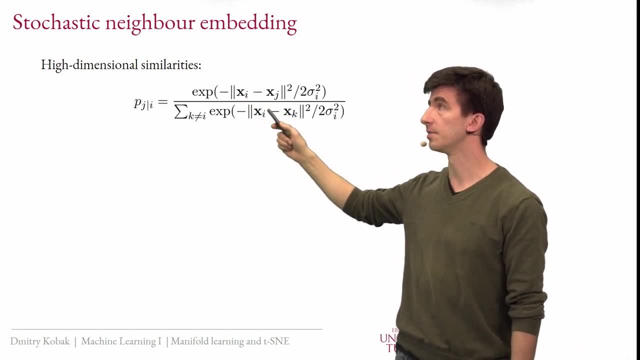 So let's go over it. We'll start with high dimensional similarities, the P values. and what t-SNE does is that it essentially just computes. It computes the Gaussian kernel. here It takes the distance in the high dimensional space. In this case it's Euclidean distance, but it could be any other distance in fact. 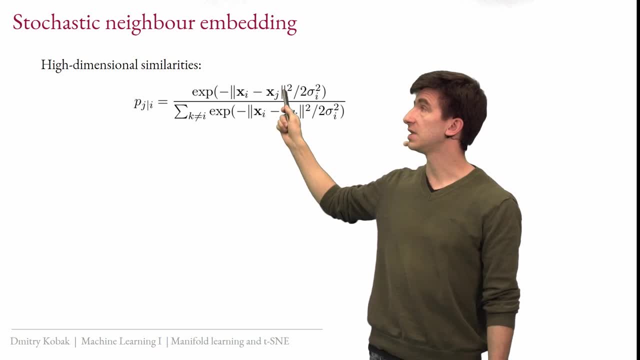 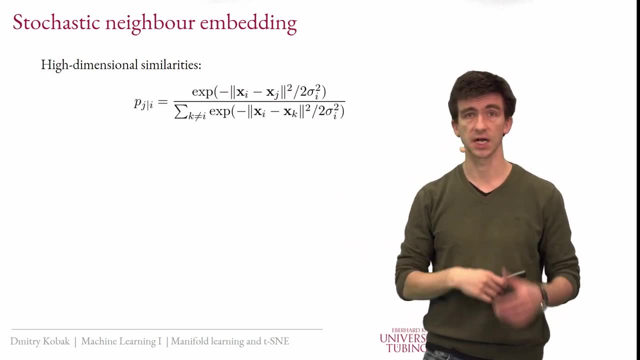 But we will just talk about Euclidean distance today. So this is the distance between high dimensional points and then its exponent with a minus sign of that. So a Gaussian kernel: The larger the distance, the smaller the Pij. So this is: 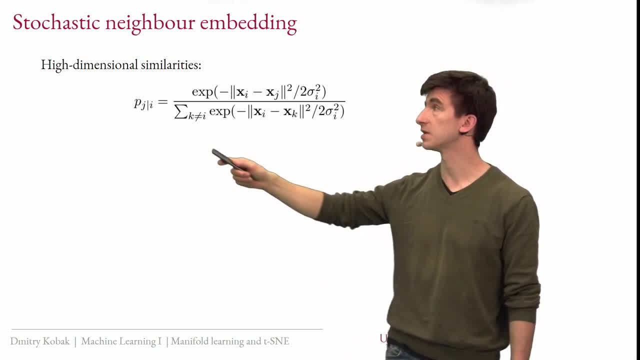 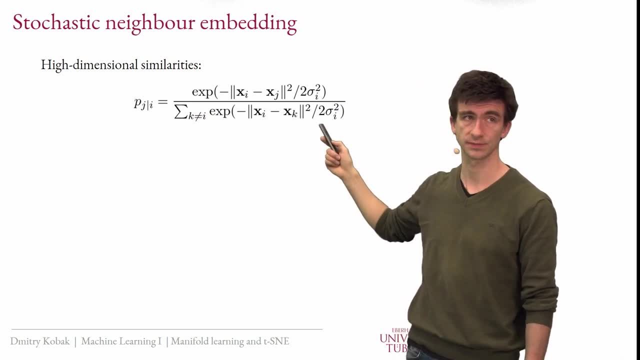 One can call it a directional affinity. So Pji is not equal to Pij over here. And notice that in denominator we're just normalizing everything so that this thing sums to one. Okay, The larger the distance, the smaller the affinity, and they sum to one per point. 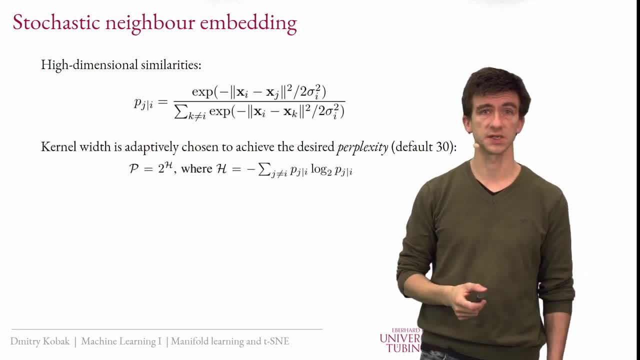 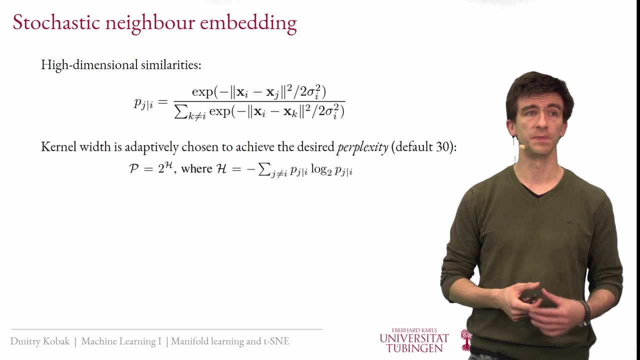 And there is the sigma. i squared term here. So this is a variance of this Gaussian kernel. the standard deviation And the width of the kernel is chosen adaptively to achieve the so-called Okay, To achieve the desired value of the so-called perplexity. 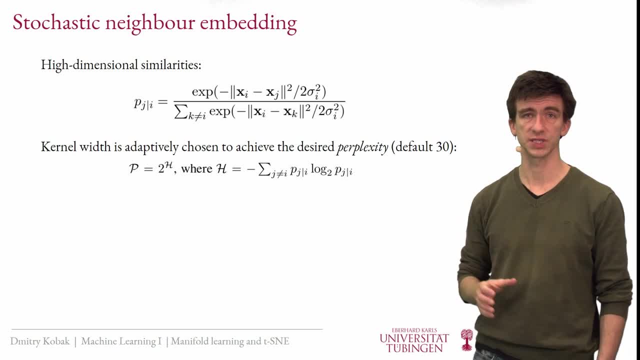 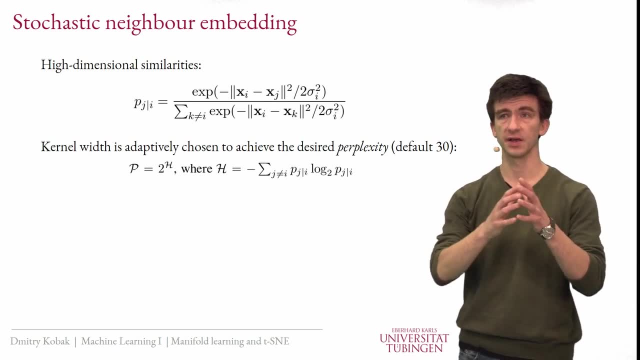 And I don't want to spend too much time explaining that. You will see in a moment why. Think about perplexity as the effective number of neighbors. So if we are in a very dense part of the high dimensional space, then the sigma will be: 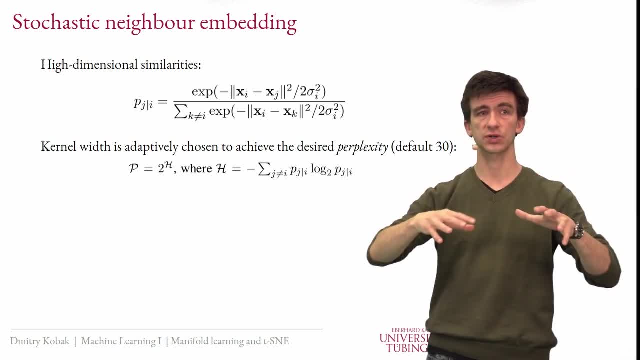 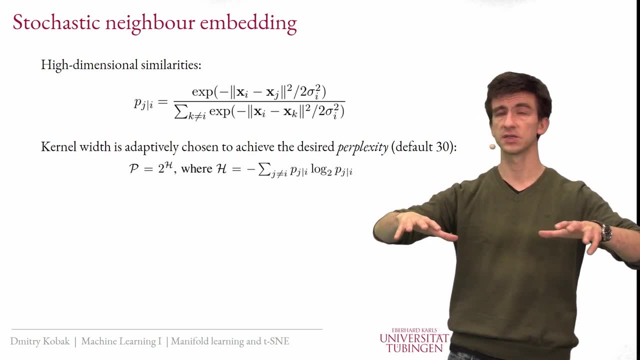 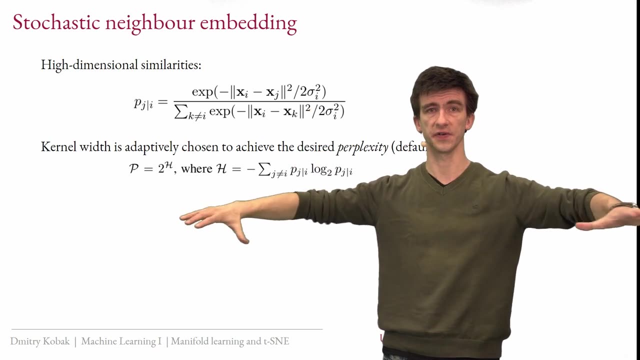 small, so that this Gaussian kernel covers approximately 30 neighbors. Okay, This high dimensional Gaussian kernel, If it's bigger, it's smaller. If it covers around 30 neighbors, then the perplexity is around 30.. If you're in a non-dense, in a very sparse region, then it will be a fat Gaussian. so 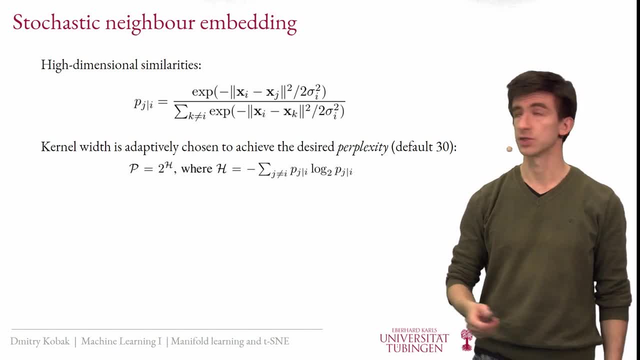 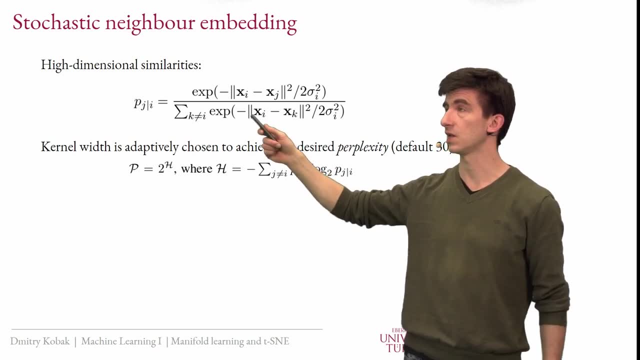 that it again covers approximately 30 neighbors. So we just want that, we want to choose this adaptively- the width of the kernel- so that around 30 values are large And everything else should be much smaller. Okay, That's the intuition here. 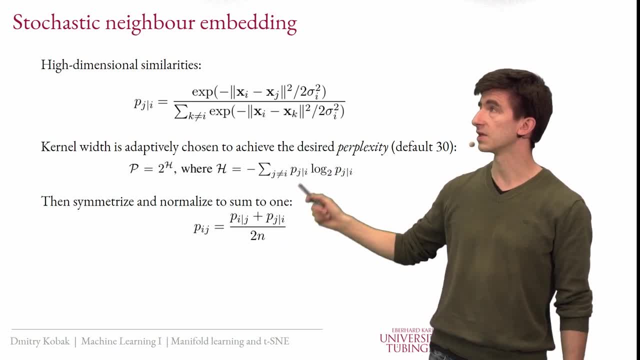 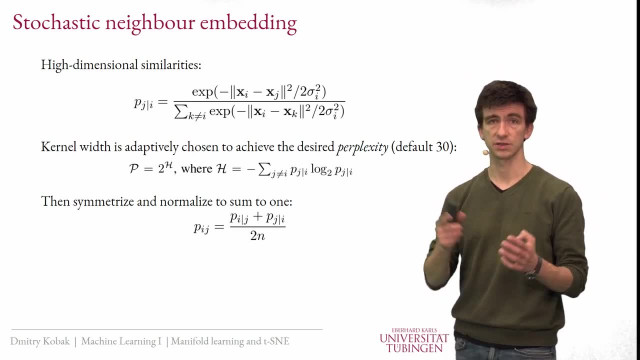 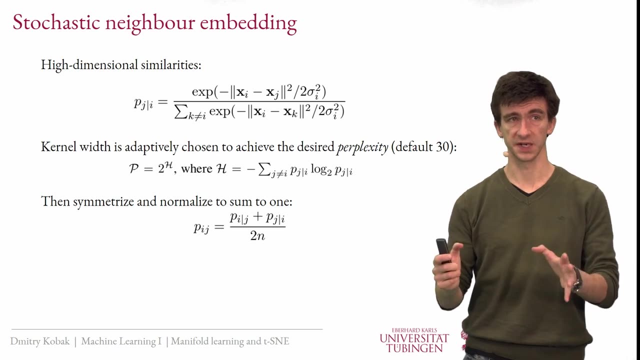 And that's not symmetric. So we'll just symmetrize that And then divide by N so that the entire Pij matrix sums to one. So it's symmetric by construction. It sums to one. by construction, Every point has around 30 large affinities where the perplexity parameter regulates this. 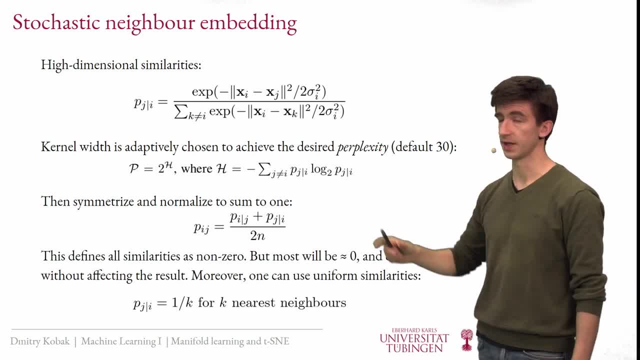 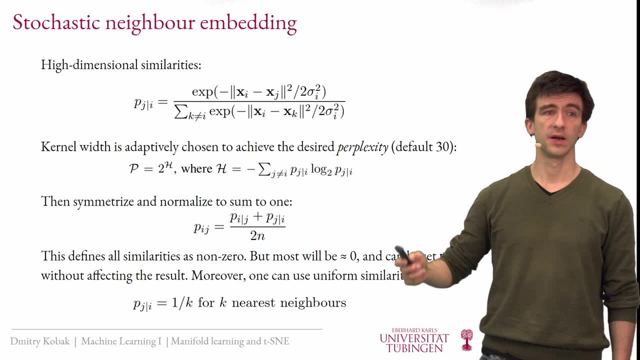 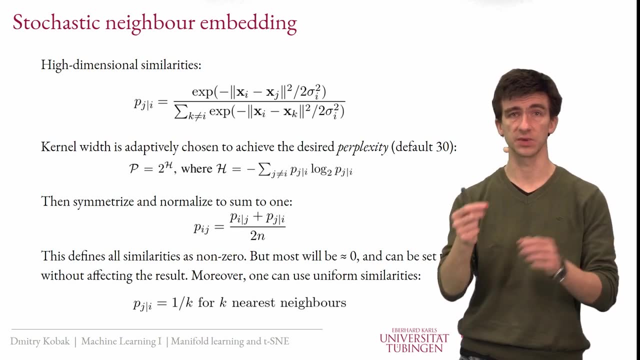 value, And if you're a little bit confused by that, that's okay. But I'm going to show you later that actually this isn't very important. One can define uniform similarities which are much, much simpler. We'll just say: we'll just take 30 nearest neighbor for each point. 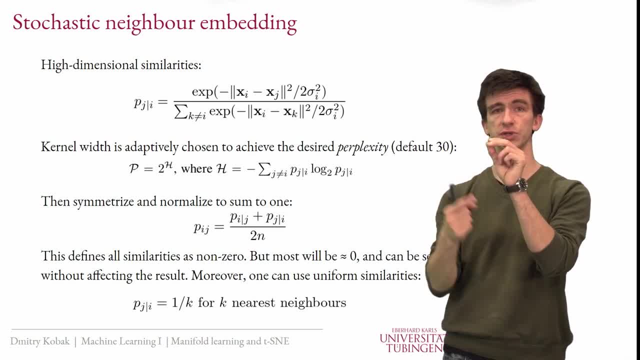 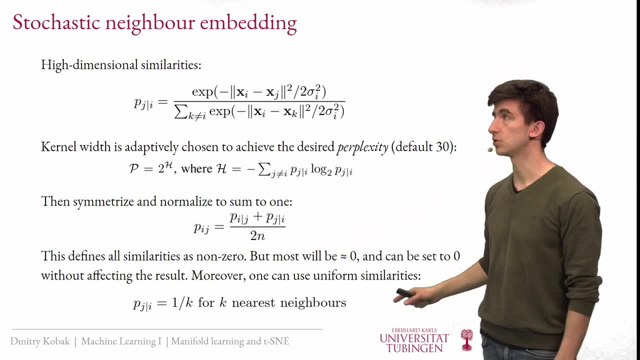 For each point, we take 30 nearest neighbors and say that the affinity all these 30 nearest neighbors is exactly the same: 1 over 30. And it's zero everywhere else. Okay, So this is something I will call uniform similarities. 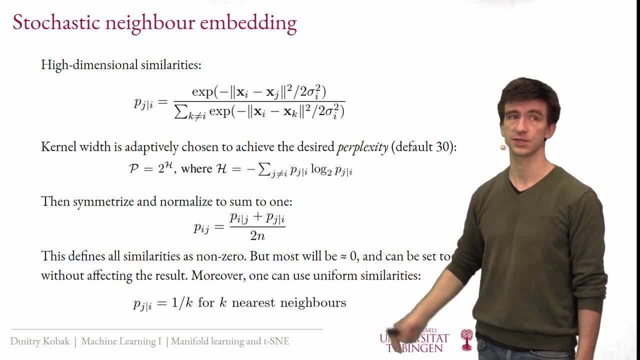 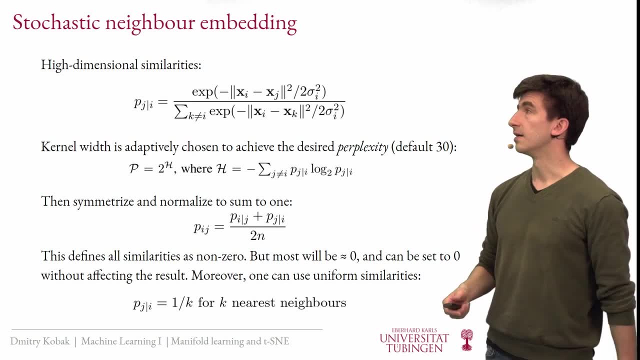 So I'm replacing these two lines by this very simple definition, and I will later show that in most cases it just produces the same. Okay, So it's a very, very similar result. So here all affinities are the same. Here they are not exactly the same. 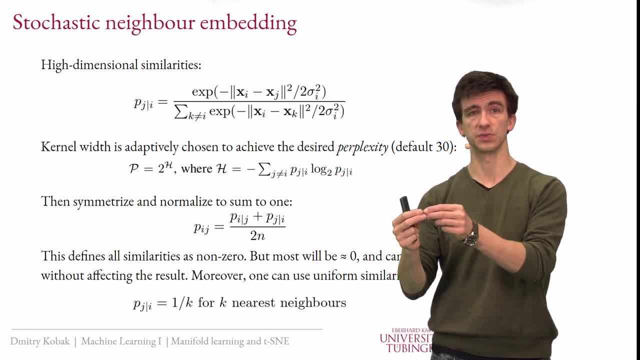 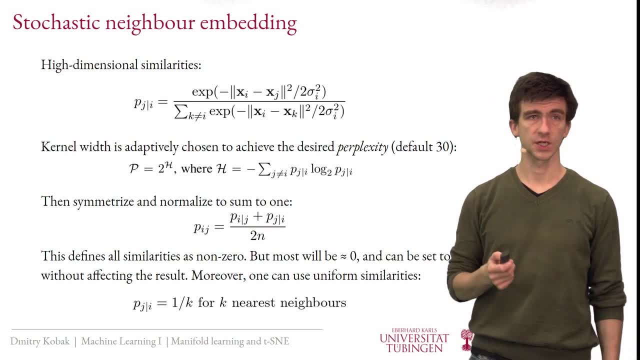 The closest point has a bit larger affinity. The points further away have a bit smaller affinity. Important is that once you go beyond 100 neighbors or so, everything is zero. All right, That's how we define high dimensional similarities. Now the low dimensional similarities are defined similarly. 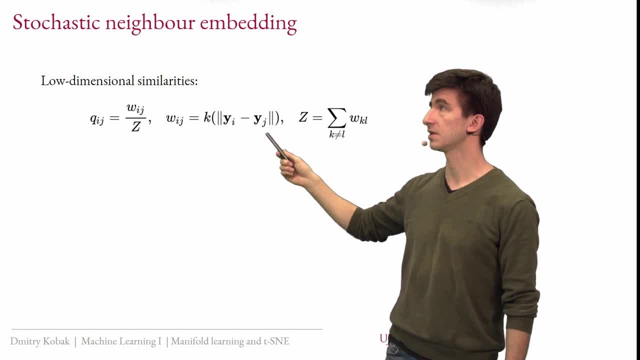 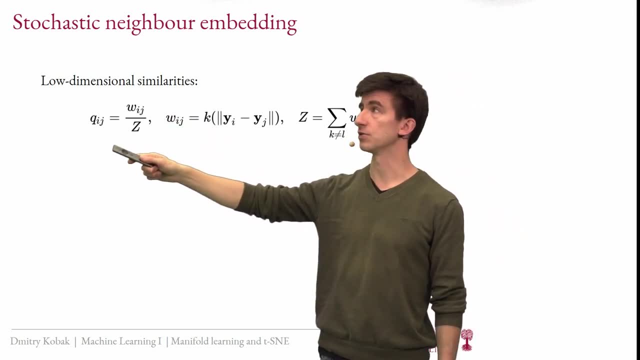 So we compute the distance in the two dimensional embedding. That's my Ys. I put the distance through the kernel, which I will show in a second, and that's my Q. values divided by this normalization factor that just sum over the entire data set. 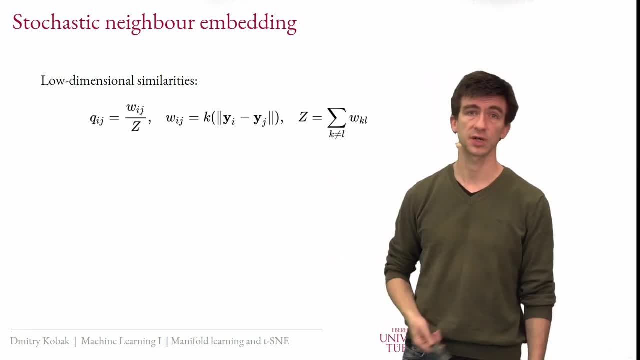 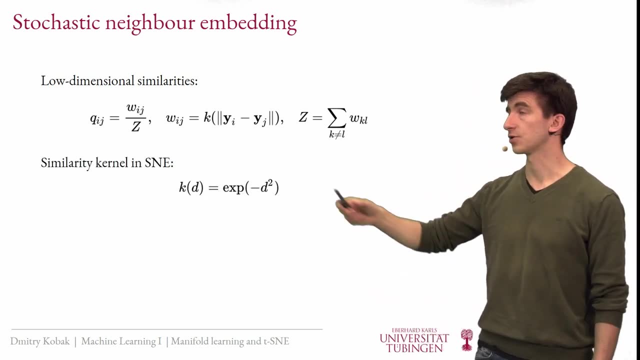 So all pairwise distances here. So this sums to 1 by construction. This is symmetric by construction. We just need to choose this kernel in the original paper, the SNE paper. use the Gaussian kernel here as well. Okay, So that's. 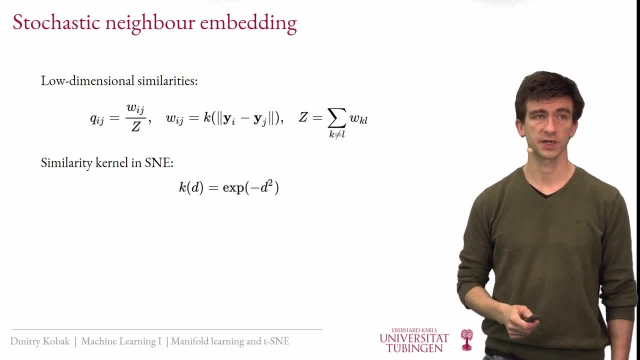 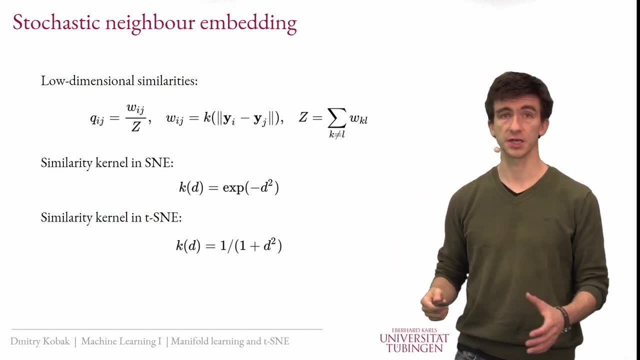 That now concludes the setting up the SNE SNE loss function. T-SNE made one change. It suggested to use a T distribution kernel- In this case it's also Cauchy kernel- Instead. So instead of this function, T-SNE uses that function. 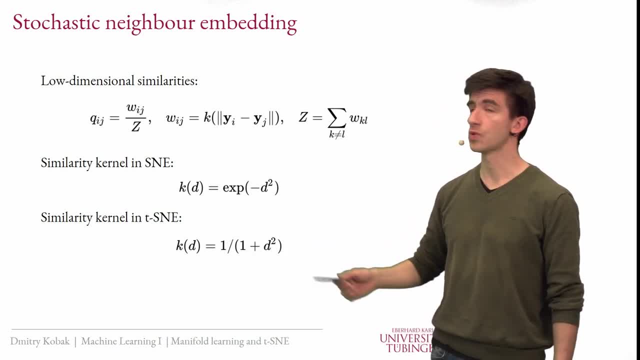 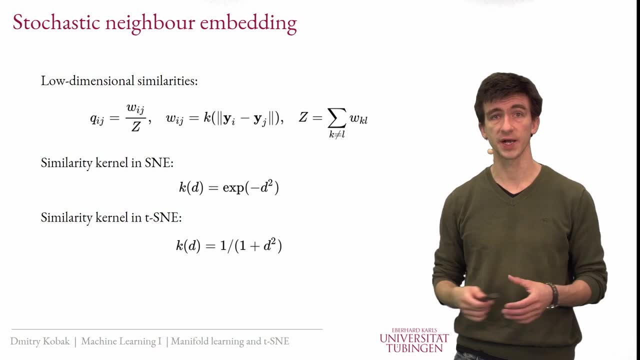 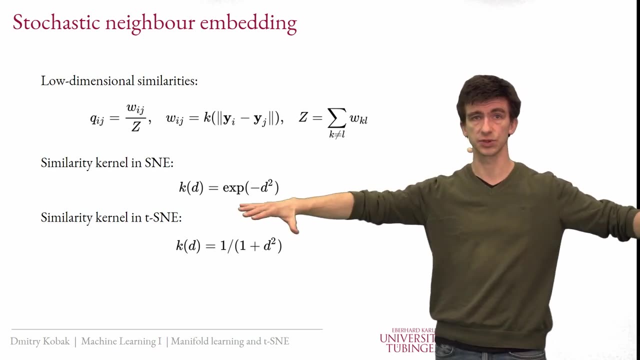 That's the only difference between SNE and T-SNE: One over one plus distance squared. So this thing decays exponentially. This thing decays as one over D squared. So it's called heavy tails. Okay, The Gaussian kernel and the T distribution kernel. the T distribution kernel has heavier, 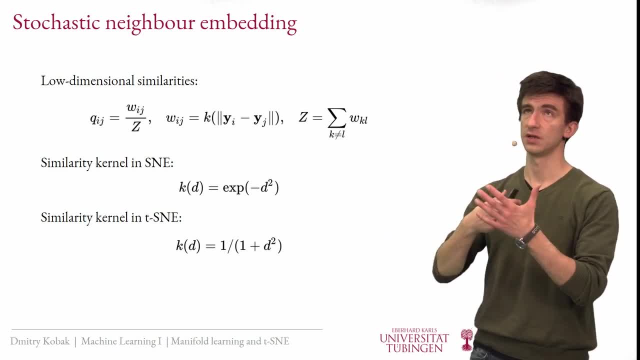 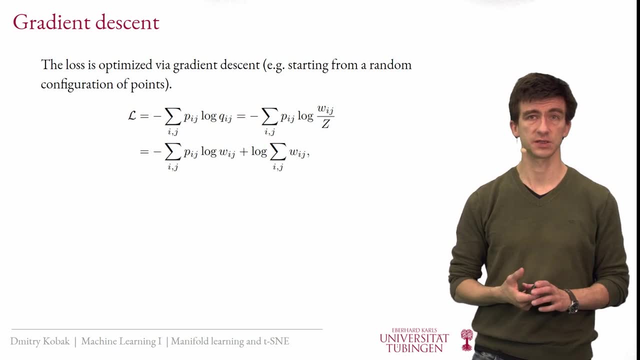 tails. We'll get back to what it means or, no, what it makes, to the embedding in a few slides. Okay, What we need to discuss first is how do we optimize that? So now we have P's, Q's, we have K divergence between P's and Q's- loss function. 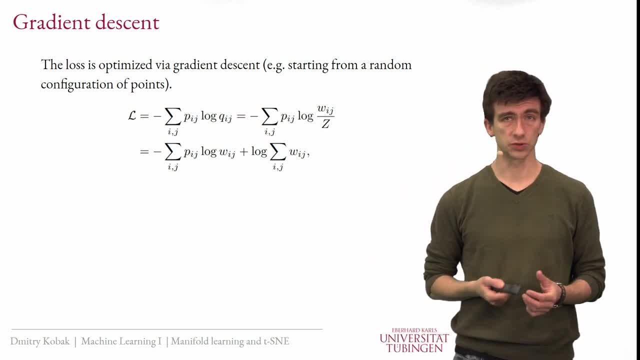 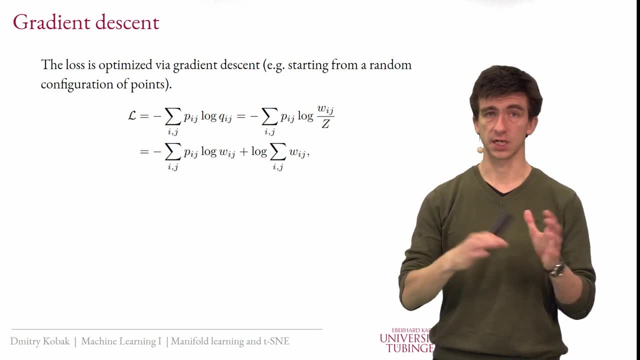 How do we optimize that Turns out, one can just use good old gradient descent, and it works. So the loss is optimized via gradient descent. For example, one can start with a random configuration of points. We will talk about initialization a bit later. 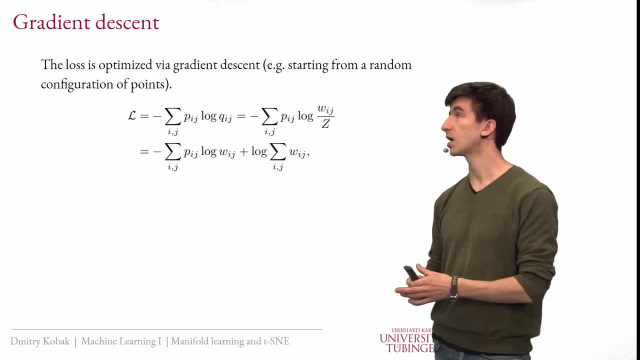 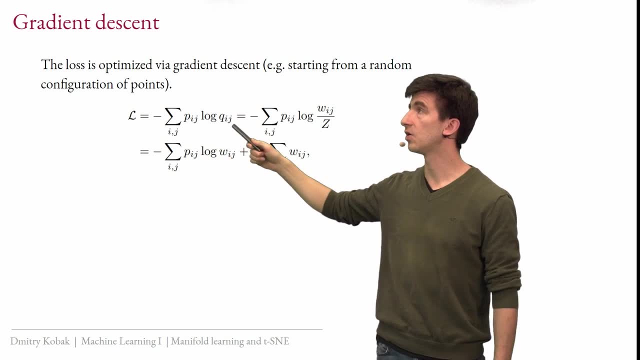 And then just run gradient descent And that's the final embedding that you will get. So let's try to work out quickly how the gradient works here. So the loss is P times the sum of P, of logarithm, of P over Q. So it's actually two terms: P log P. 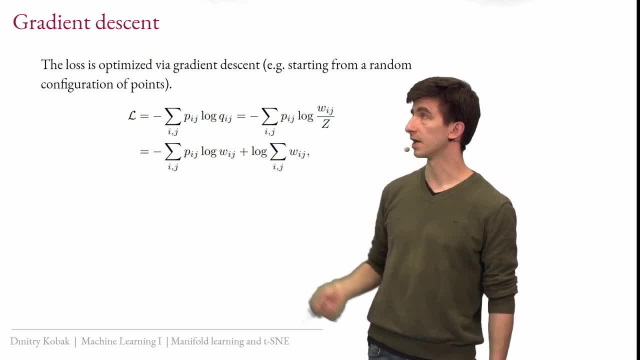 That's a constant. We're not optimizing over it, So I will remove it. I'm not even showing it here. What is left is minus P, logarithm Q. Now remember that the Q was defined as this W, which is the kernel of the distance in low. 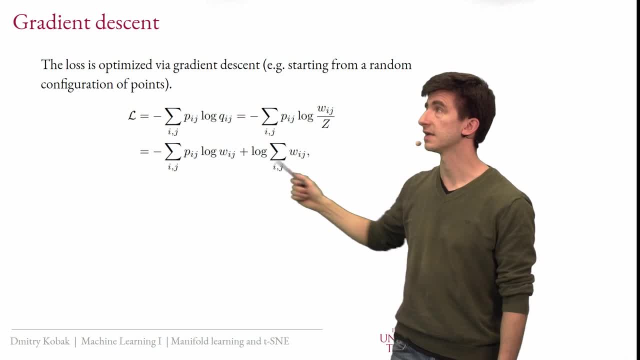 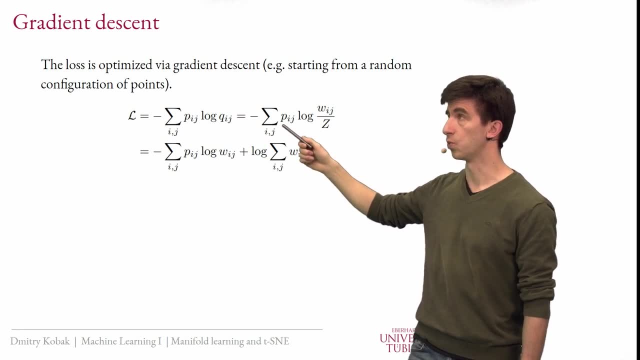 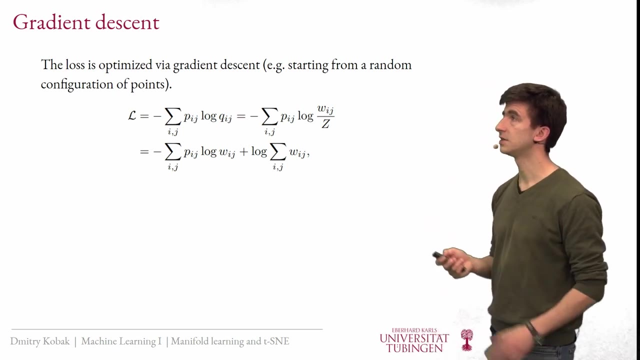 dimensions divided by normalization factor. So I will write it like that here And decompose in two terms. Remember here that the sum of P over all pairs is one, Which is why I can write the second term like that. And now, if we look closely at these two terms, 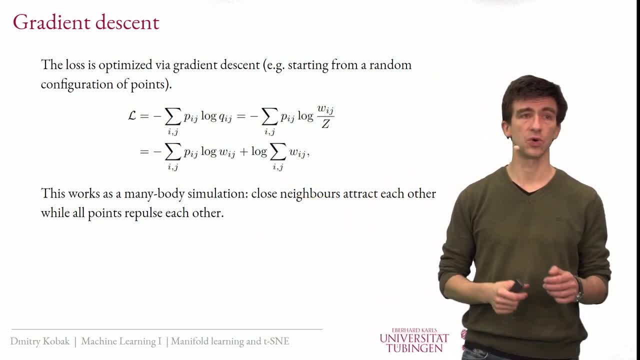 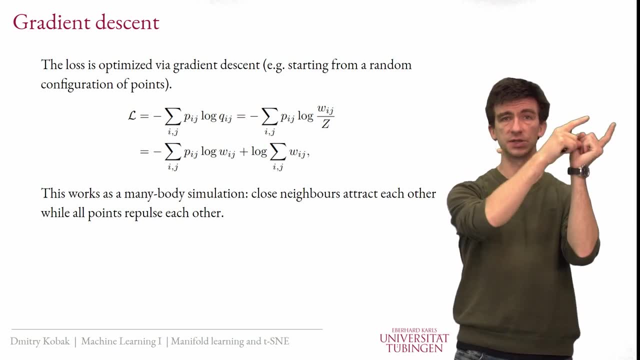 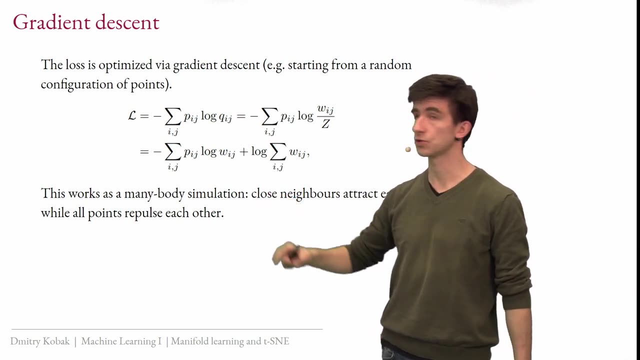 We can see The first term can be interpreted, or it will generate attractive force between two points in the embedding that were neighbors originally, And the second term will generate repulsive forces. So to see that actually one doesn't even need to compute the derivative right. 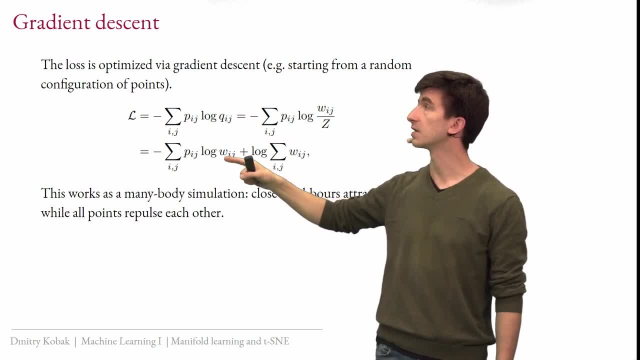 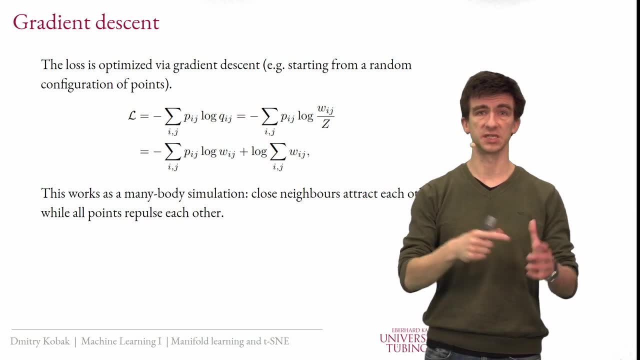 That's not gradient yet, That's just rewriting the loss function. So if we look at that, this has to be small. So wherever P is non-zero, this has to be small, So W has to be small, Which means the distance. 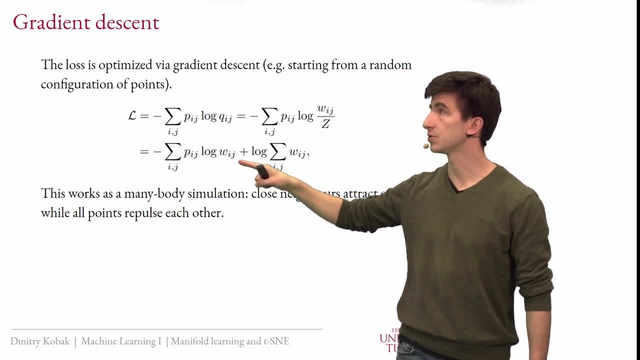 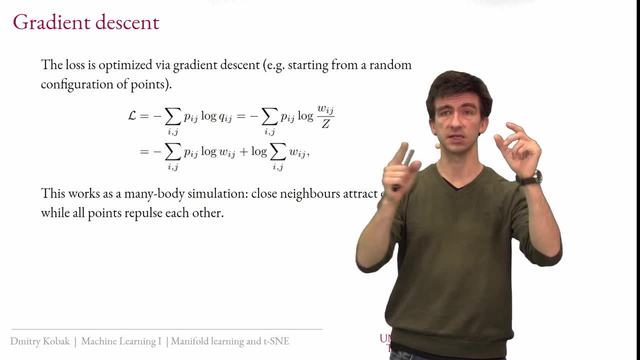 Right, Sorry, There is a minus sign. W has to be large, So the distance has to be small. So wherever two points were neighbors, the distance should be as small as possible in the embedding. So this term will try to pool neighbors together. 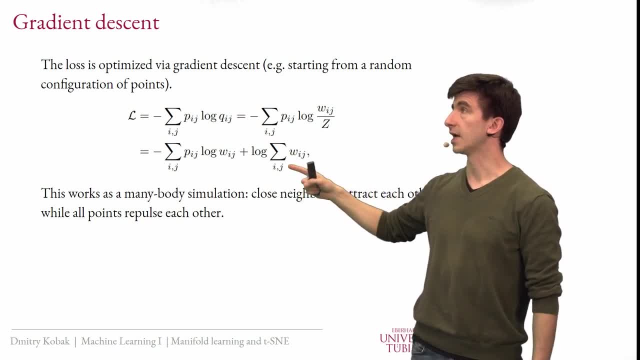 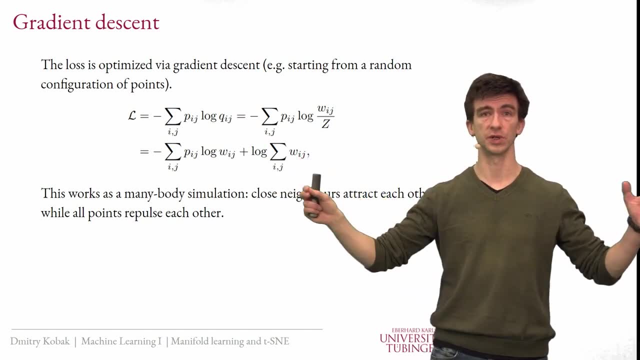 Okay, That's what we want. What does this term do? Again, we want to minimize that, And now there's a plus in front of it. So we want to minimize every W, Which means that the points will fill Repulsive forces. 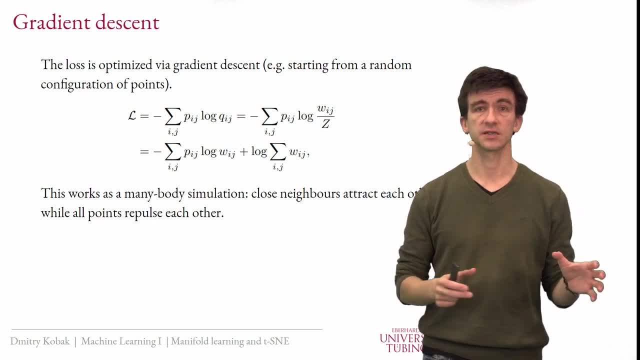 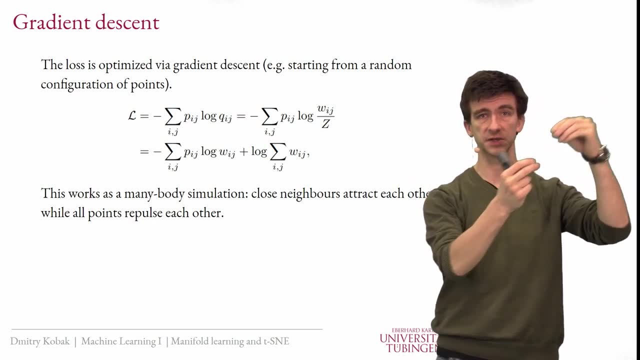 And that's the balance here. So one can. I will show you T-SNE optimization in a second- And it basically works as kind of physical many body simulation. The points are flying around in two dimensions. The neighboring points feel attraction and want to get close. 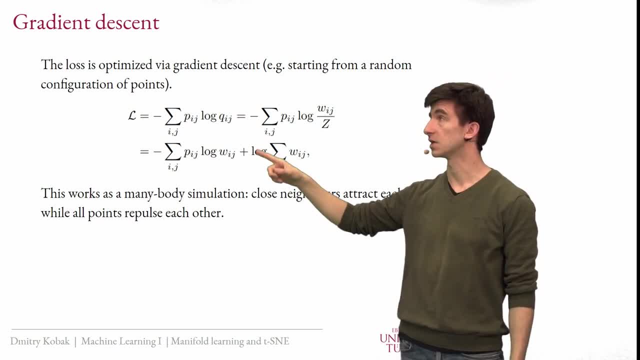 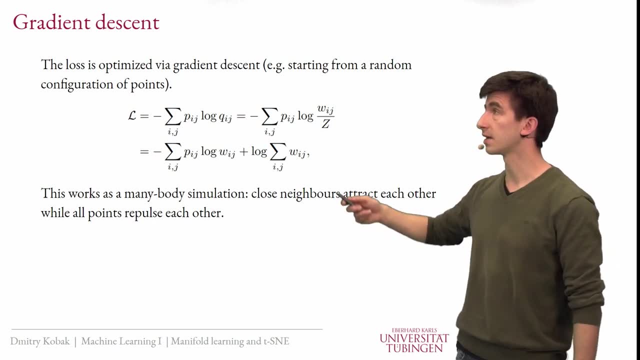 But there's also repulsive force between all pairs of points that originates from this normalization term And there's this balance between attraction and repulsion and in the end we get some embedding. We can compute the gradient. We actually need to take the derivative. 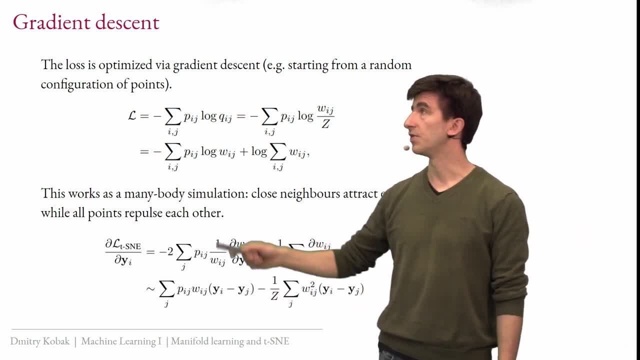 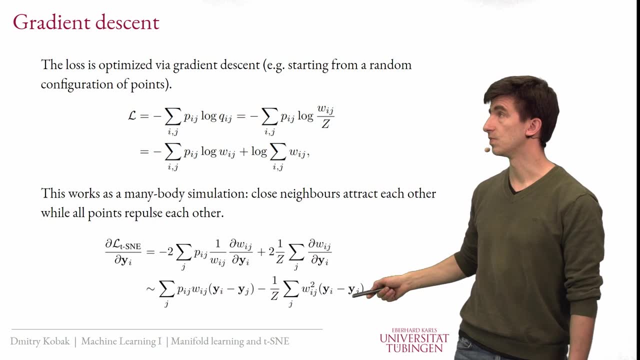 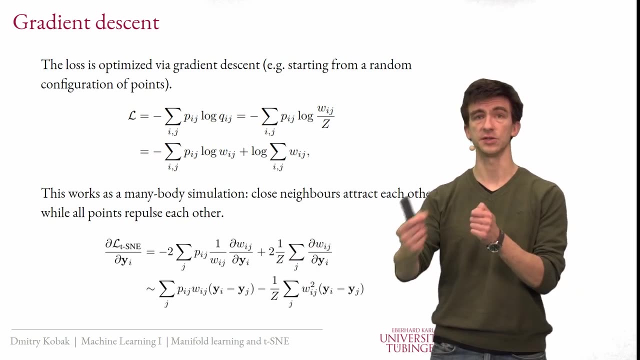 And if one takes the derivative of this, then indeed this term ends up giving you attractive forces And this term ends up giving you repulsive forces. And then, on each iteration, you compute these forces for every point, Make a little step in the direction of this gradient, which just means you move all the 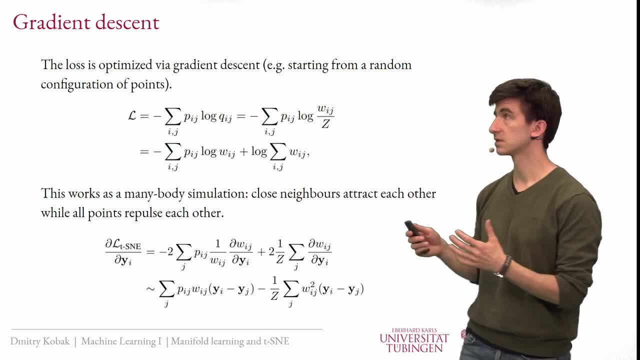 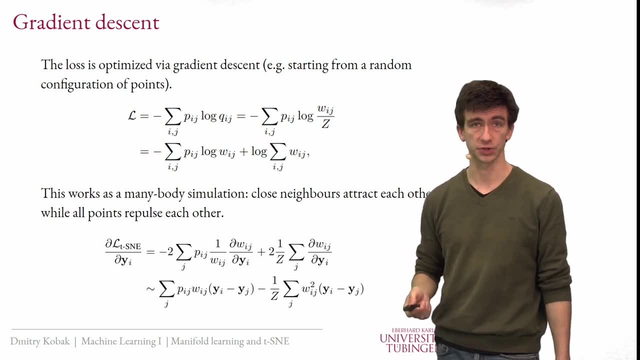 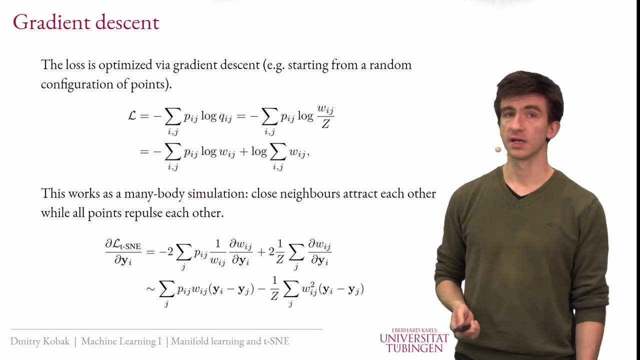 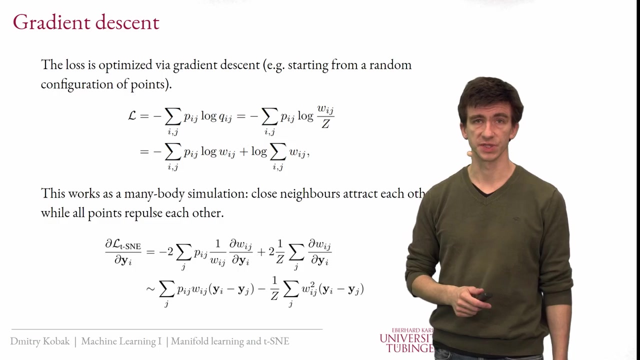 points, Then you recompute the gradient and so on. So that's roughly how the optimization for this, For any method Actually, for multidimensional scaling it works similarly And for T-SNE it also works out like that. So think about this interaction of points as an intuitive picture behind the optimization. 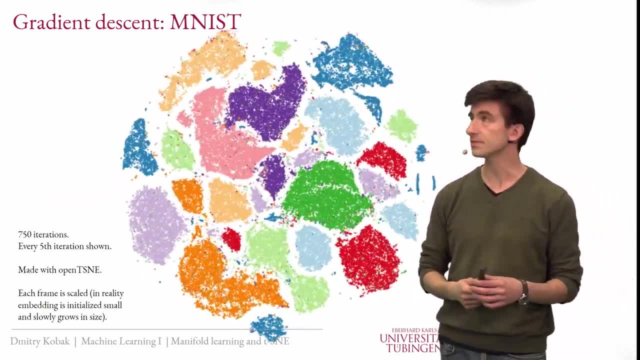 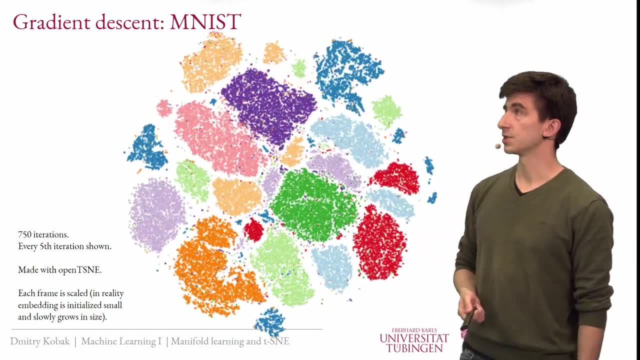 And now I can show you the gradient descent optimization of the MNIST data. I will let it play a few times And notice that we're starting here with random initialization. That's the Gaussian. That's the gradient. That's the gradient. 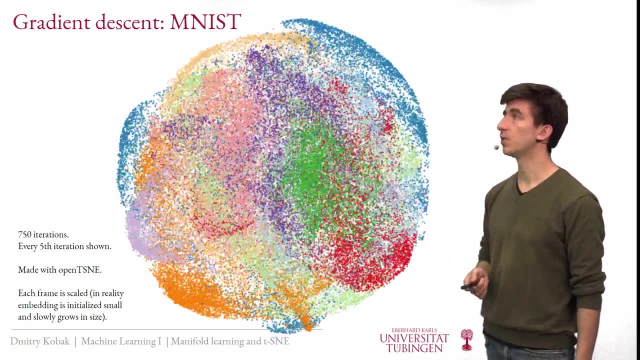 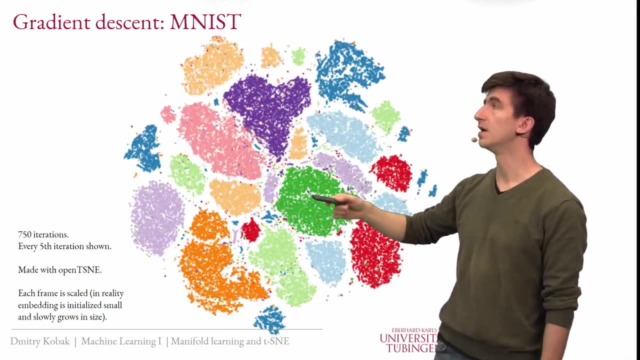 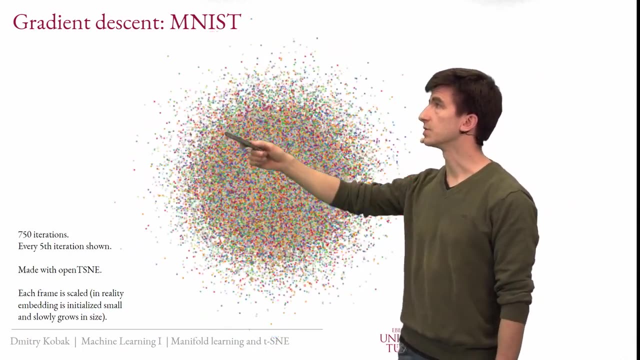 That's the Gaussian blob in the beginning, And then the point starts moving And relatively quickly they form the islands of the same color, which is the same digit, And then slower you see that it gets progressively better. And yeah, I don't know this salmon colored cluster, for example. you can watch that. 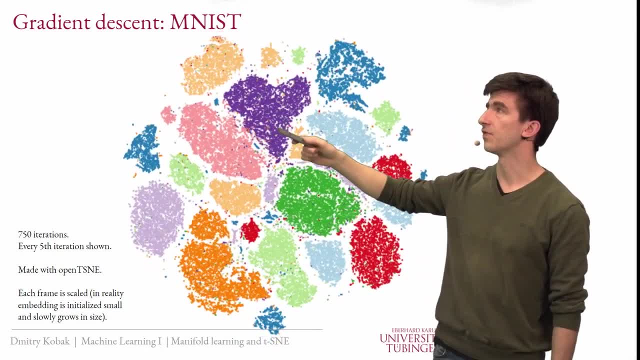 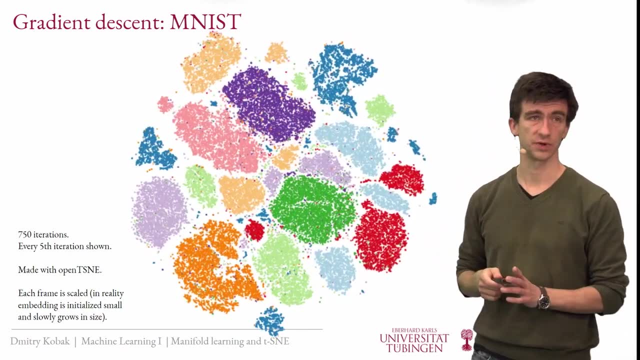 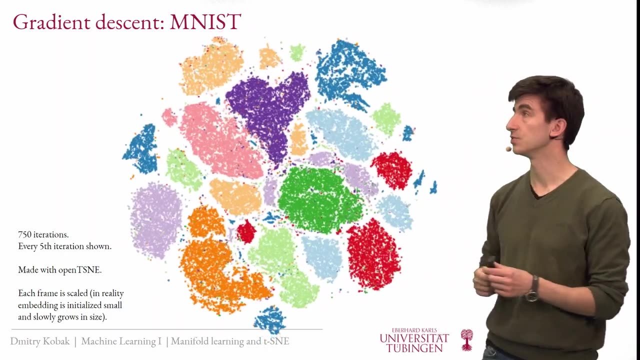 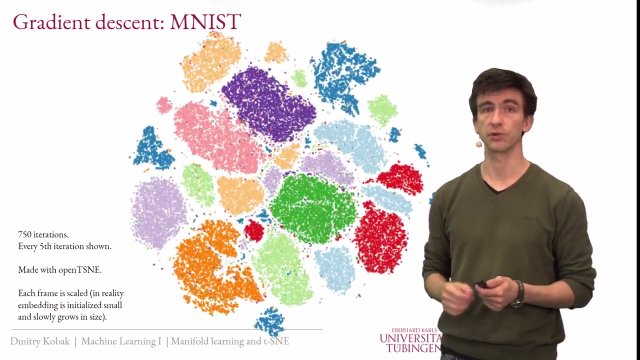 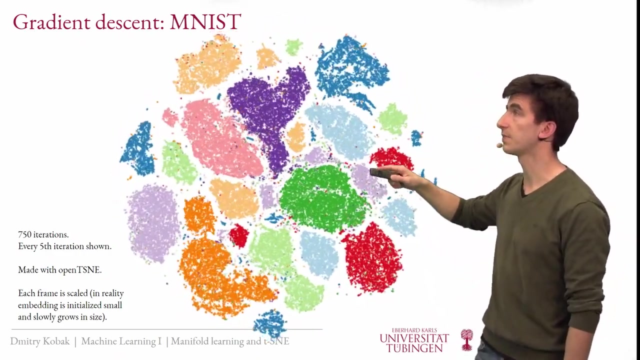 It slowly gets together, And this violet cluster also gets together, and so on. The end result here? The end result here is, though, not as good as I showed before, right, why is it not as good as I showed before? so I'm not doing. I modified it a little bit to show you that, or to say it better, I did not employ one trick that is usually employed. I will tell you about the trick in a second, but let's, I think it's very important to see here and understand why this happens. 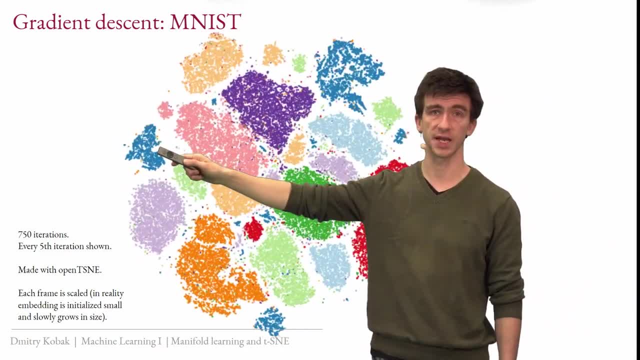 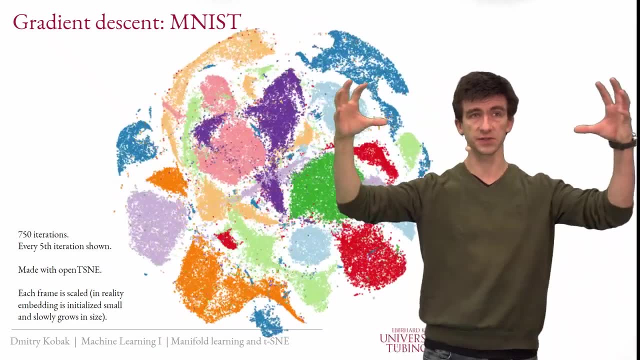 So these blue points and these blue points feel attraction, Some of them are neighbors, They want to get together But There's all this stuff in between and they feel repulsion from that. So these two groups of points, they feel attraction, they want to get closer but they can't. they cannot because of the stuff in between. 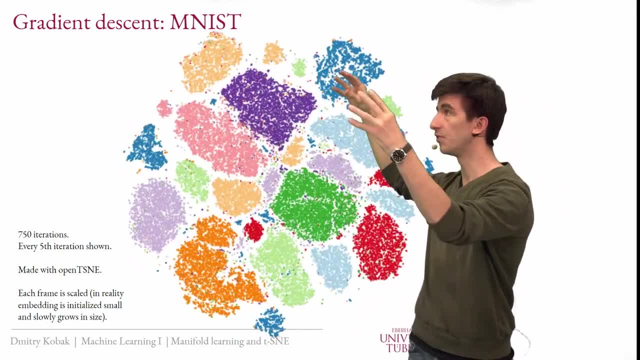 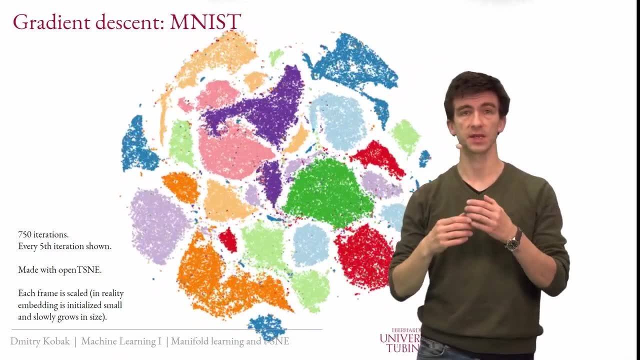 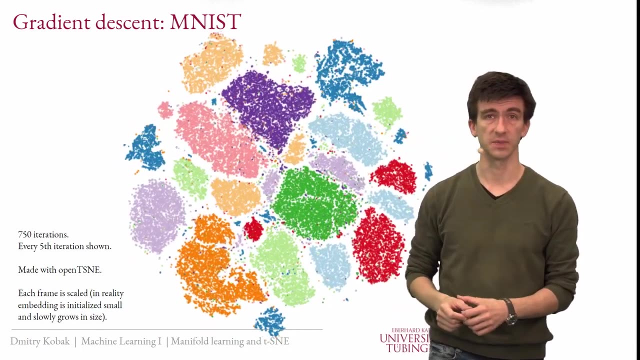 So in the end, you converge to something which is a local minimum. Moving them closer would decrease the loss function. Moving this entire island over there would actually would actually be a better solution, but that's not. you can't get from there from here, so you're stuck in a bad local minimum here. 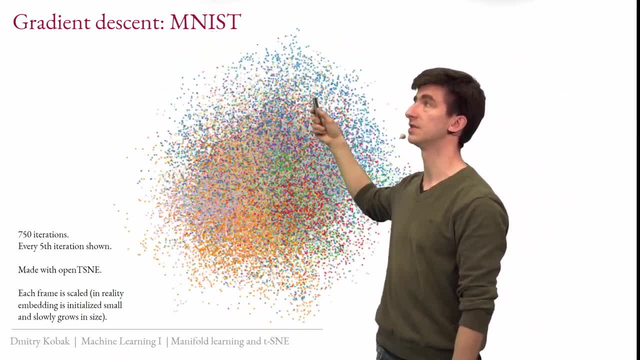 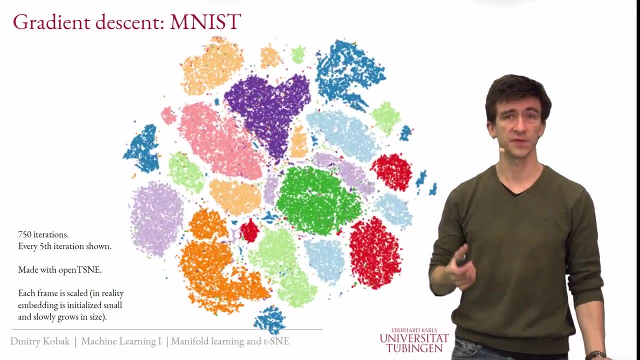 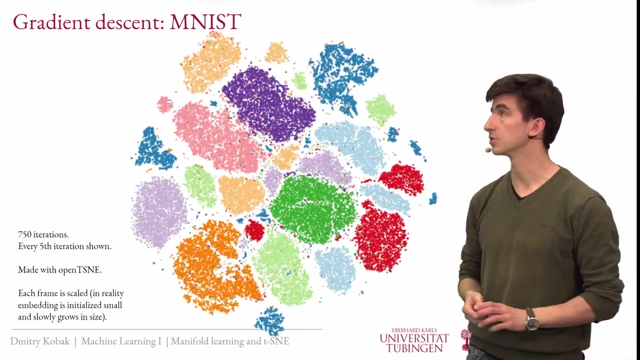 And it happens because the repulsion is too strong. in a way It does not allow these things to get together, even though they want to. That's the intuitive, intuitive picture of that. So how can we fix that? And in fact, already the original papers suggested a very useful trick: how to how to do it better. 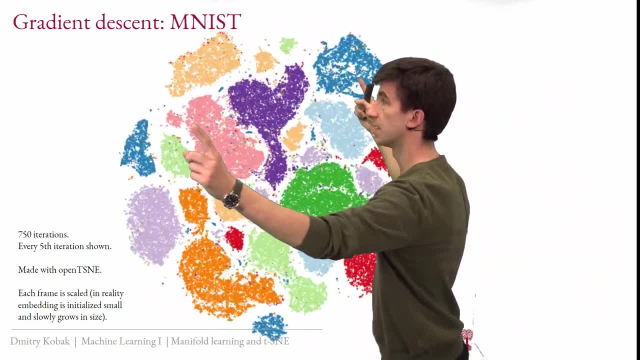 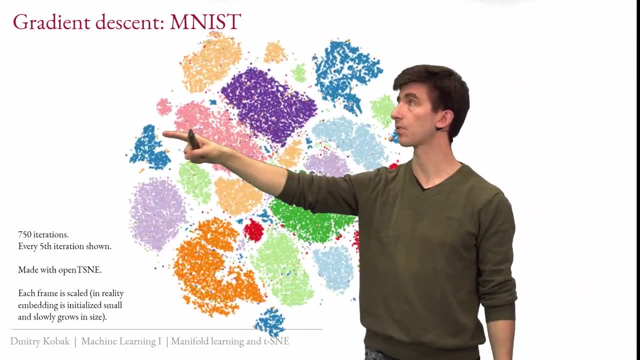 And the trick is well, they can't. they want to get together, but they can't get together, right These things. So let's increase all attractive forces temporarily And hopefully this will let them Go through this whole clusters in between and and connect, and then we'll decrease it again. 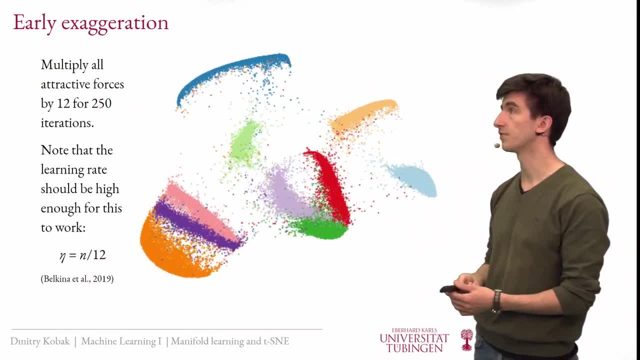 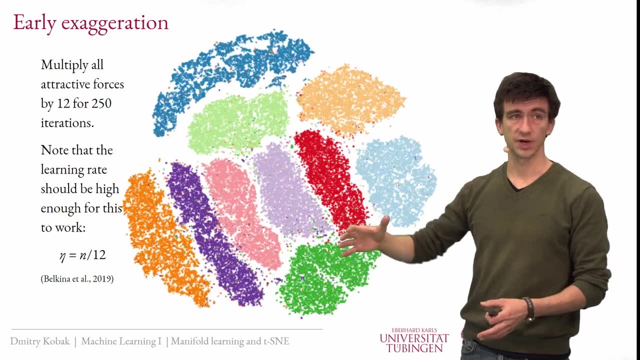 So this is a trick called early exaggeration, and I'm showing the animation of MNIST using early exaggeration. And now you see, it's, it's, it's much better Now. everything is very neatly separated And, importantly, I started from the same random initialization as on the previous slide. 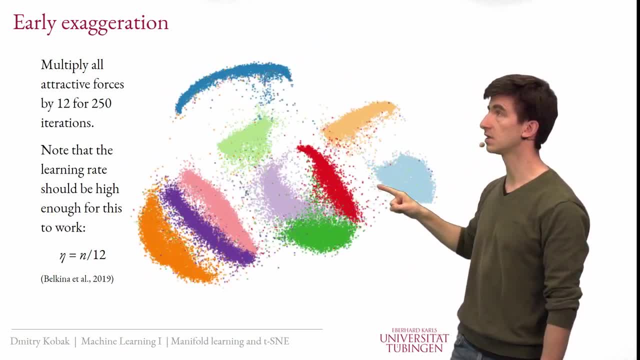 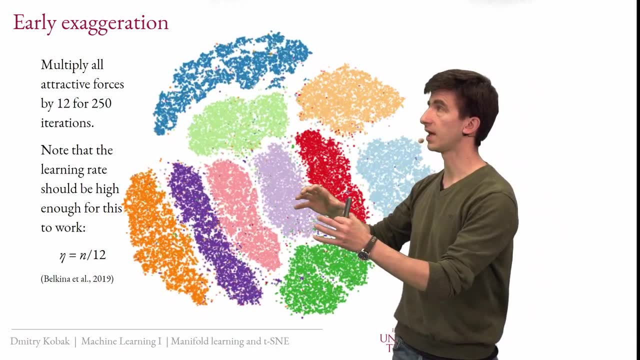 Okay, And here it works, because until now- look here now. now the early exaggeration was turned off And until it was turned off It, the attraction was so strong that every, every digit, so every cluster, could collect together right here. 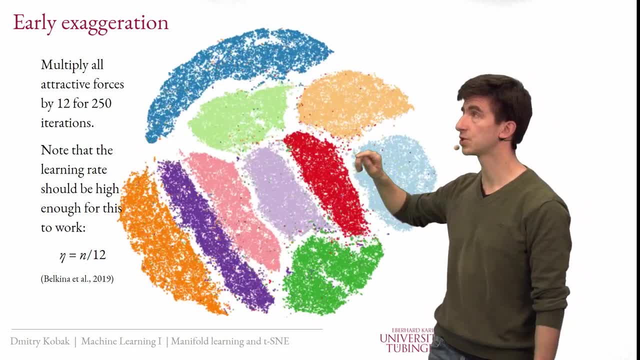 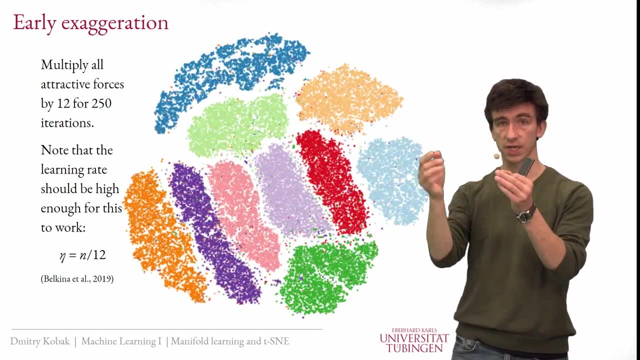 And it's actually interesting embedding in its own right. We'll get back to it a bit later. Then we turn the early exaggeration off And that's the moment where every cluster expands a bit, because now repulsion attraction is weaker, repulsion is stronger and you get the final t-th new result. 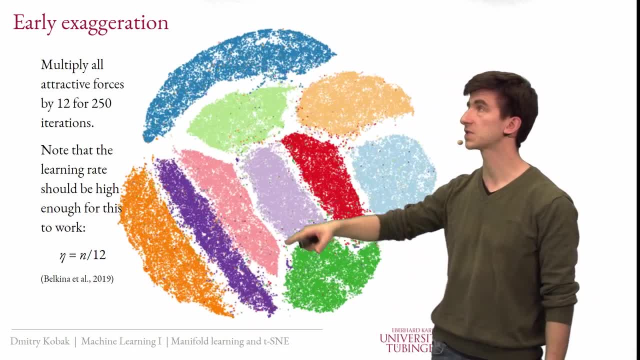 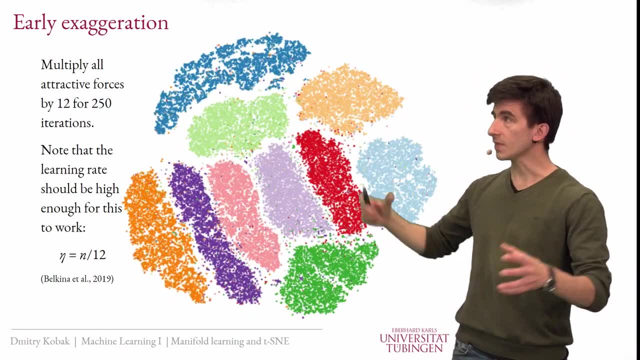 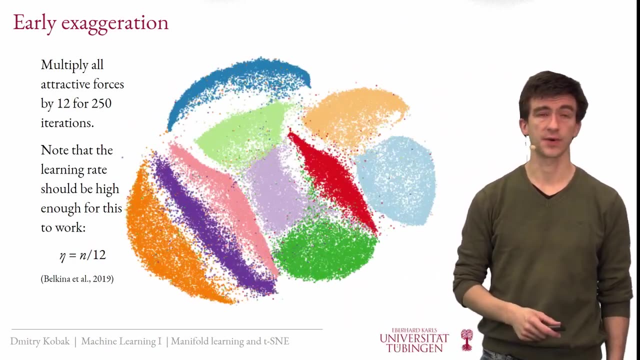 It's important that the learning rate is is large enough so that there's enough time in these early iterations- 250. Gradient descent iterations by default for early exaggeration to work. But there is a good heuristic for the learning rate actually suggested recently. that does the trick. 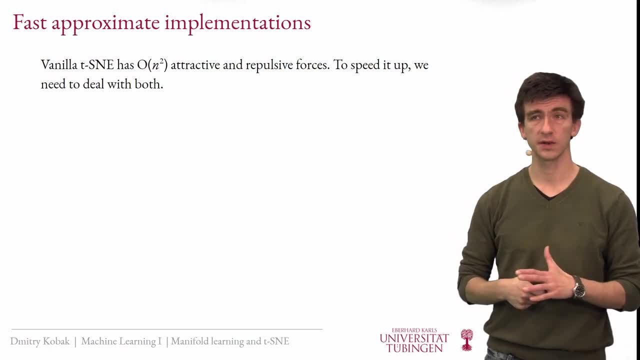 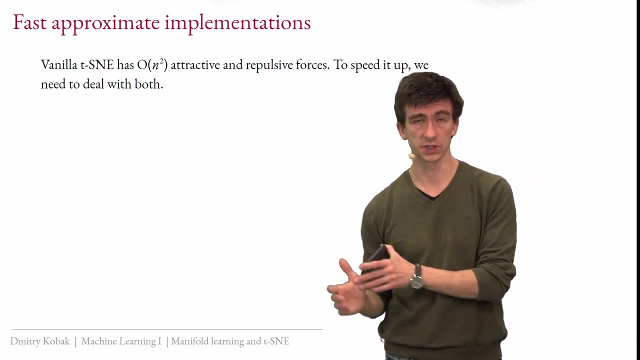 Okay. So one final but a very important remark here, or a topic, is that well, if we want to scale t-th new up, For even for MNIST, 70,000 points, but maybe beyond, for 700 points, 700,000 points, seven million points. 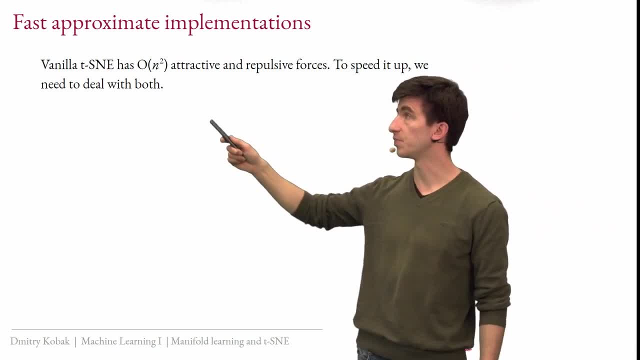 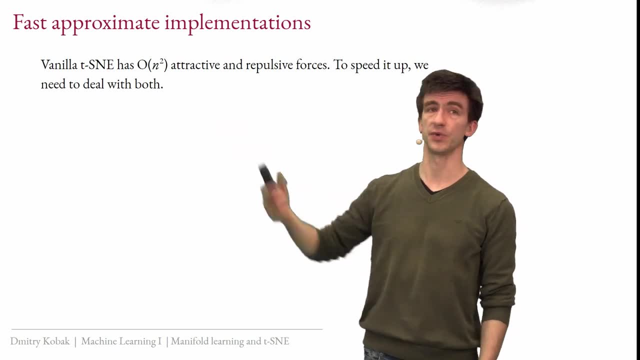 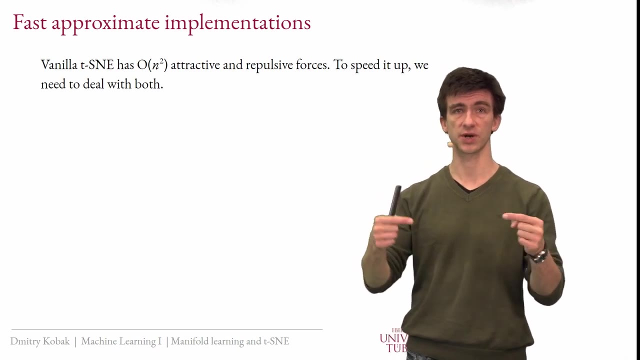 Then we need to, somehow, we need to think, we need to, to speed it up, because naively, you compute the pairwise distances between all points In high dimensions. in low dimensions, that's N squared memory and N squared complexity, Because in each gradient, descent iteration you need to take care of all pairwise forces. 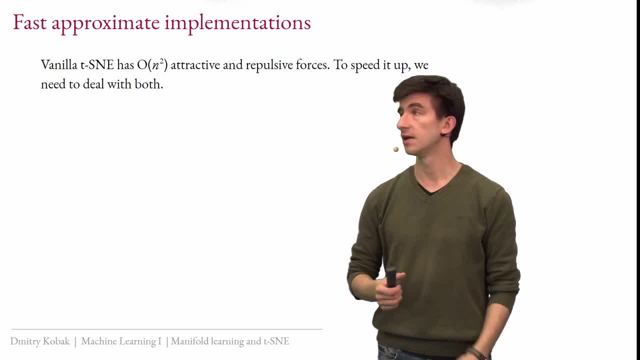 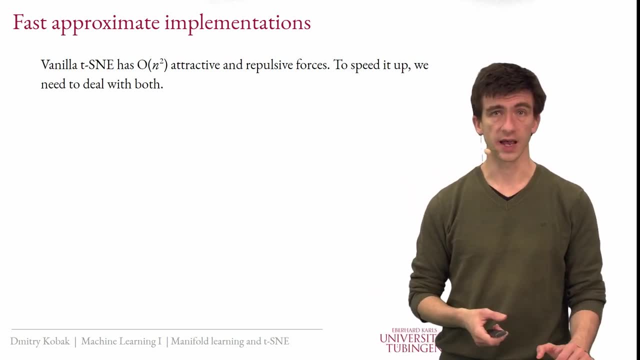 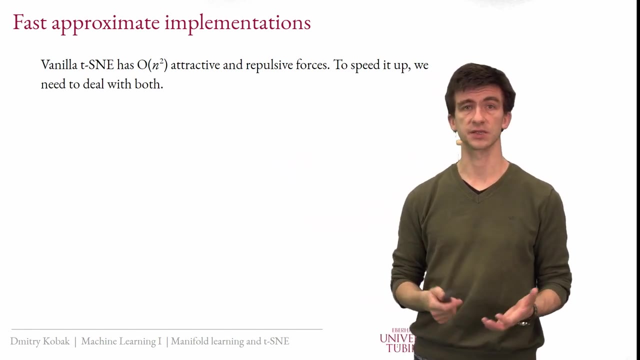 There was attraction, There's also repulsion between all pairs of points, So that's clearly. this is not going to work. So in order to use it- and I already used it in these MNIST animations- We need to do something with attractive forces and with repulsive forces to make it feasible. 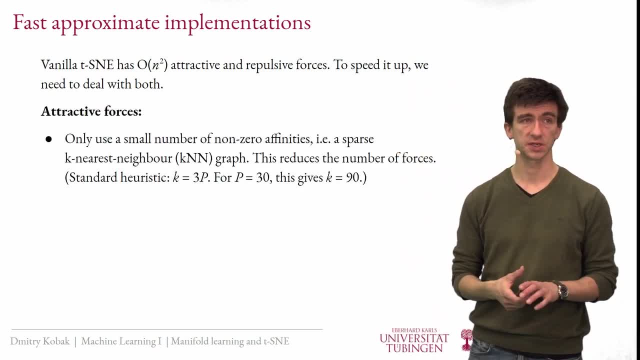 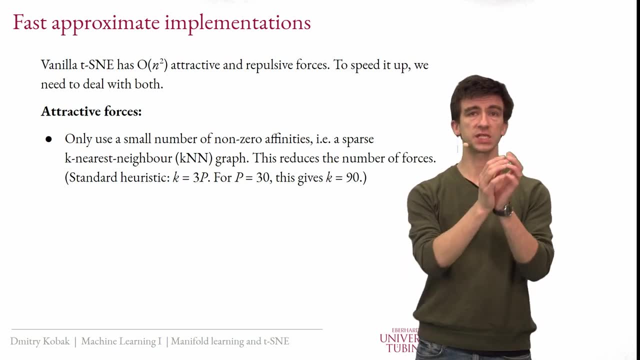 So let's discuss them separately. Attractive forces first. So attractive forces, that's the easier part, Only small. I already told you, only a small number of similarities will be will be large, Most similarities, even if you compute the entire distance matrix all n-squared. 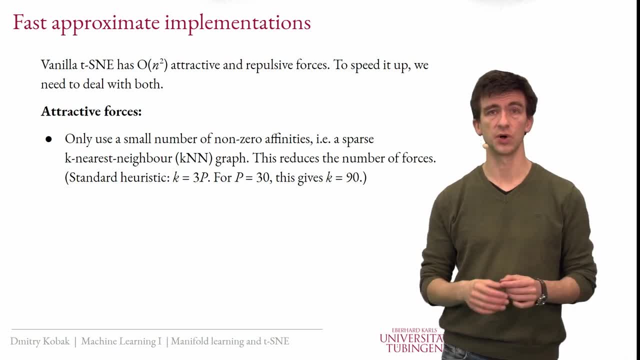 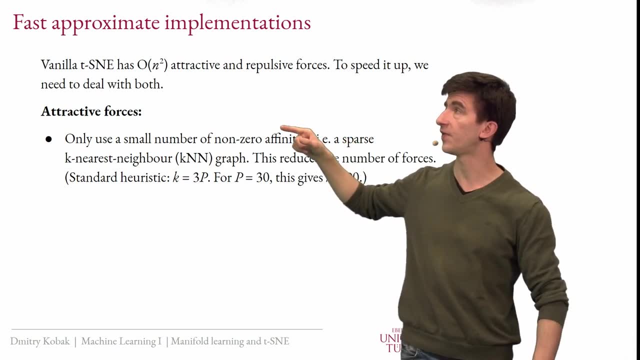 values and then put them through the Gaussian kernel, most of them will be around zero. So we can say we're not going to compute these near-zero values. We will just, for each point, find its nearest neighbors, a small set of nearest neighbors. That's called constructing a k-nearest neighbor. 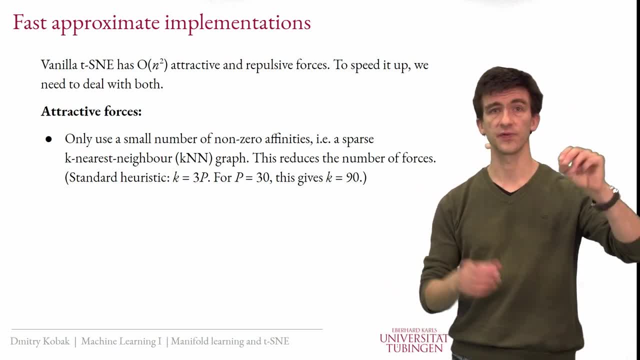 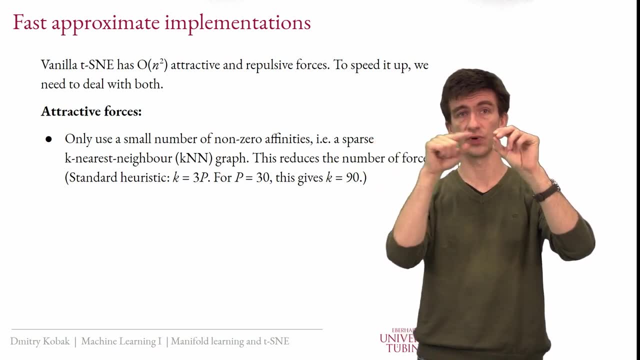 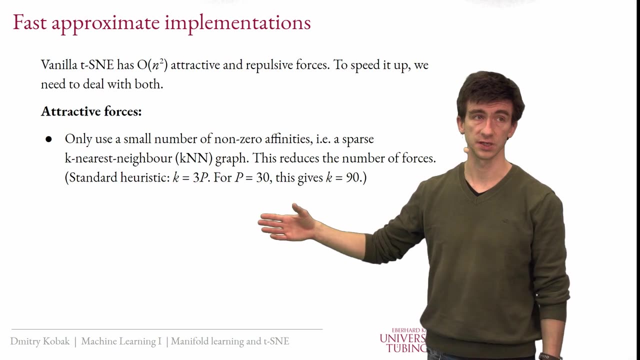 KNN graph of the data. So it's a graph where every point, every sample is a point and if a point is a nearest neighbor among the nearest neighbors of some other point, then there's an edge between them. That's a graph. So, for example, if you want to use perplexity 30, which is the standard, 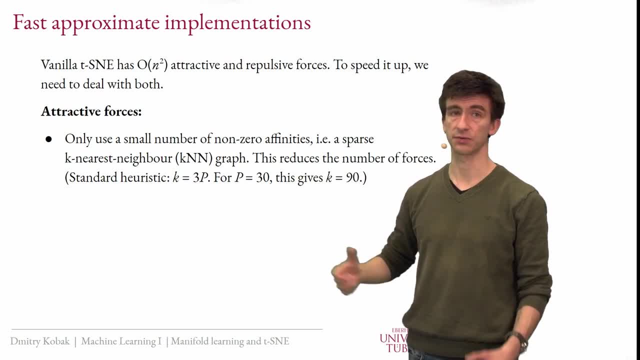 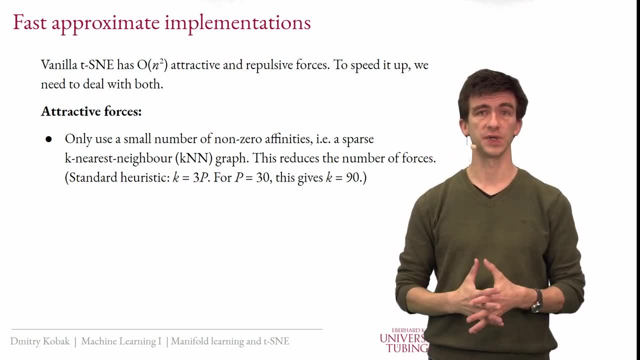 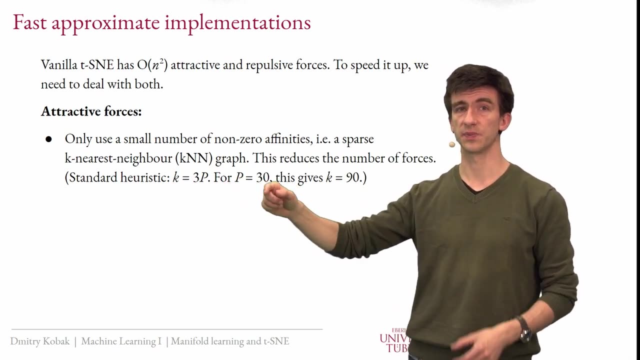 default choice for t-SNE. then we can take 90,, three times larger k for the KNN graph, find 90 neighbors of each point and compute this Gaussian similarity between them, And by the time you go to 90th nearest neighbor, the PIJ is. 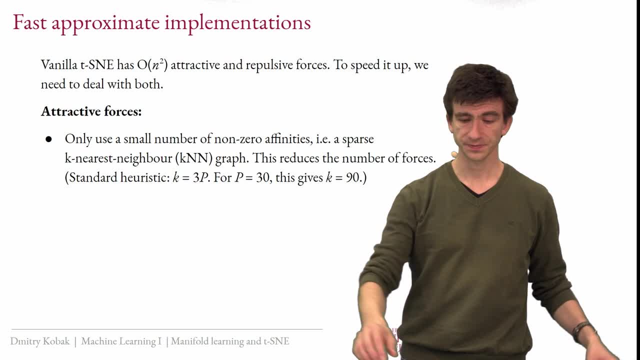 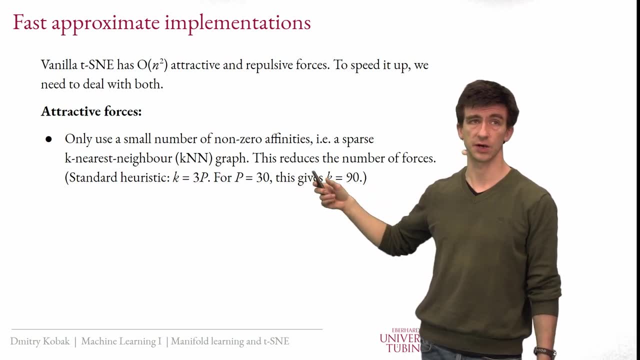 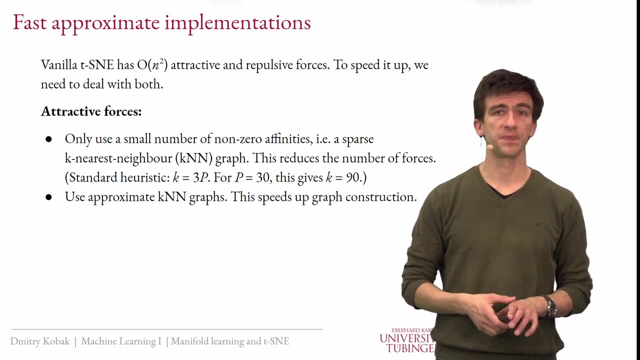 basically zero, and for everything else we'll just say it's exactly zero. This makes it a lot faster. the optimization, because you don't need to. you don't now. you don't have n-squared attractive forces. you have n times 90 attractive forces. roughly, But even. 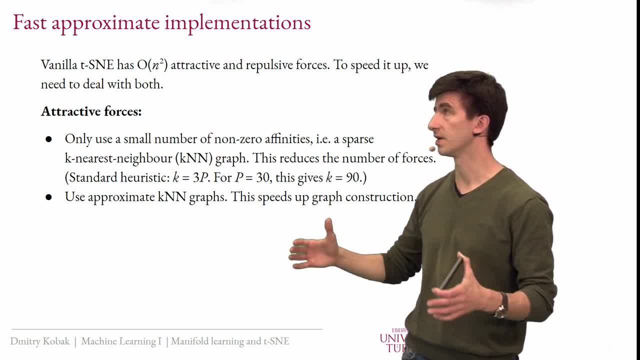 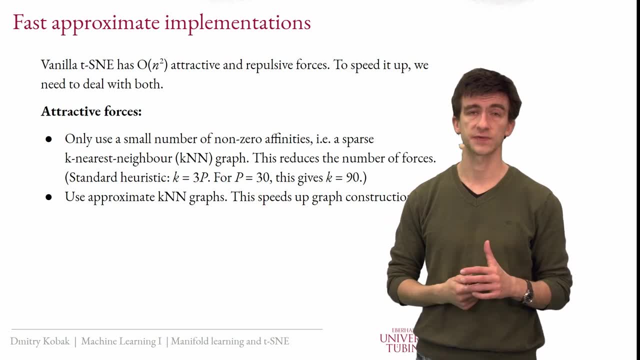 a lot of the larger gain you get, or maybe another- just I'm not sure what's larger- but another very large gain you can get if you use something called approximate KNN graph. So it turns out- and this is something I don't have time to cover today- that there are algorithms, even different approaches to constructing. 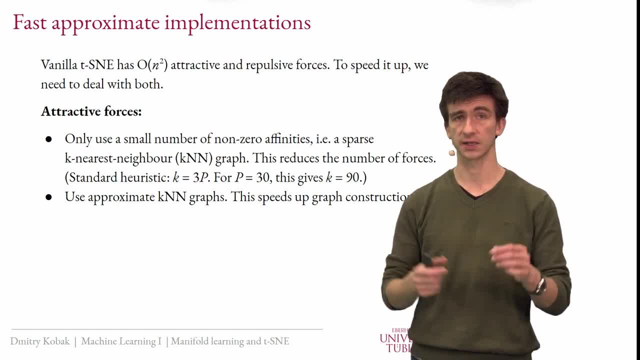 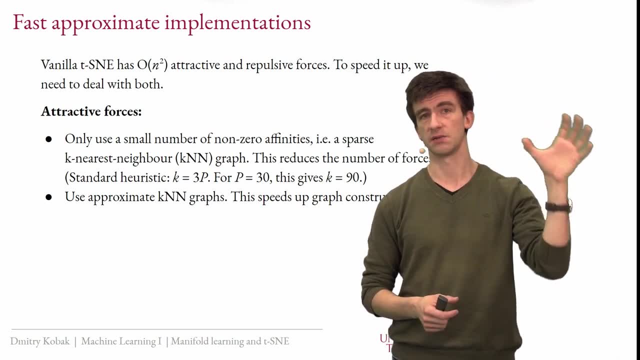 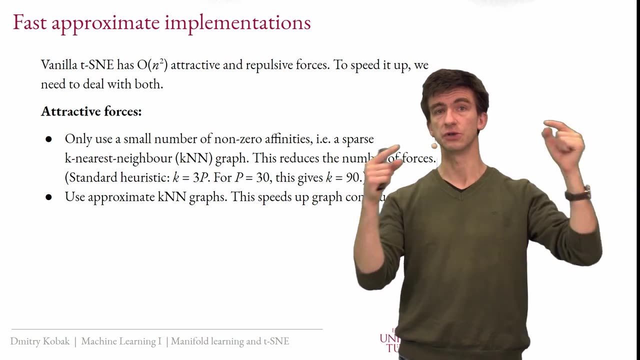 KNN graph- approximately Approximate. KNN graph means you construct a KNN graph but there can be errors. So maybe you find 90 neighbors for each point, but actually only eight. five are really the 90 nearest neighbors and five points that you found as nearest neighbors are not really. 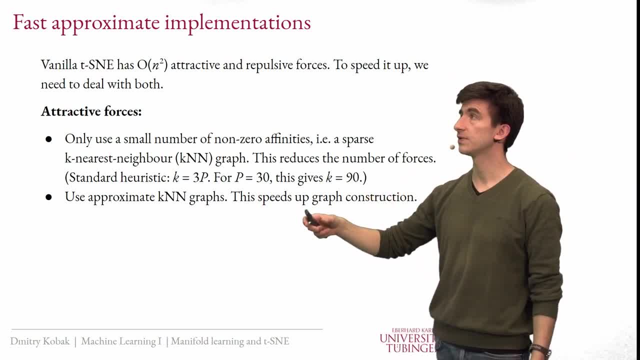 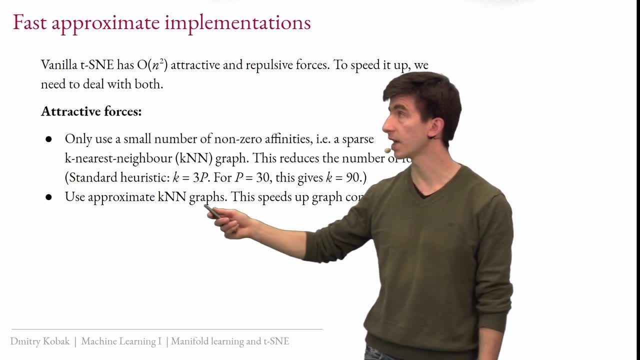 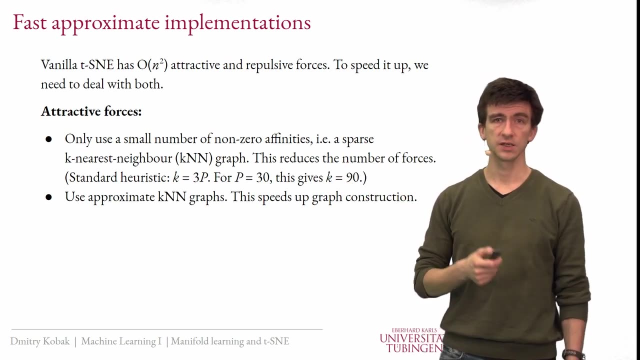 nearest neighbors, but it works well enough, so that doesn't make any difference for t's new, for example, and it still works exactly as well. so these algorithms are great, work pretty good, and they're much, much faster than finding the exact canon graph. so that allows us to deal with the 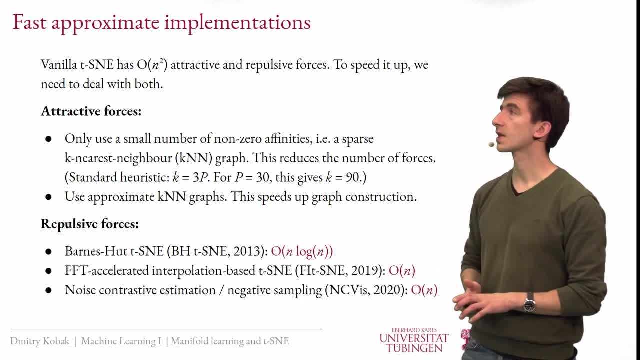 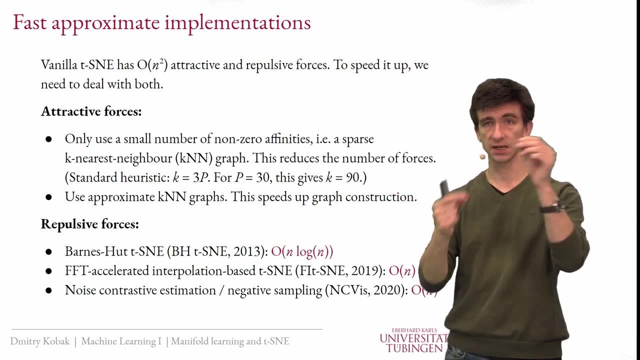 attractive forces effectively for repulsive forces. um, that's a whole large topic that i don't have time to discuss in detail, but there is. different approaches were suggested over the years of how to approximately compute these repulsive forces between all points. so instead of computing exactly all n squared repulsive forces, we're computing them approximately. so there are. 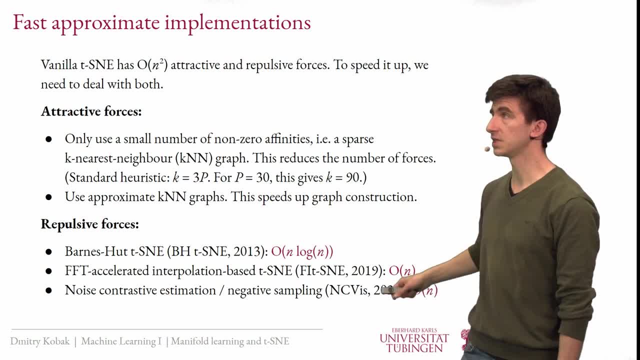 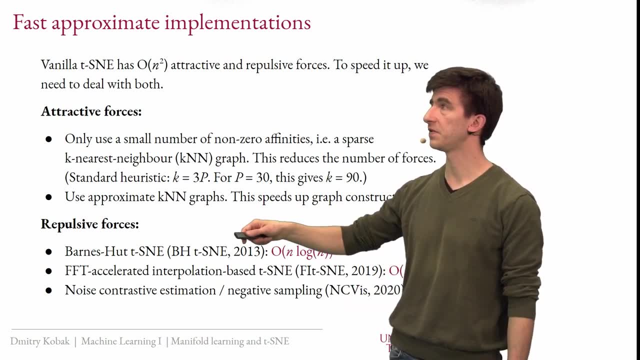 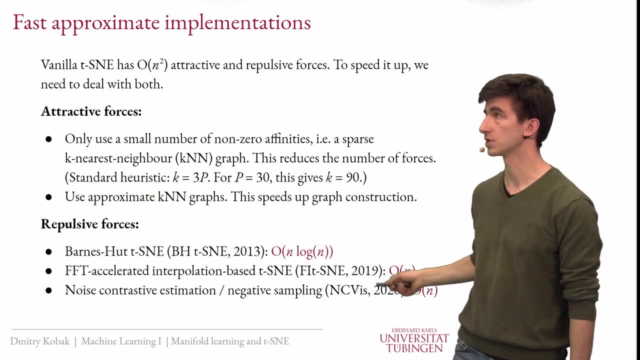 different ways to do that, with recent ones having actually linear complexity. i don't have time to explain what this does. i will very briefly explain you what barnes-hart does, even though you shouldn't use barnes-hart anymore now because there are methods that are much faster. 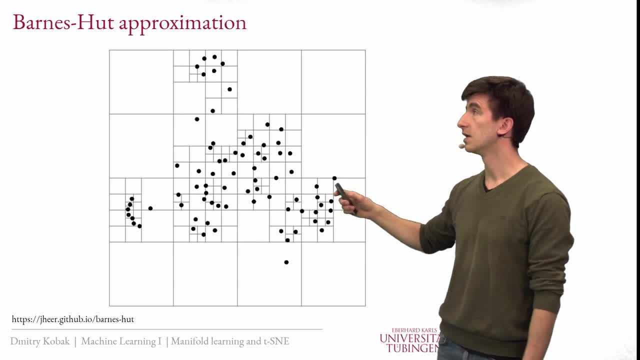 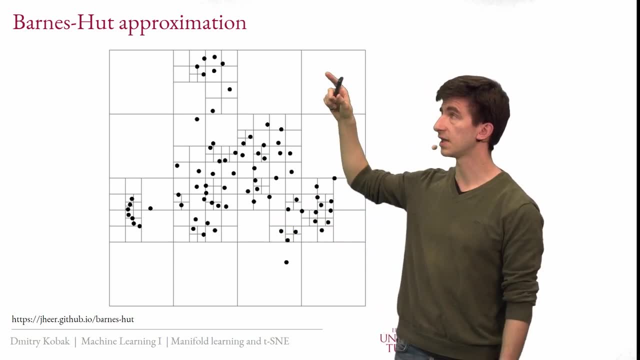 but it's slightly easier to explain. so i will, on this slide, try to give you just the gist of what's happening here. so imagine these are your points and i i should say that the technique, this barnes-hart method, was developed in physics, in computational physics, to solve the problems of 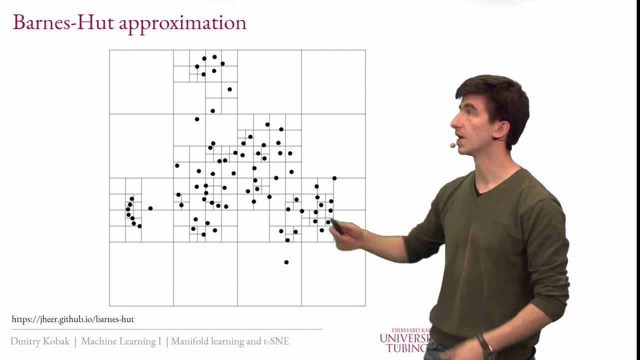 of many bodies, simulations and can be just used here. so you have points arranged like that. you construct this partitioning of the space so that the dense regions are partitioned finer and the sparse regions are partitioned um coarser, so to say. and then, if you need to compute, 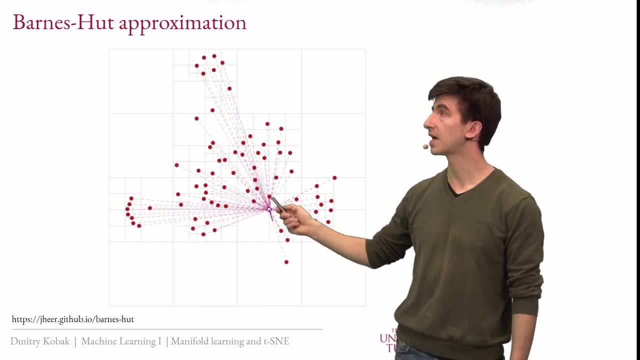 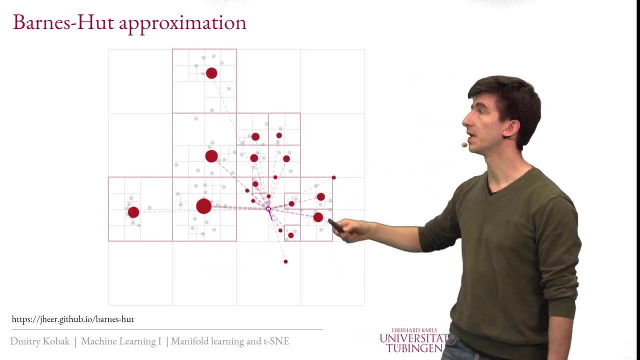 so, after this is constructed, if you need to compute the sum of the repulsive forces that this point, for example, feels so for it's pointing down here, uh, let's say we can, instead of computing the sum over all these points, we can coarse grain it and say for this: 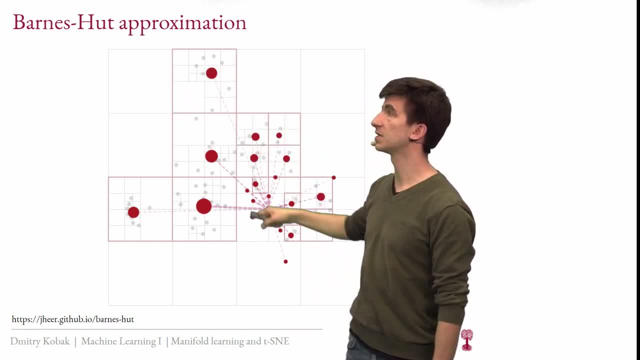 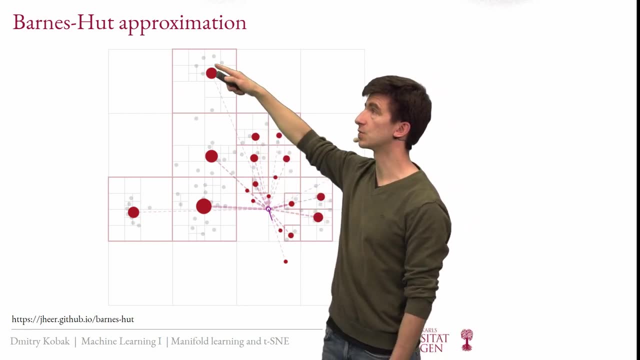 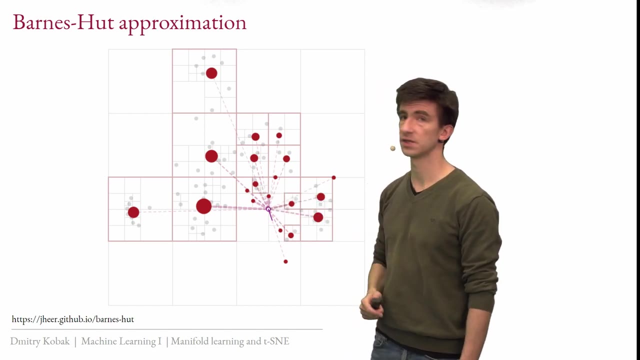 for these, uh, all points over here. the repulsion that this point feels is roughly, the repulsion that it would feel if it were one heavy point. okay, so we're computing just one term over here. but the closer you get to this point, the the more fine-grained um, you, um, you, you. group. 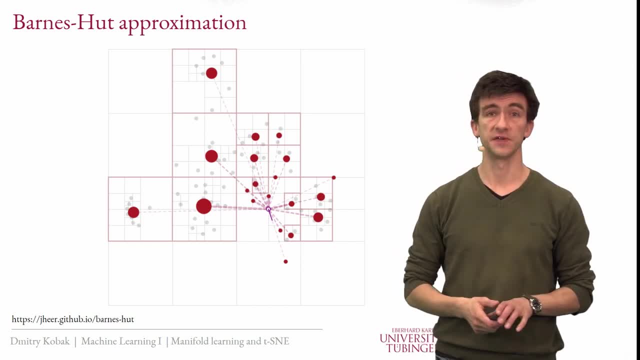 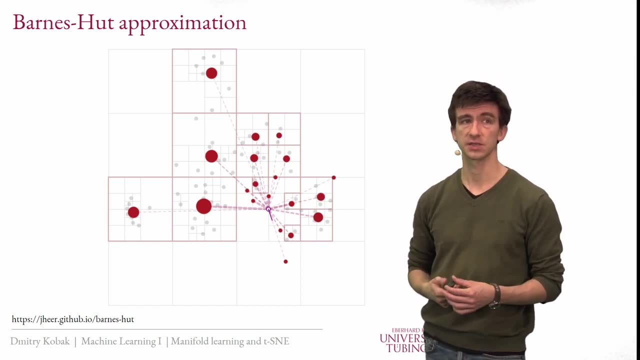 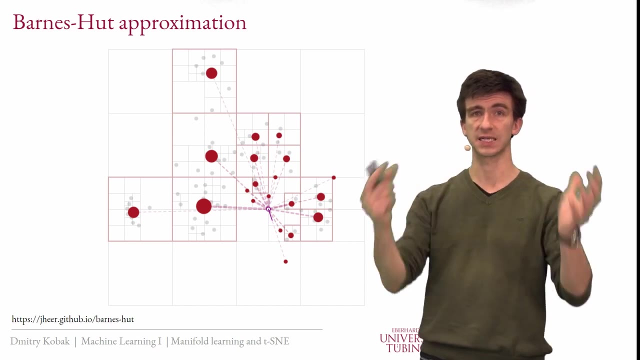 these points. so this allows this can be effectively implemented- uh, efficiently, sorry, implemented- and can work pretty fast. and allows one to actually embed things like amnest, even though, as i said, there are even faster approximations. but that's the general idea. you somehow approximate the sum of the repulsive forces that each point is feeling okay, great. so 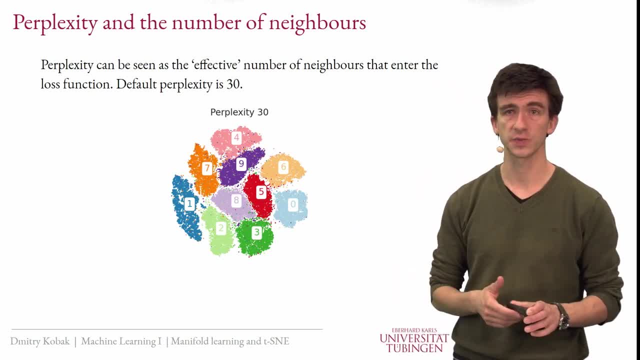 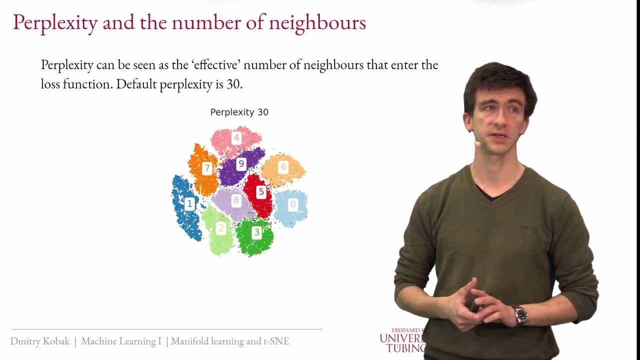 with this. i'm done with technical part. i explain you how to optimize the loss function, explain you the loss function itself. and now let's see how to optimize the loss function itself. and now let's discuss various parameters that there are in t-snear and what they do with the embeddings. 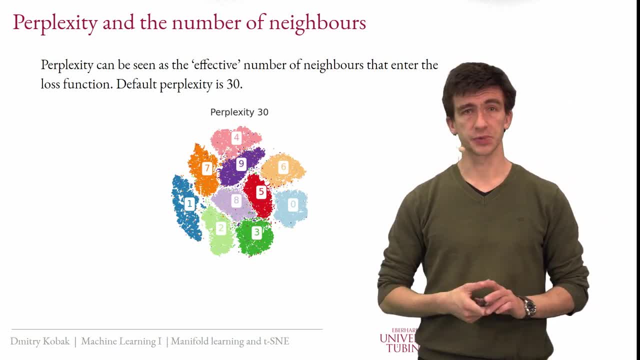 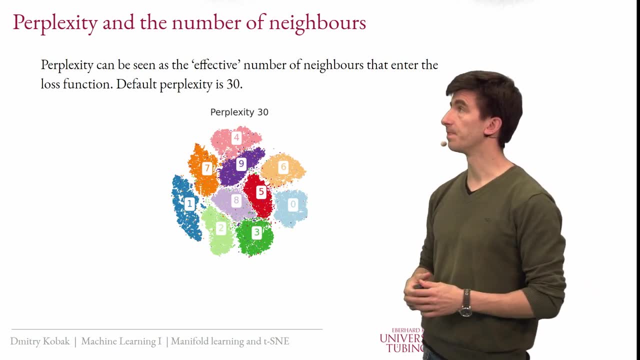 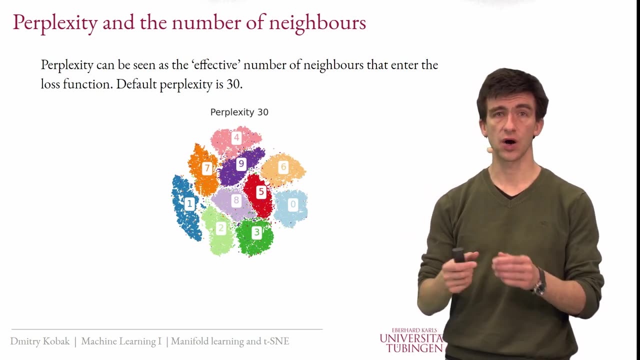 so i think, traditionally most people think that perplexity is basically the parameter that one can adjust in t-snear. so again, that's the. essentially the k regulates the k in the canine graph. so how many neighbors each point is feeling attraction to? and this is again the same image of amnest with perplexity. it's the launcher, etc. there are some functions that we're looking at, making every point with rozum, and so how many neighbors each point is feeling attraction to. and this is again the same image of amnest with perplexity. so and so shows you. also, if you have a thank you toadamente, which is actually a chainsaw, and the test 저기, is okay, but the answer to how you feasible is user signhy and that's for sure. in addition to you actually touch down here is, uh, not the intervals on the gray line of boundaries, so you can adjust this. 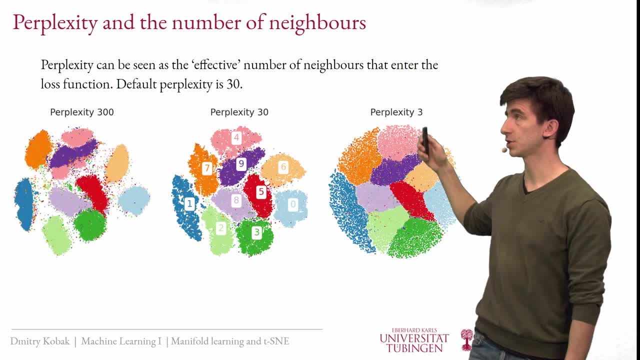 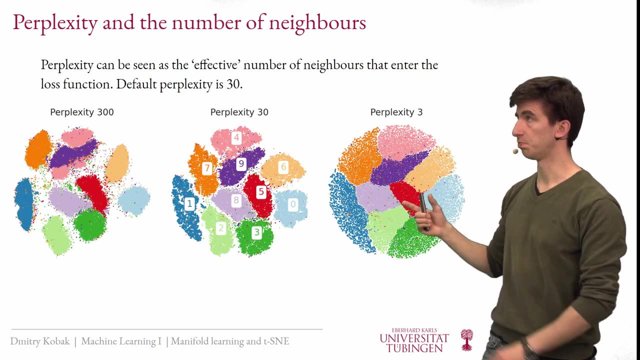 MNIST with perplexity 30.. So let me just show you what happens with much lower perplexity and much higher perplexity. And what happens is that there's less attractive forces around here. So this thing like inflates more and looks a bit like soap bubbles, I think. 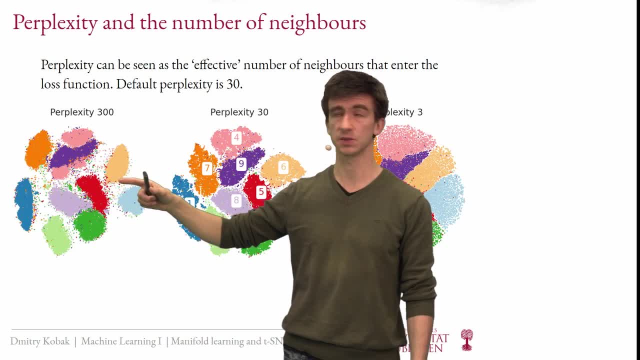 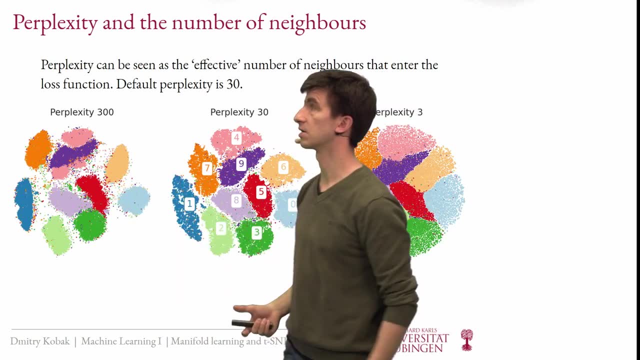 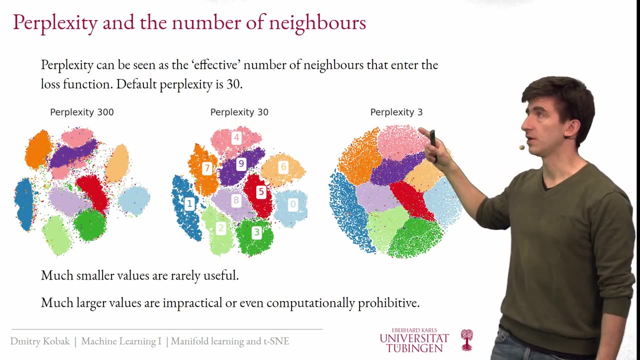 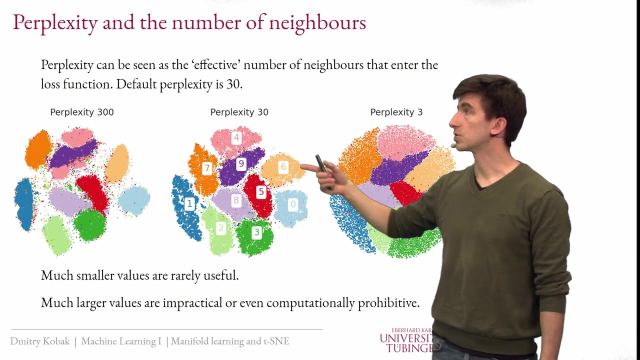 And here you have more attractive forces between more distance points. So what happens is that larger clusters, so to say, collect closer together in the embedding. But the thing is that very small values are rarely useful. Usually it looks like that and it's not very useful. 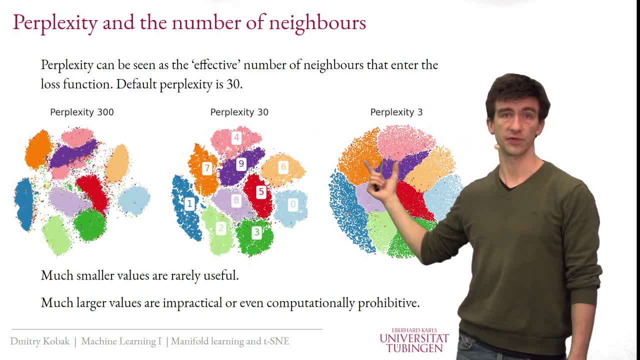 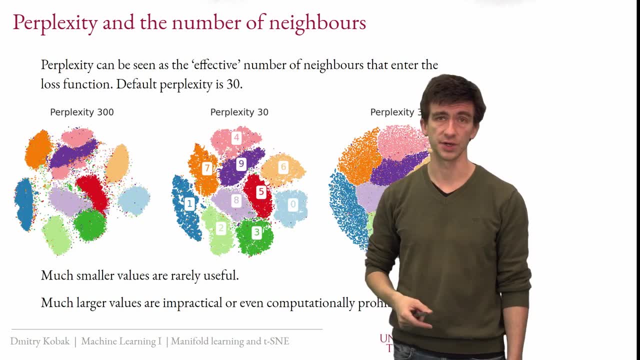 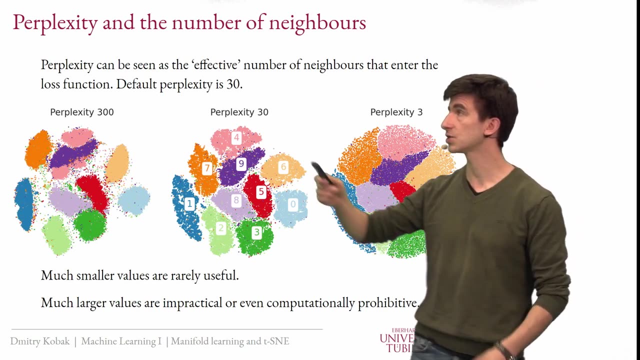 So to use a perplexity that is much smaller than 30 in order of magnitude is almost never useful, And to use a perplexity that is much larger Than 30 is almost always impractical or even completely prohibitive computationally, Because the larger the number of neighbors that you want to keep track of, the more attractive. 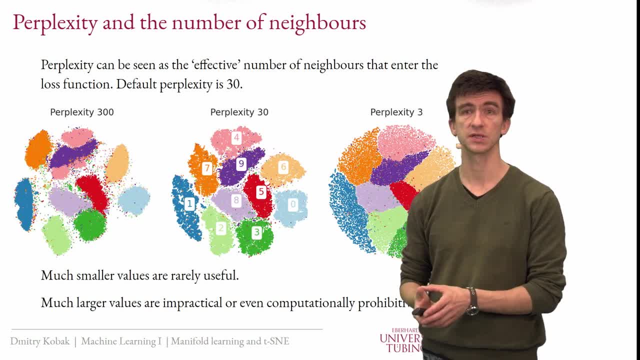 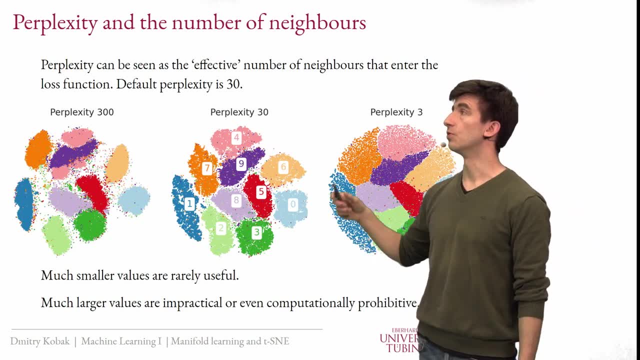 forces you have to deal with. So if you have a data set of million points and you want a perplexity of 100,000, this will just not work. This will not fit the memory and it will never converge. So if you have a large enough data set, then you're basically stuck. 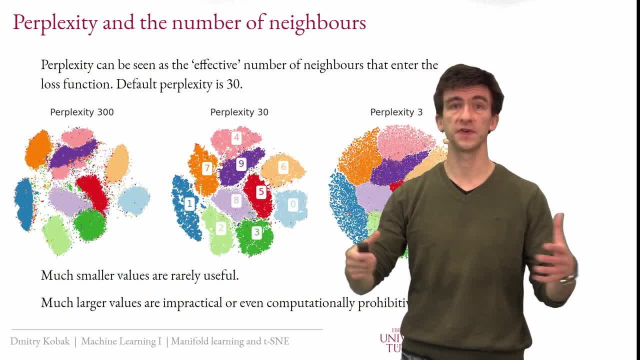 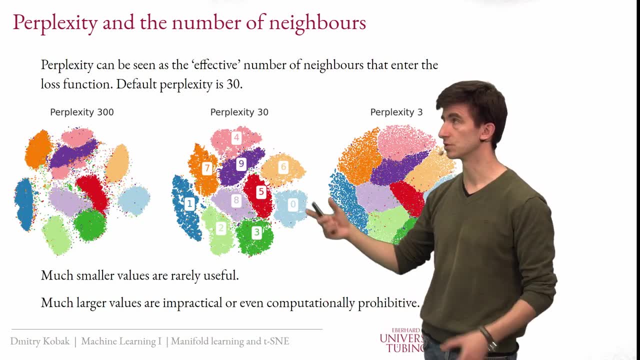 Then you're basically stuck. Then you're stuck. You're using perplexity of 30 or 50 or 100, but this doesn't make any difference for large data set, but you cannot increase it enough to start seeing something qualitatively different. 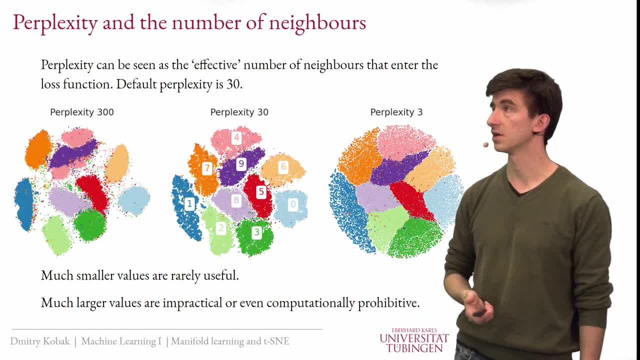 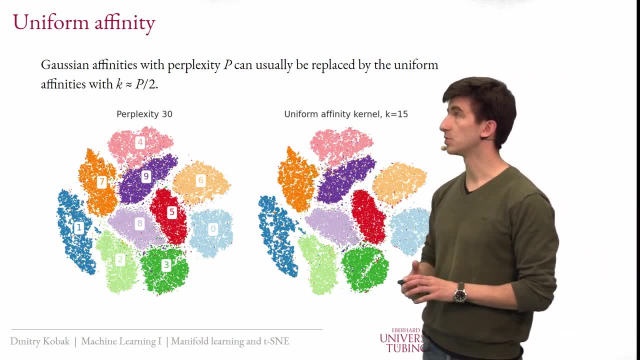 So, in fact, in most practical cases, perplexity is not a parameter that you can meaningfully vary, at least in my experience. That's one thing that I promised to show you about the affinities. So this is again the default T-SNE, with perplexity 30.. 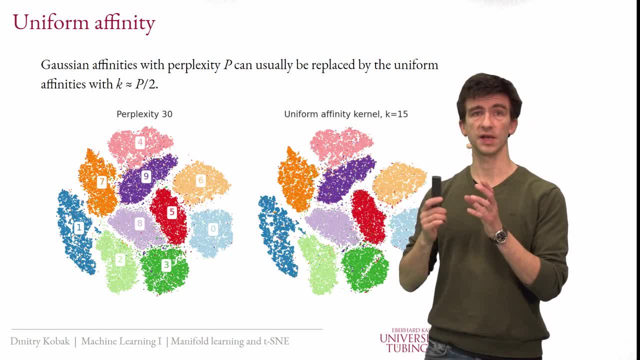 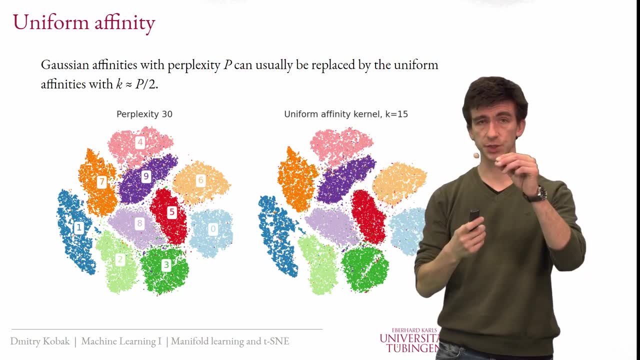 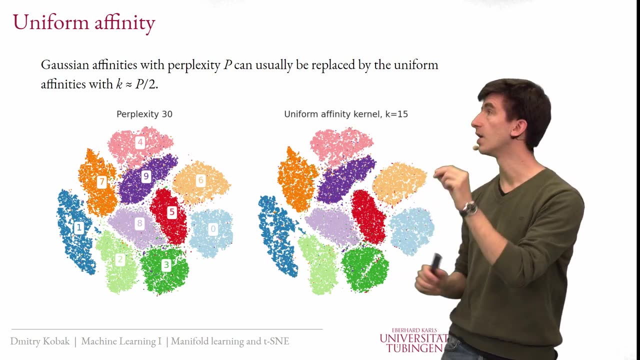 And this T-SNE I made, made with uniform affinity in the high dimensional space with 15 neighbors. So each point for each point I find 15 nearest neighbors and it has the same affinity values to all 15.. And you have to look very, very closely to spot any difference here And even to make 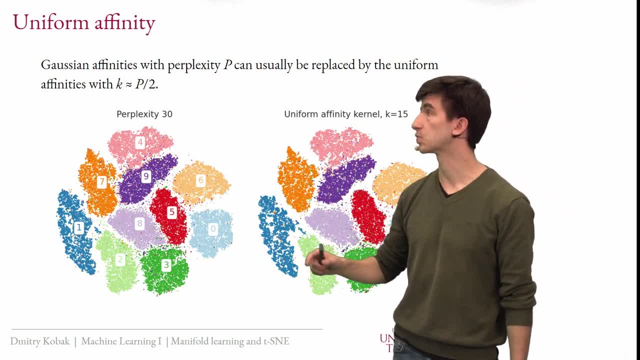 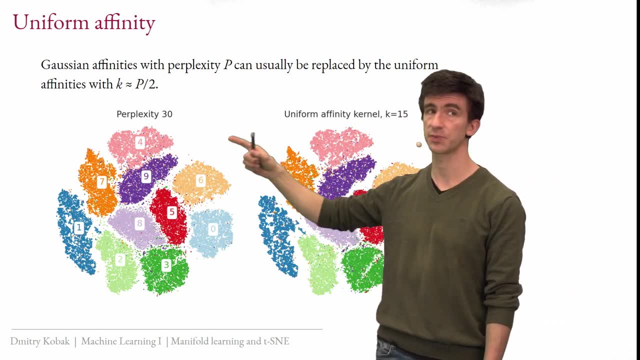 sure that I didn't by mistake. I'm not showing you the same picture twice, but look, for example, this yellow cluster looks a little bit different. So it is not the same picture, but it's very similar. And you can take perplexity 300 and the uniform similarities with K150 and they 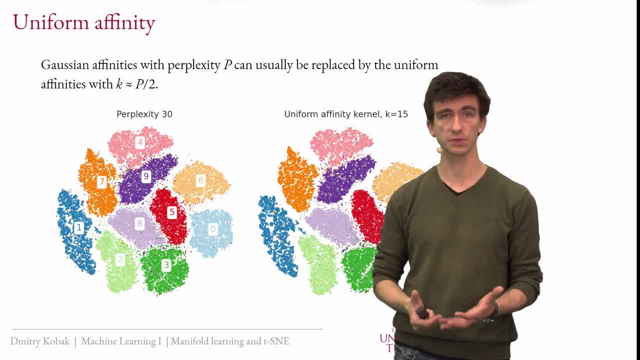 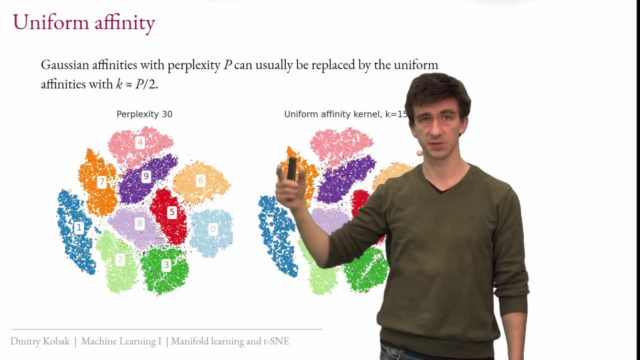 will again look very similar. So it doesn't have to hold mathematically. but in practice. for most data sets it holds very well. So these entire Gaussian affinities in the high dimensional space, this is actually not important. You can just take uniform affinities with. 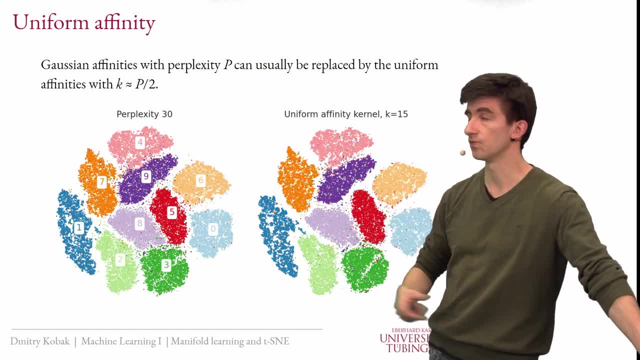 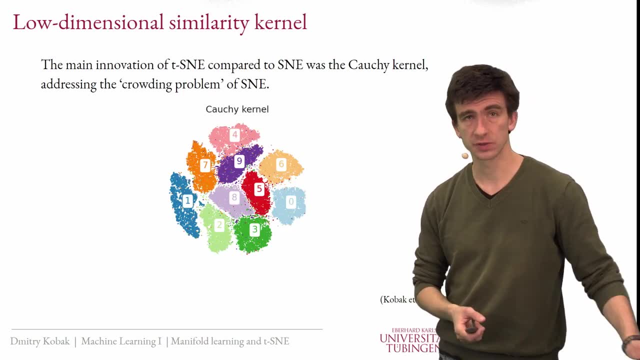 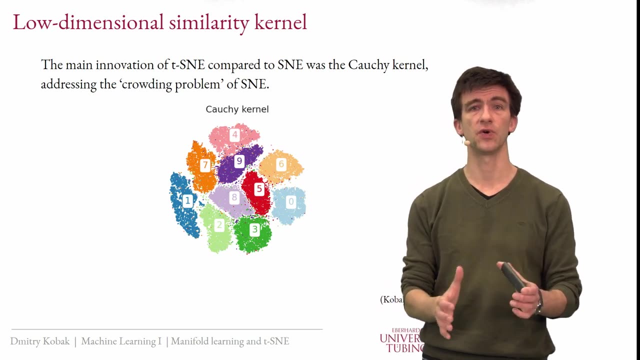 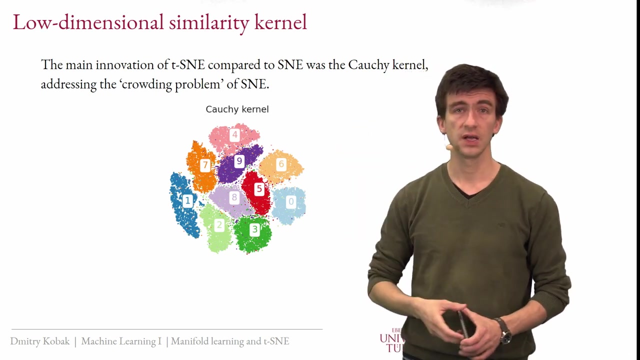 15 nearest neighbors and the rest Just works the same way. Okay, Another important thing is what happens in low dimensional embedding with the similarity kernel. I mentioned before that SNE original paper used Gaussian kernel and the TSNE used Cauchy kernel And the TSNE paper made a big deal out of that. They said 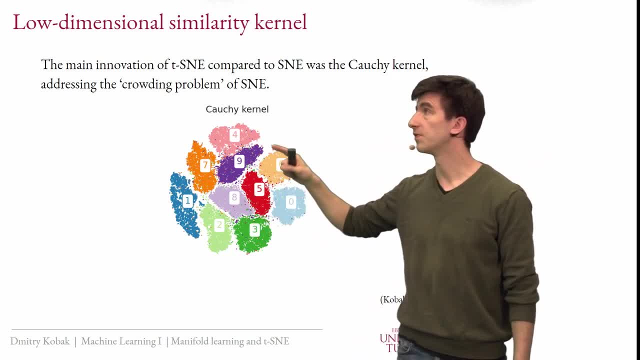 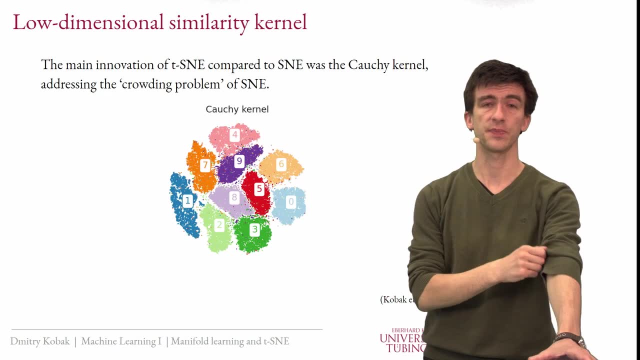 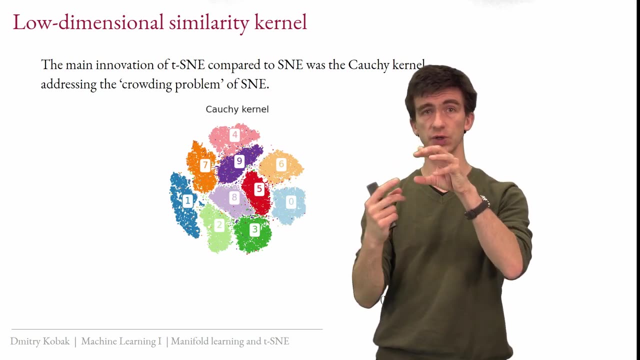 that they are addressing something they call crowding problem, And the intuition that they present in the 2008 paper is that sometimes the embedding one, like the TSNE loss function, wants to preserve, for example, I don't know- 15 nearest. 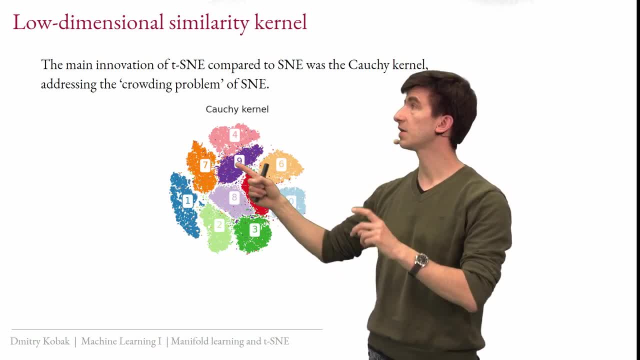 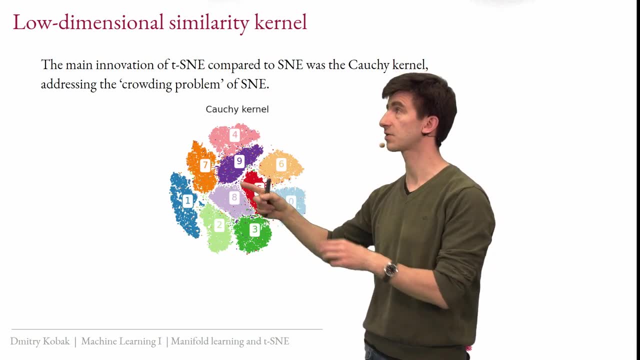 neighbors of a particular point. but there is not enough space, so to say, in a two dimensional space, to keep all these points closer. So you have to make some sacrifice and put some of the nearest neighbors a bit further away, And if the kernel is Gaussian, then you will. 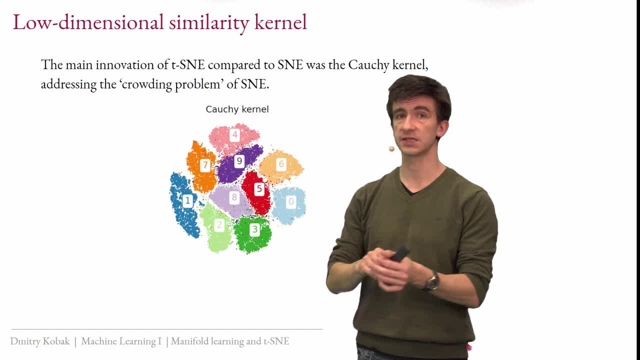 pay a high price for that. So the argument is: let's take a kernel that decays slower, so a heavier tailed kernel than Gaussian, and then maybe some of the nearest neighbors can be allowed to move a little bit further away, but the Q value will still not. it will. 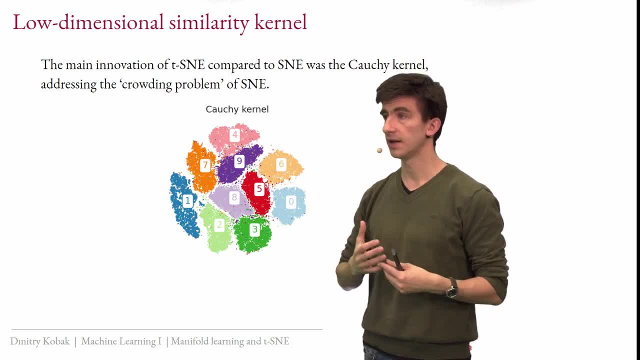 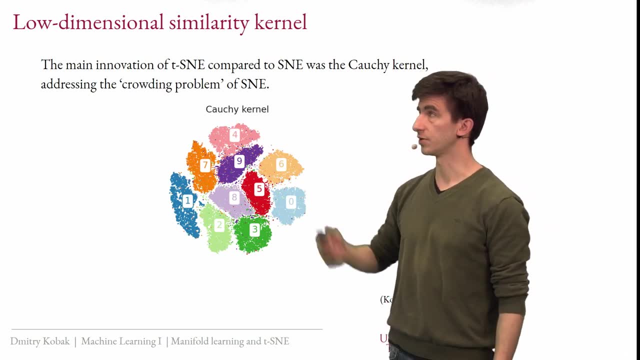 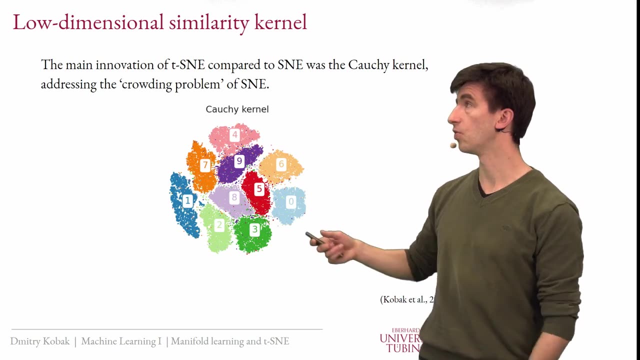 not go down by that a lot. Okay, So the heavy tailed kernel is more permissive, so to say, in a sense, and so the crowding problem is addressed or solved. So the funny thing is that the original paper doesn't actually show, for example, the SNE of the entire MNIST. 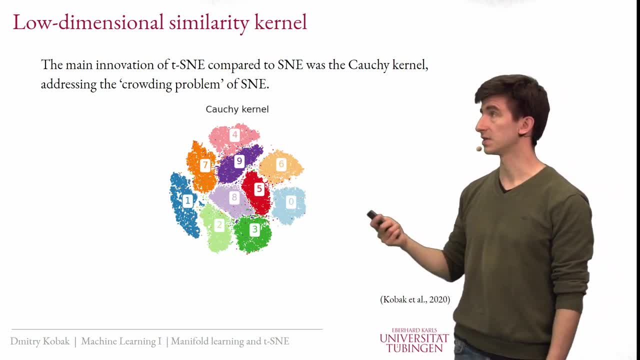 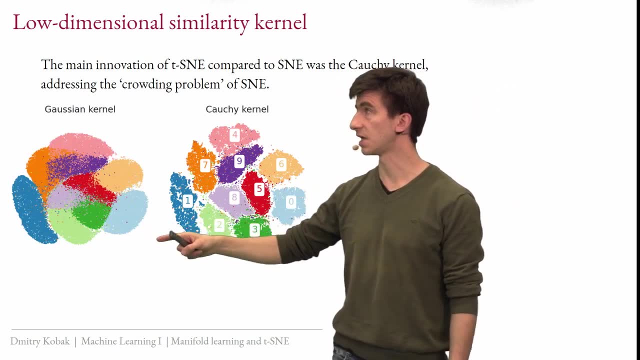 and it wasn't until recently that we implemented that in modern TSNE implementation to see what happens. and here's what happens. So this is the SNE result on the entire MNIST and this is the TSNE result: the Gaussian kernel, Cauchy kernel, So what you see here. 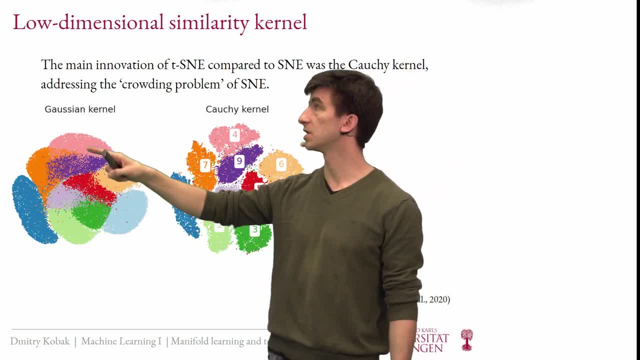 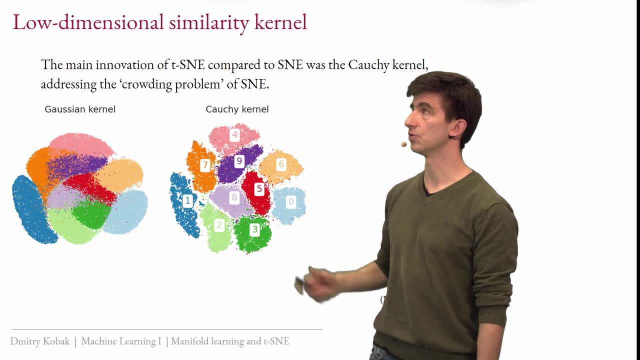 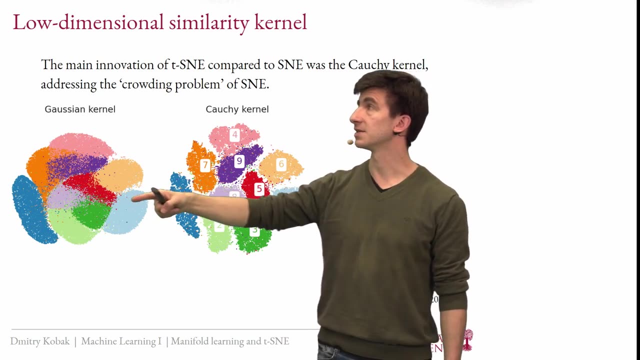 is the crowding problem And, in a sense, yeah, there is some overlap between clusters and there's very little, no white space in between the different clusters, and that's something you get with TSNE. Funny thing or interesting thing is that one can think of that as a family. 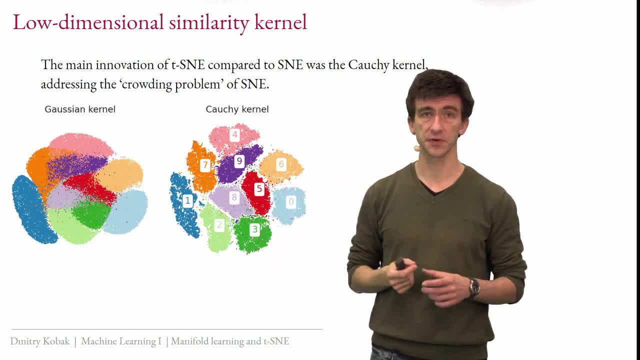 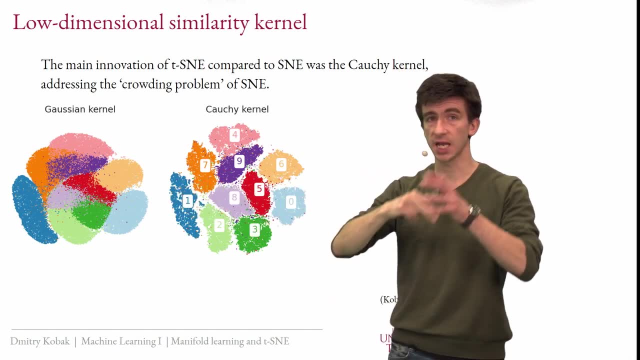 of kernels where this is a t-distribution with infinite degree of freedom, if you know that from your statistics classes and this is a t-distribution with one degree of freedom, and one can vary the shape of this kernel, making it more or 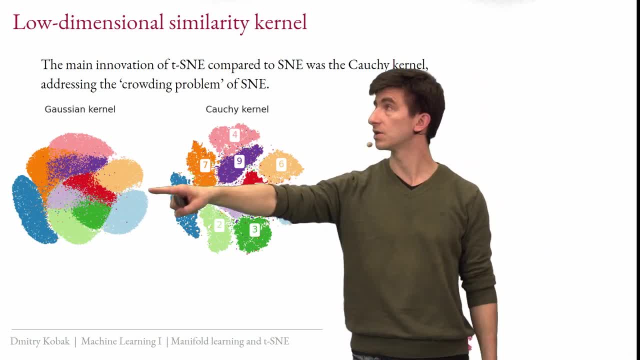 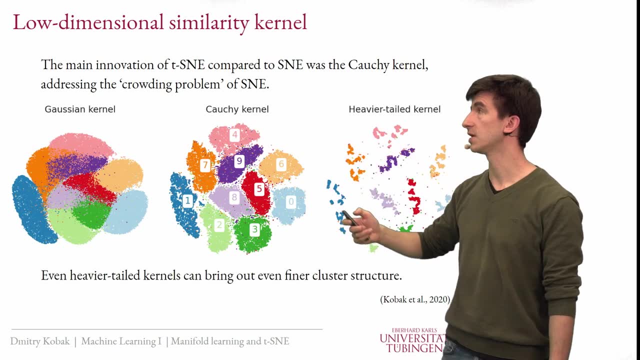 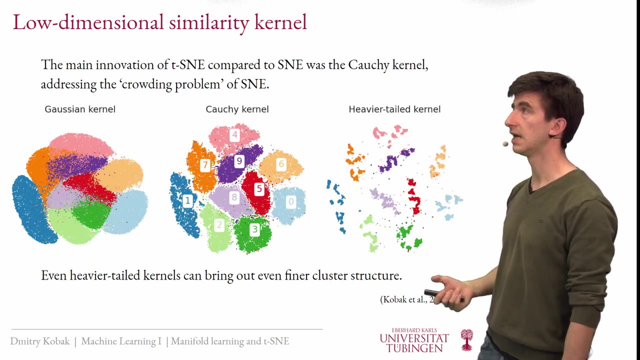 less heavier tailed and see what happens with embedding. So here you move, like imagine moving from this embedding here, but one can make it even more heavier tailed And if you do that you get a picture like that. So this is using even heavier tailed kernel than the Cauchy kernel. 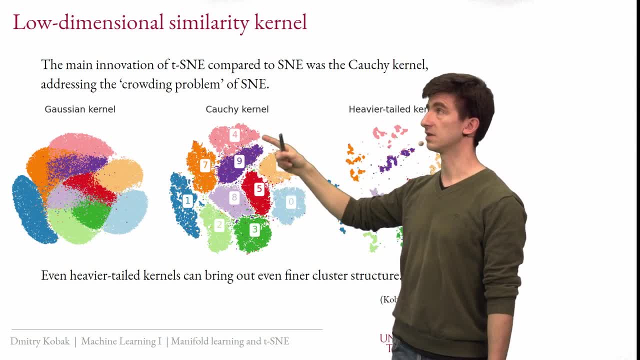 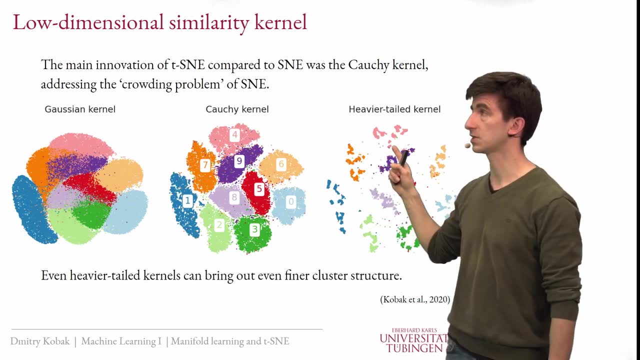 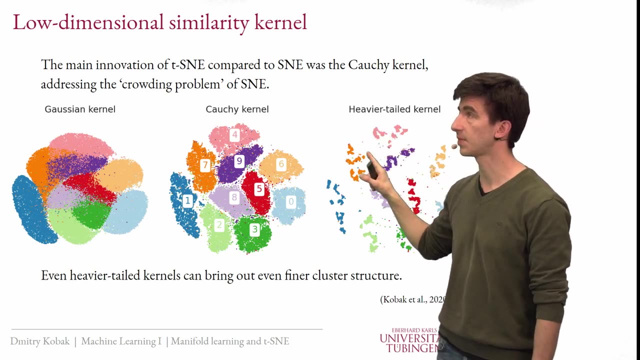 And an interesting thing happens in that each digit splits into more fine clusters, So you'll see finer cluster structure And the interesting thing is that you can. if you look at what images form this cluster, then you see that at least in some cases that's meaningful islands. 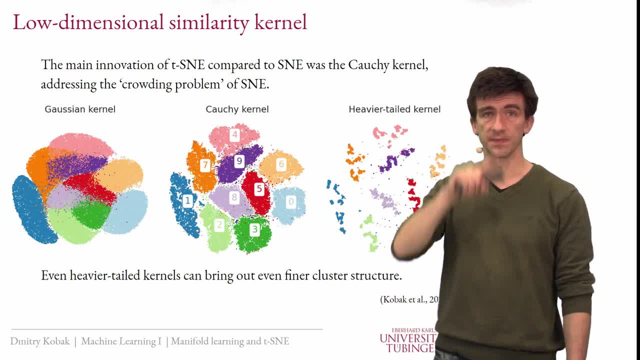 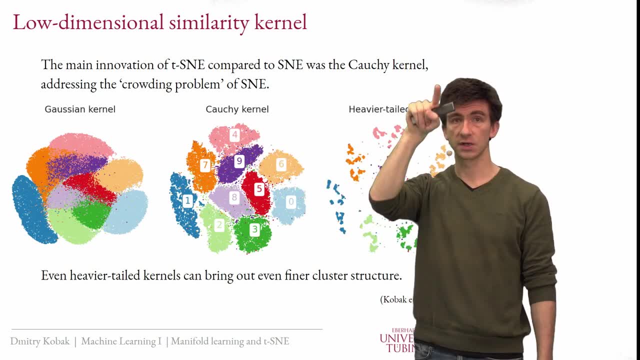 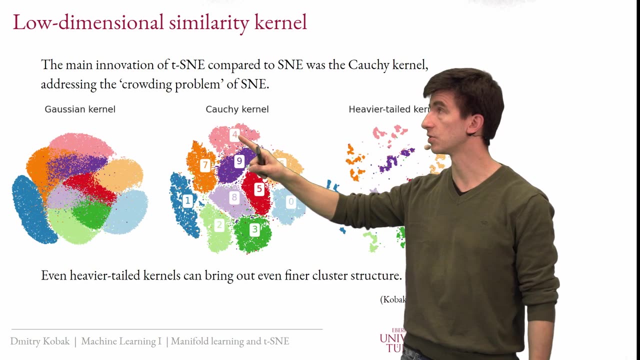 So, for example, the four can be written like that: open on top, or it can be written as it's printed over here, when it looks like that: Okay, and some people write four open on top and some people write four closed on top. 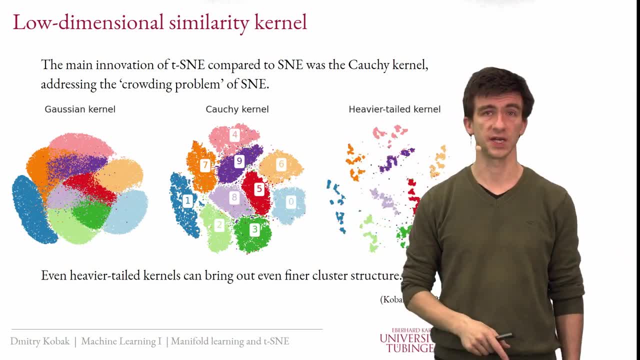 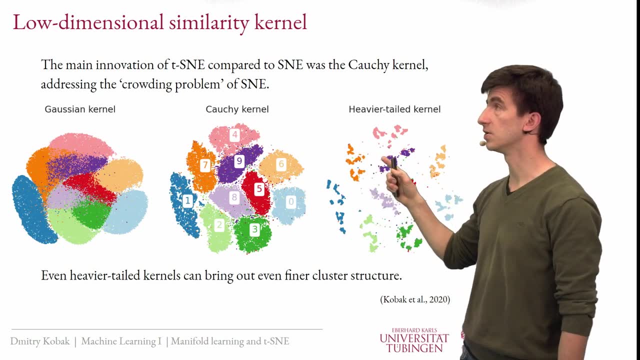 And you'll see that one of these islands corresponds to one of the handwritings and the other islands correspond to other kind of handwritings. So you can, one can actually show that at least some of these islands are meaningful, and one can show the same on other data sets. 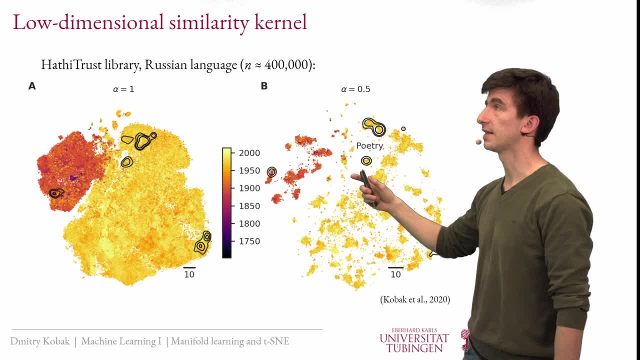 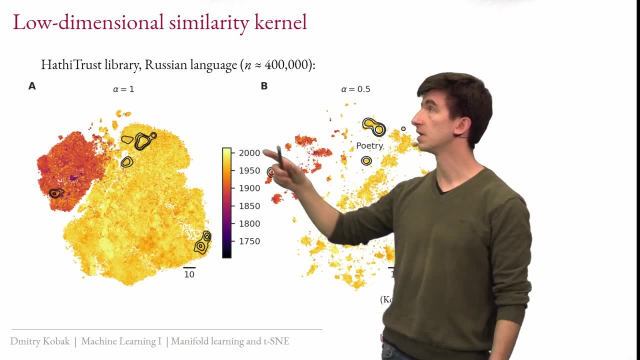 So that's something I find even more remarkable. So here's, for example, analysis of the same library data set that I mentioned in the beginning, but a subset of it of Russian language. So there's half a million 400,000 points over here, colored by the: 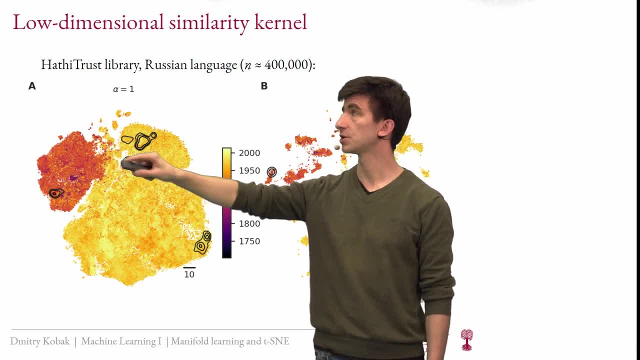 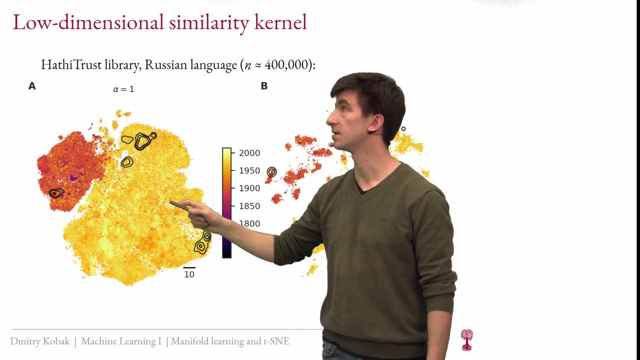 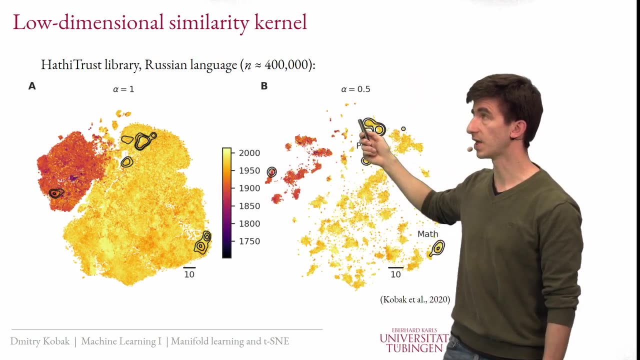 by the year when the book was printed, the Russian language changed, changed orthography in after the revolution. That's why all pre-1917 books are there and later books are over here. But the interesting thing is that you decrease the. 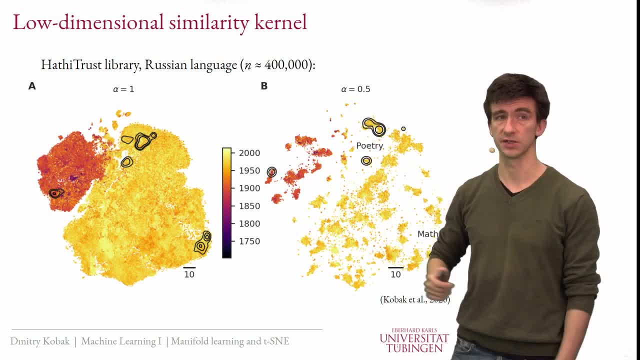 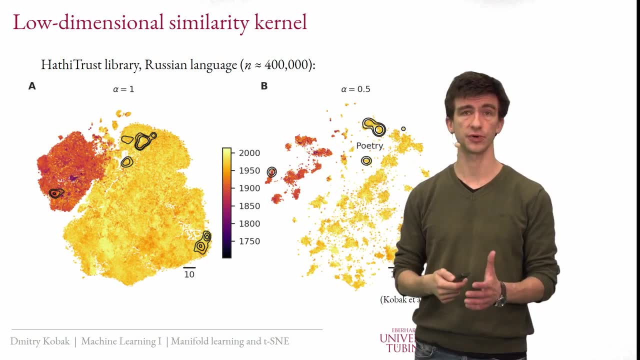 this parameter, you increase, you make the kernel more heavy-tailed. Over here you get all these islands. Are they meaningful, or are they not meaningful? Well, we can find, for example, all the poetry books, and it turns out that the poetry books are all over here. 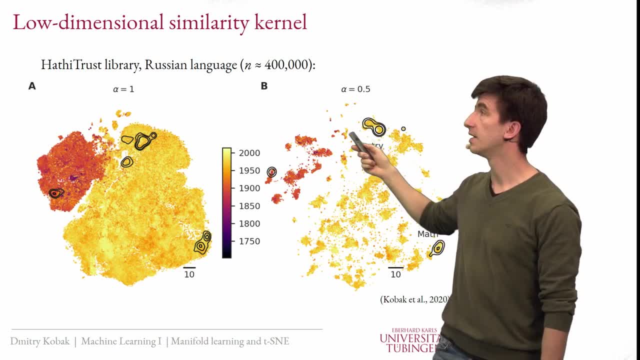 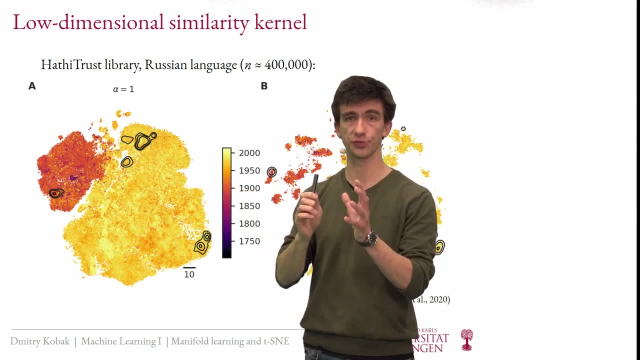 So this island is the poetry island. It makes a lot of sense Here. all the poetry books are also together. So t-SNE does like a default. t-SNE does group them all together, but it doesn't separate them from the rest visually. 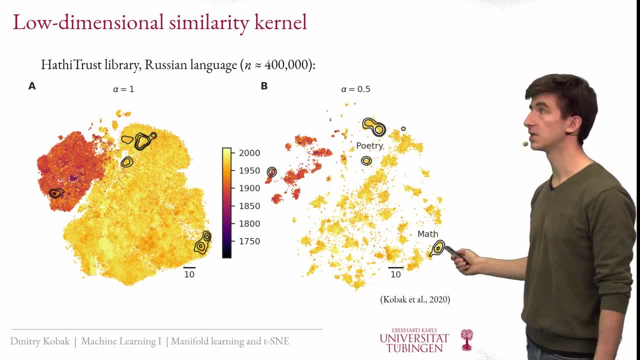 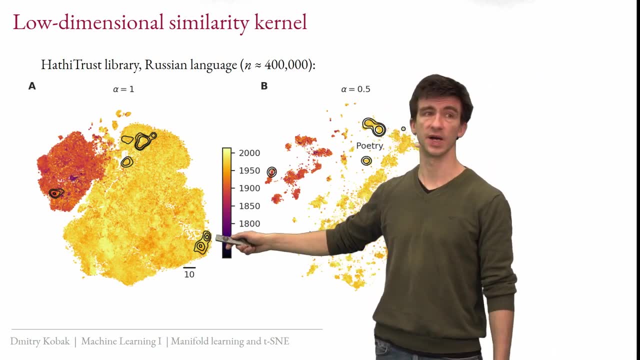 And all the math books that you can also just find by keywords are concentrated in this island. So this is the math island and here all these books are in this corner. But if you didn't know that these are math books, you would not suspect that this is something separate. 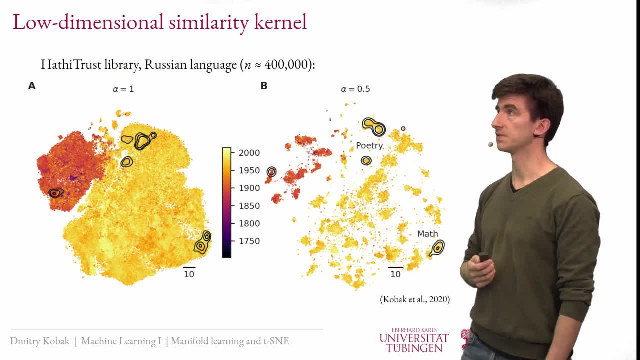 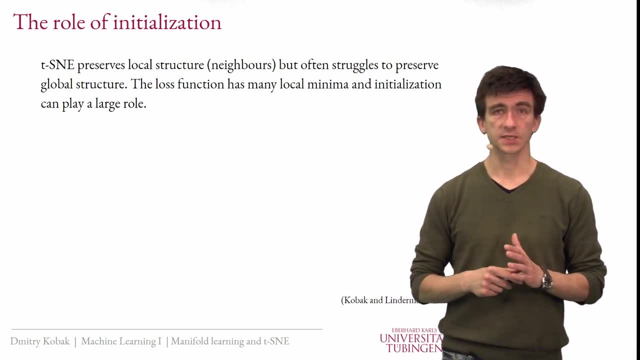 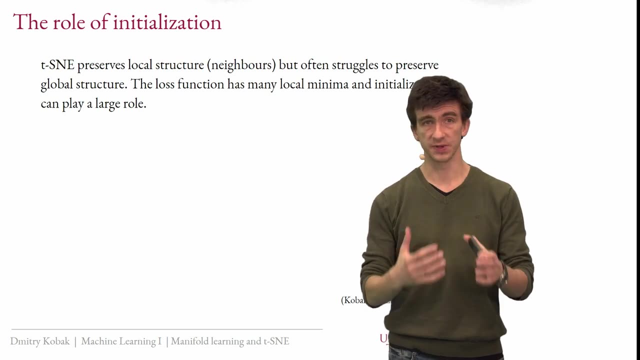 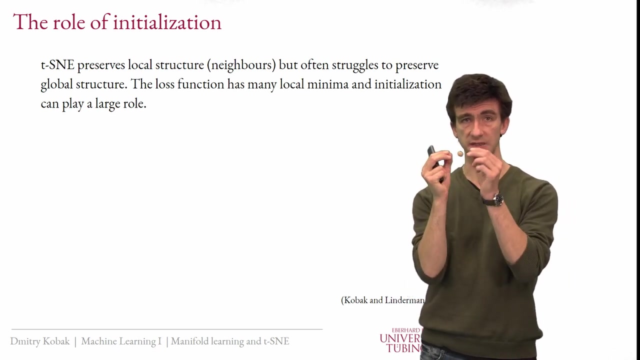 So what happens here is the heavier-tailed kernel. emphasize this fine cluster structure. Something else I said before that t-SNE preserves, like the loss function of t-SNE explicitly, is constructed to preserve local structure of the data If points are neighbors, nearest neighbors. 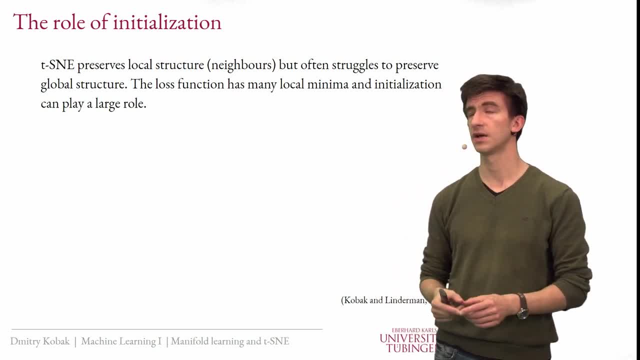 then t-SNE try to keep them as nearest neighbors in the embedding. At the same time, t-SNE will often struggle to preserve global structure of the data. Another way to formulate that is: you do the gradient descent, You start from some initialization. 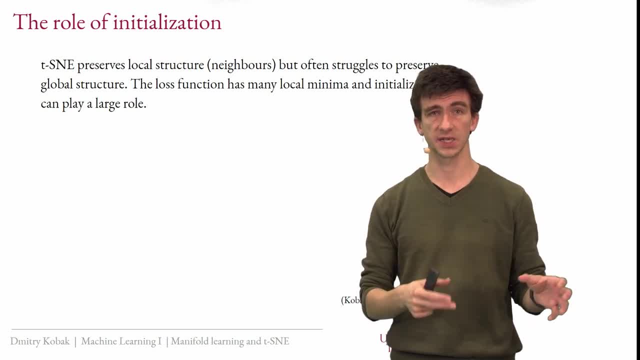 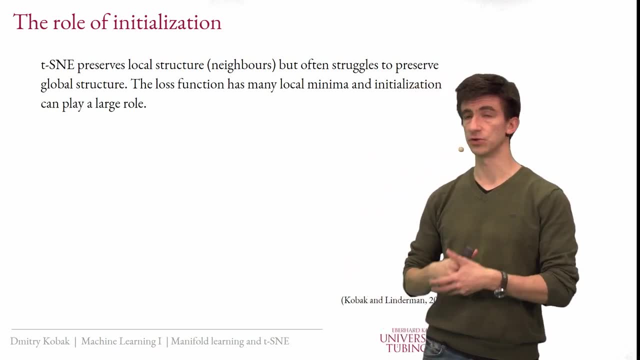 but actually the loss function has many local minima and sometimes they are bad local minima. I mentioned this before. Remember the first time I showed the MNIST animation it was stuck in the local minimum. We could solve that one by early exaggeration trick. 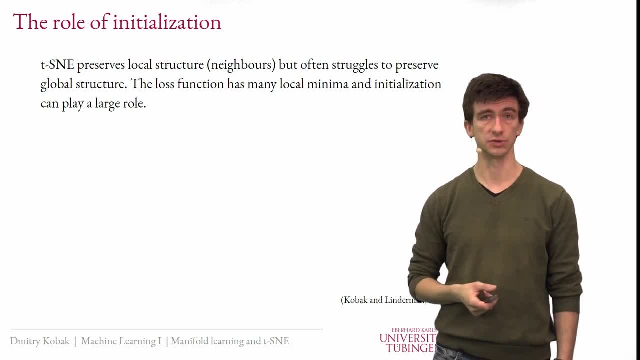 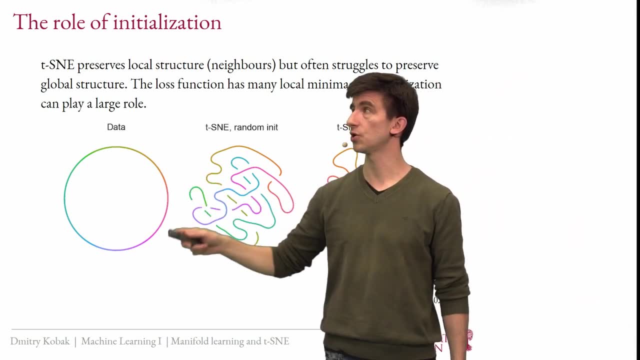 but in some cases the initialization will play a large role as well. And to show that I can use this very, very simple toy data set, where the data is just two-dimensional circle with some noise added, And then if we run t-SNE on this data, 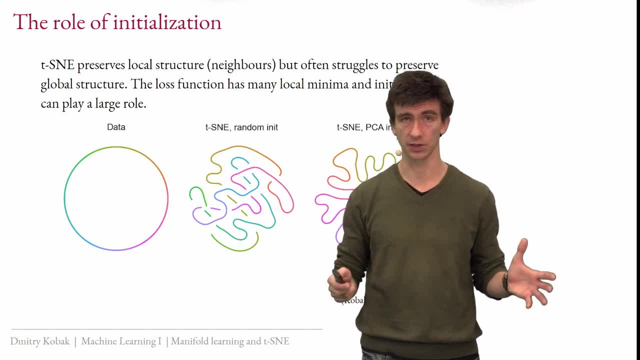 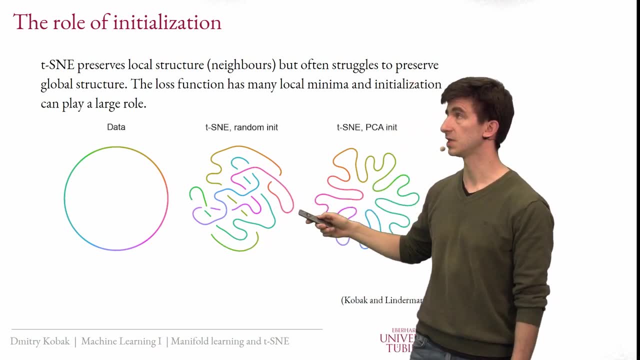 so we're taking two-dimensional data and embedding it in two dimensions. Of course this doesn't make a lot of sense, but just for the sake of this toy example, I can do that. So here's the default t-SNE with random initialization on this data. 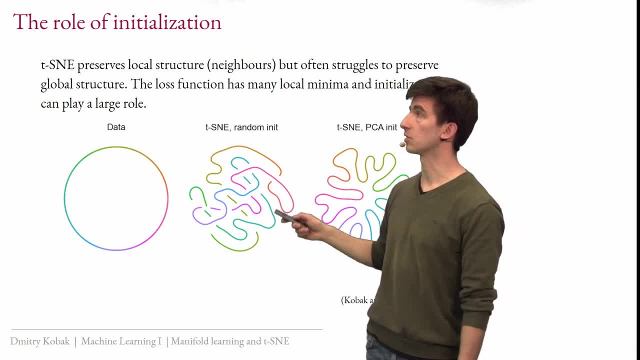 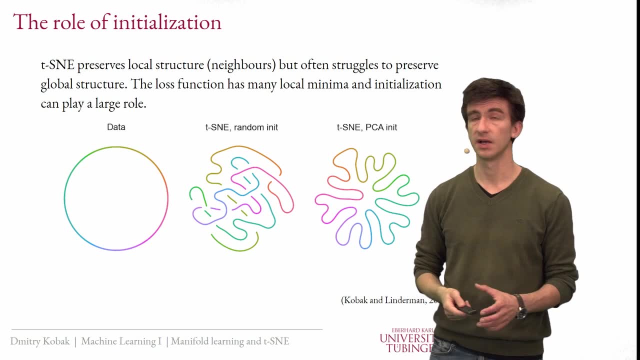 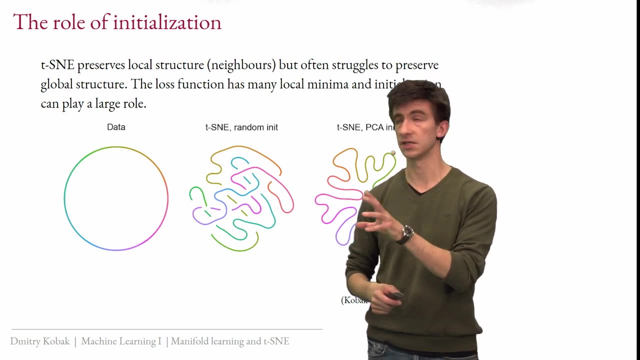 It's actually a nice picture. I think It looks like a knot, but clearly the global structure is messed up here. If you use PCA- the first two principal components of the data- to initialize t-SNE, in this case PCA just coincides with the entire data. 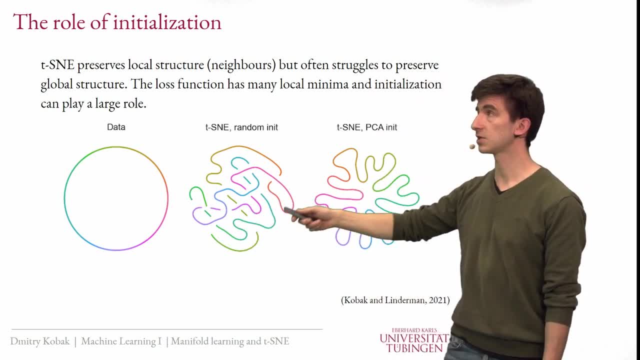 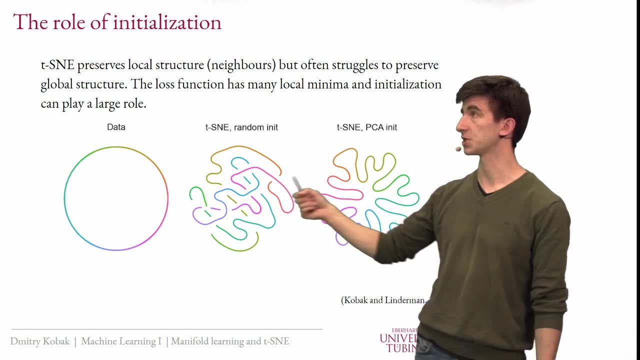 of course. then it will converge to something like that. So these are two end embeddings that the gradient descent converged to. So this is a local minimum of loss function and this also is a local minimum of loss function, But that's a bad local minimum. 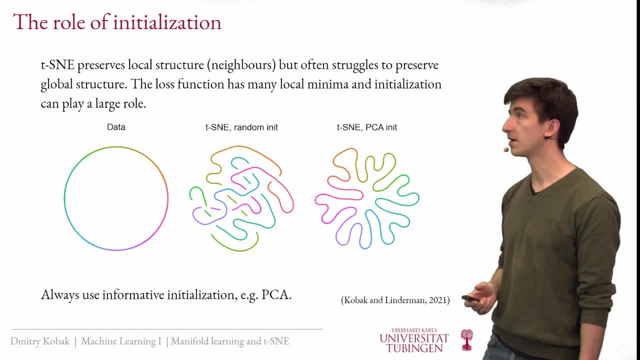 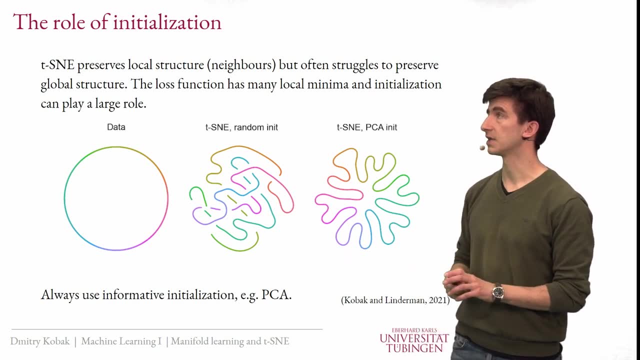 That's a better local minimum And I think the take-home message here is that it absolutely does make sense to use informative initialization, For example PCA. there are other choices, but for example, PCA to initialize the embedding. okay, Because why not? 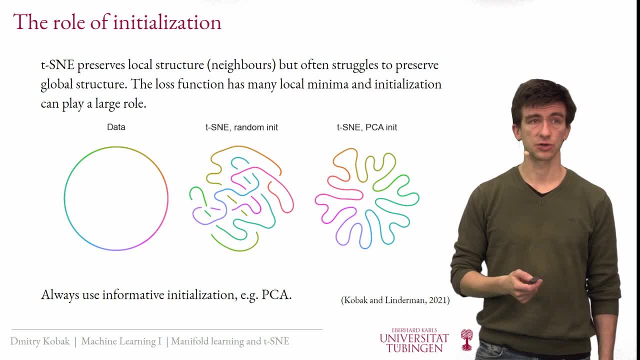 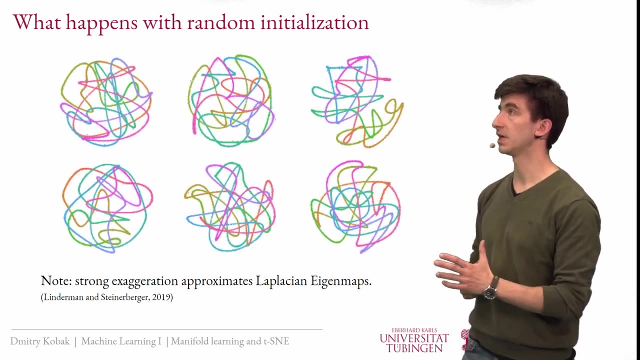 Then you will converge to a better local minimum. That's true not only for t-SNE but for any kind of neighbor embedding algorithm And yes, I have an animation that shows actually what happens if you optimize the circle data with six different random initializations. 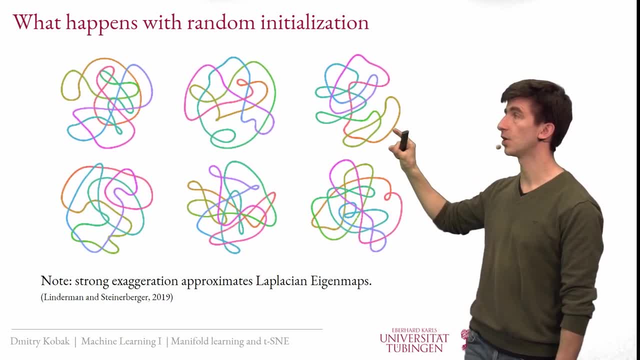 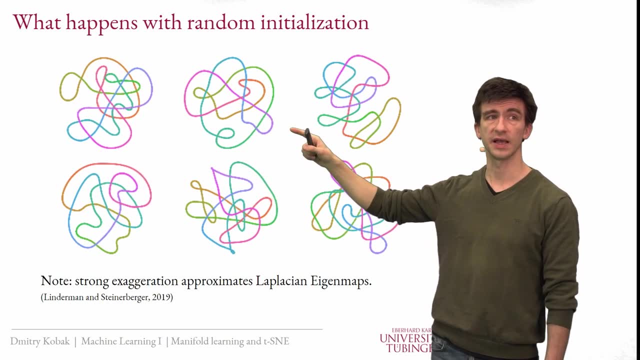 I think it's fun to watch because you can see very slowly how, during the early exaggeration phase, they are very slowly unwrapping. That's an interesting phenomenon, but very, very slowly. And then, once the early exaggeration is turned off, 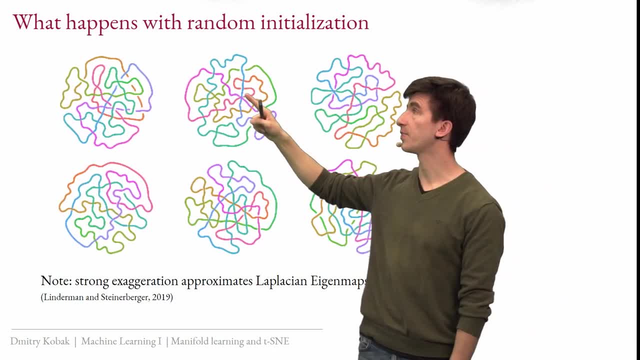 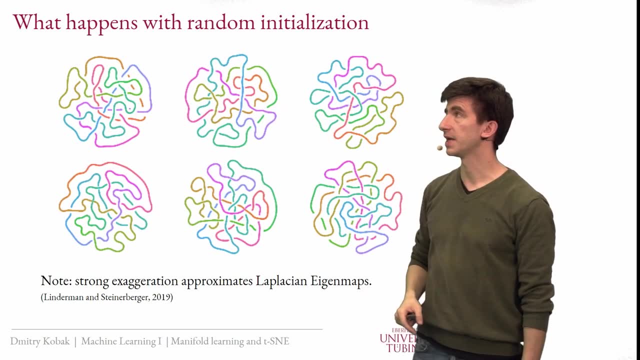 it will happen in a second. you will see that, yeah, they stop unwrapping and they make gaps. the overlapping parts make gaps because there's this repulsion that they feel And in the end you get this: six random knots. 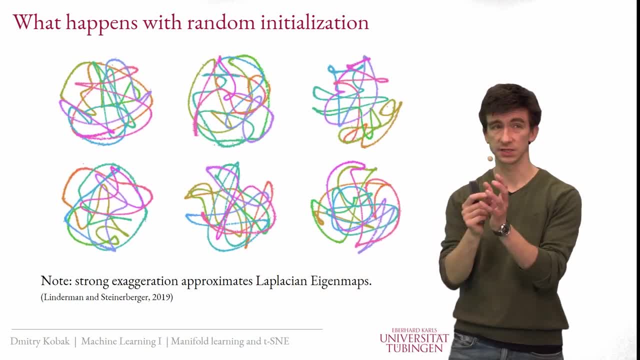 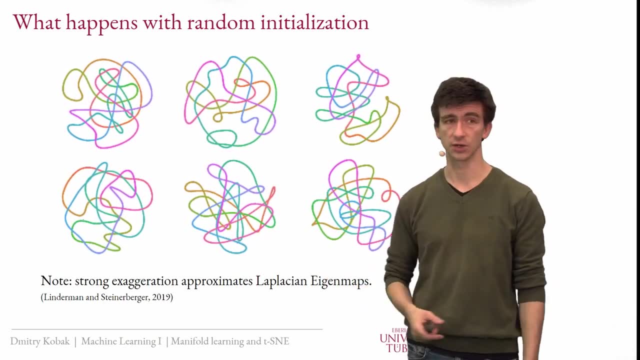 So interesting thing happened during early exaggeration, where this is slow, unwrapping, because actually one can show that there is a mathematical relationship between strong early exaggeration and a technique called Laplace and Eigenmaps, which I don't have time to introduce properly today. 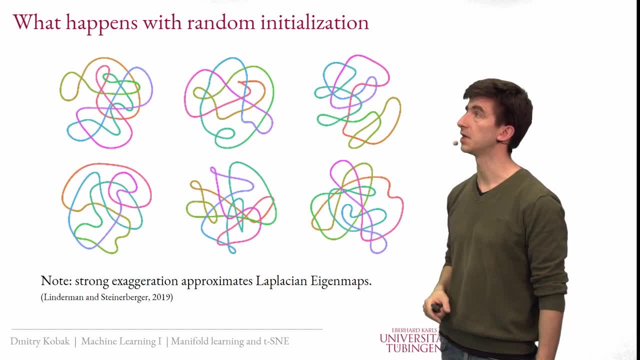 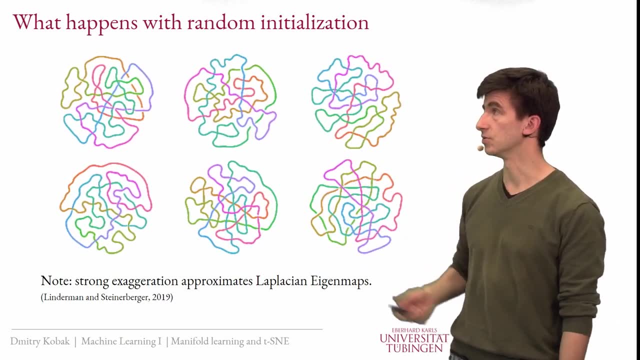 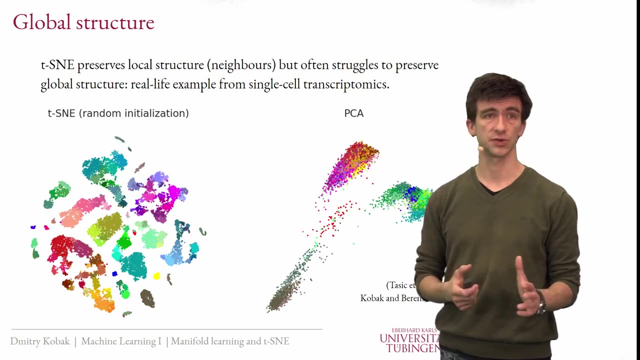 but that explains why it slowly unwraps but takes a long time to unwrap fully. So in this case you'll end up with the knots like that. And this doesn't only happen in this funny two-dimensional toy example, but let me show a real-world application. 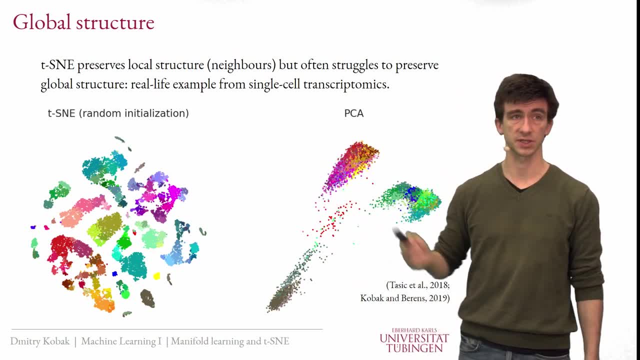 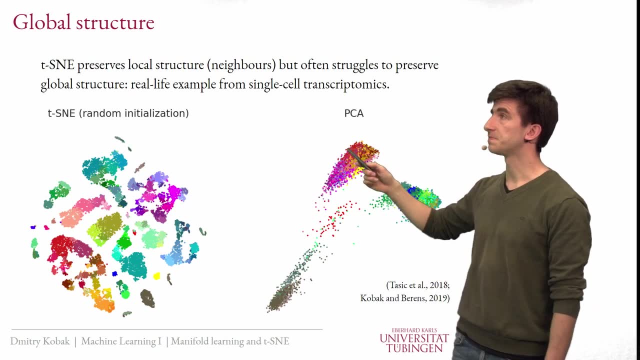 where the same thing happens. So this is a single set of cell transcriptomic data set where there's a lot of different clusters. That's the paper I take the data set from, But even though there's a lot and a lot and a lot of different clusters, 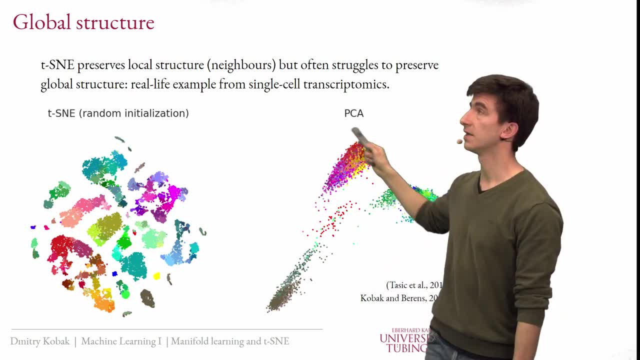 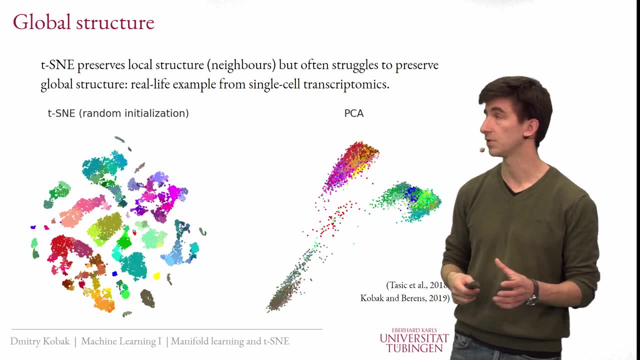 there are three very broad groups that you see here. In fact, these are inhibitory neurons, these are excitatory neurons and these are non-neural cells in the mouse cortex, But it doesn't matter for now. What matters is that if you do PCA of the data, 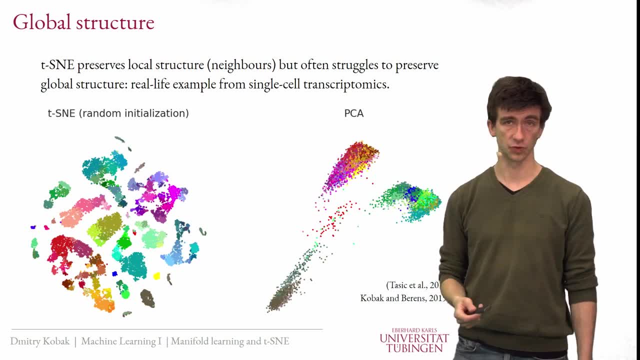 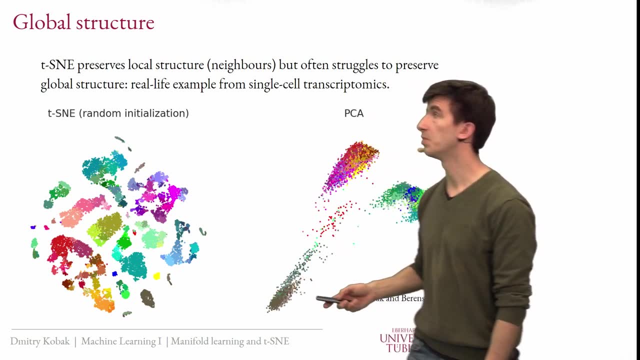 you immediately see that there are three very distinct groups, right. But if you do t-SNEAR, you see that maybe there's 100 of small islands in the data, clusters in the data, but all these cells, for example the gray-brown cells- 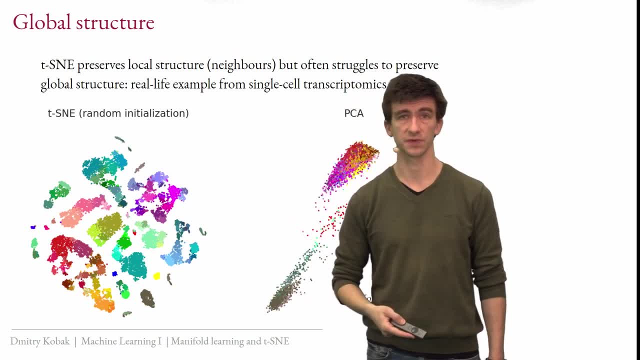 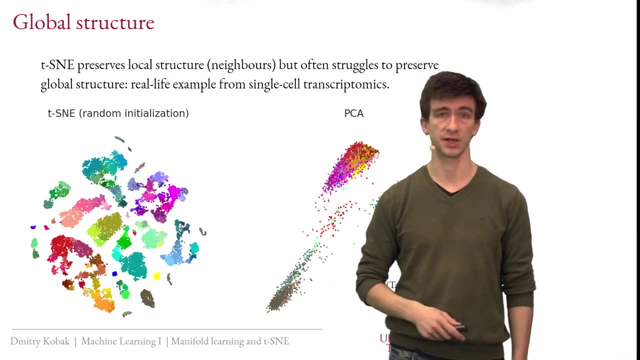 they form a bunch of different clusters and these clusters end up in different parts of the data. So I am using early exaggeration and everything else, as I should be doing here, and still it ends up like that, And that's because of the random initialization. 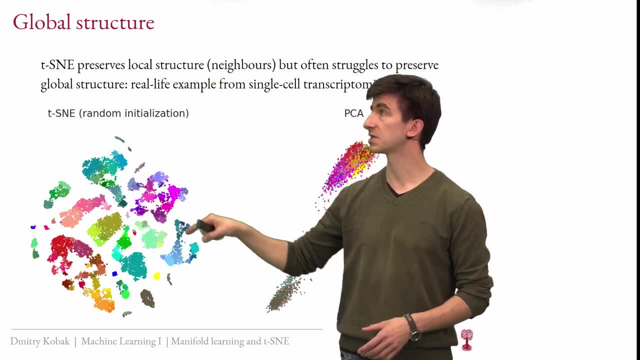 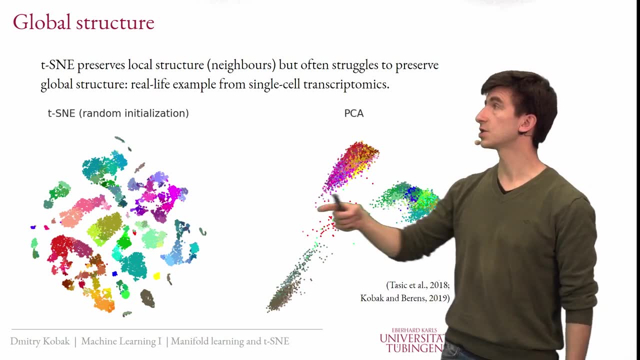 If I rerun with a different random initialization, I will see the same islands but positioned differently. So what one can do, as I already suggested, let's just initialize t-SNEAR with PCA, because why not? Then there is this global structure already in the data. 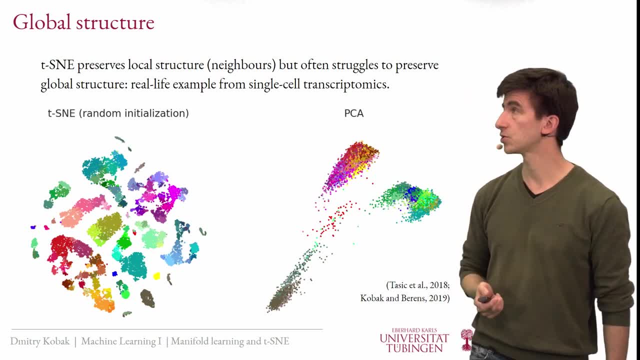 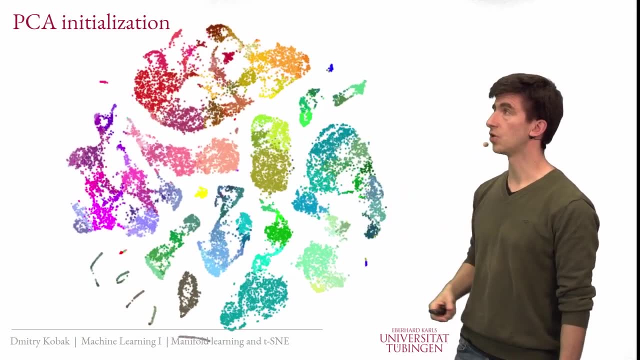 in the initialization and then we'll converge to whatever it converges. Let me show what happens. Start with PCA. here's early exaggeration phase. Now it's over and that's the normal t-SNEAR optimization phase, And here are all non-neural cells. 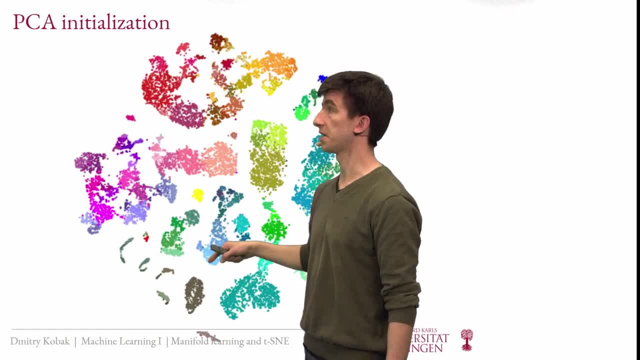 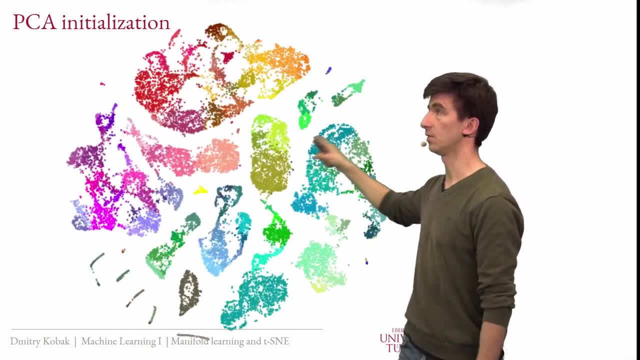 They started in this corner in the initialization and they of course end up in this part of the embedding together and all the excited tree cells will be on the right and they will still occupy the right part, like the bottom right part of this embedding in the end. 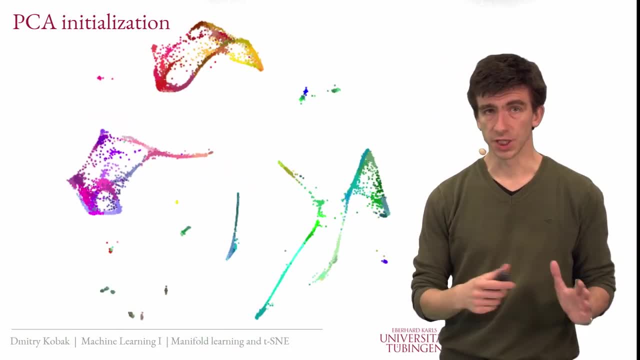 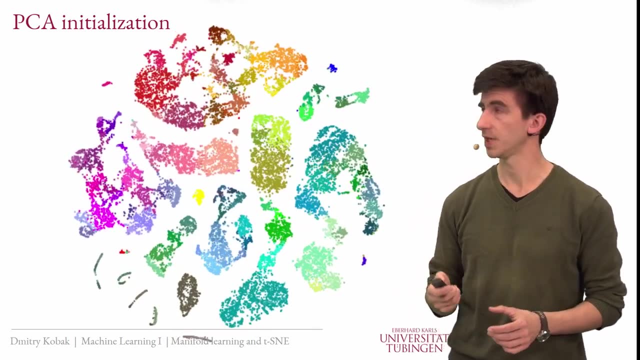 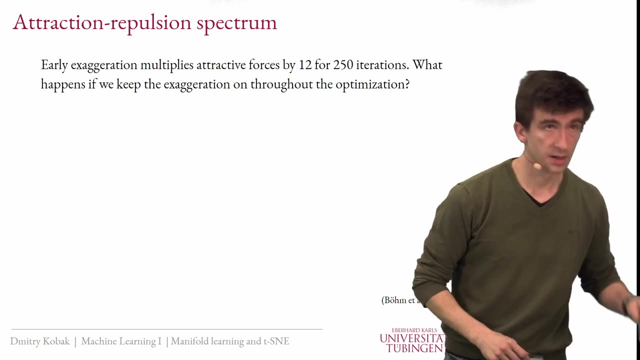 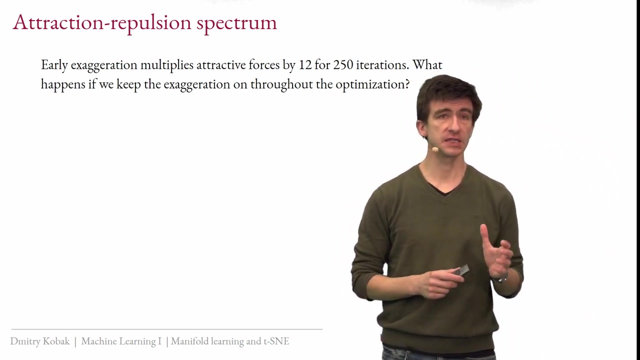 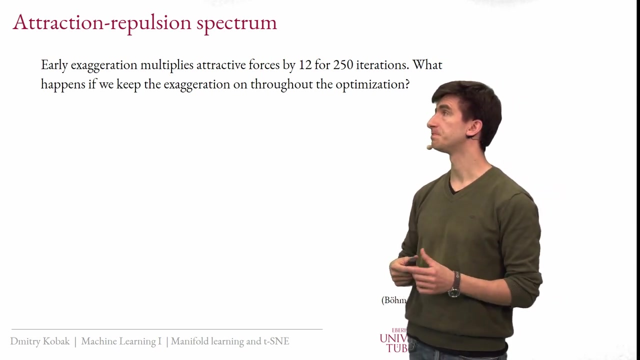 So again, general recommendation: always use informative initialization. In fact, modern t-SNEAR implementations do that by default. The last part that I want to cover today is to discuss the effect of exaggeration. So I mentioned before that early exaggeration. 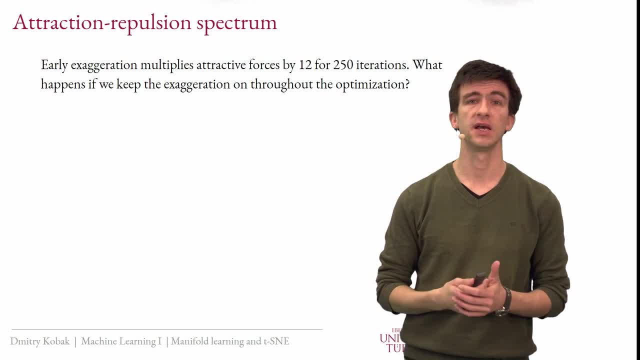 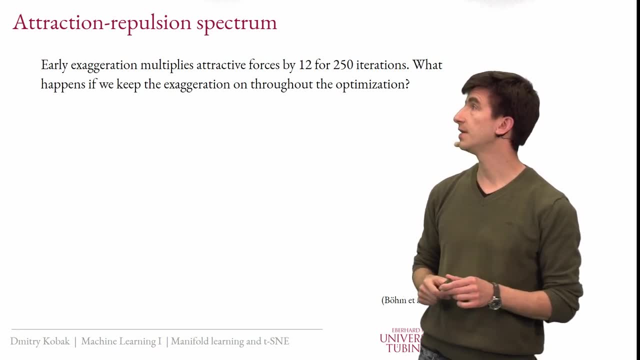 means multiplying attractive forces by some factor during the early iterations. very useful trick to get a better convergence. But what if we kept the exaggeration throughout the optimization? What if we don't switch it off in the end? And what if we don't use 12,? 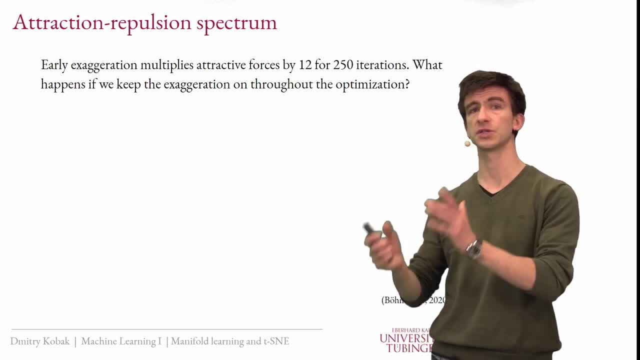 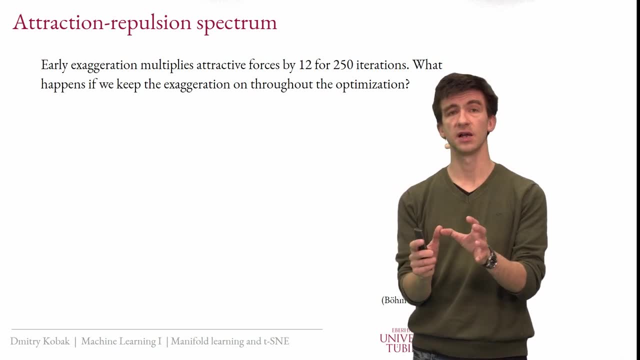 but different values and see what happens. Maybe you already noticed on the previous in my animations that this early exaggeration phase actually produces some interesting embeddings, And then I always switched early exaggeration off And in the end that's the t-SNEAR result. 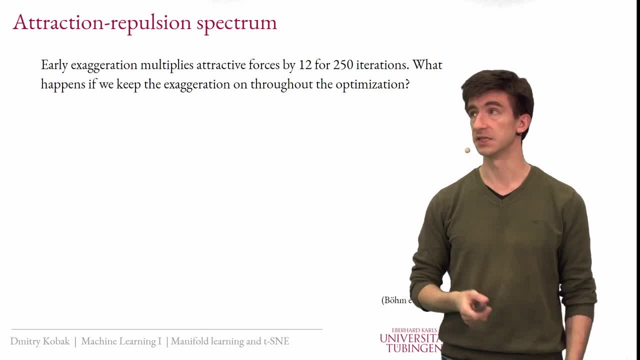 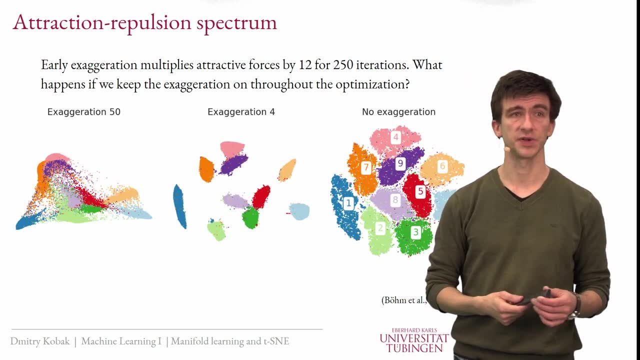 But maybe we can study what one gets with different exaggeration values, And indeed it turns out that one gets a very interesting family of embeddings. So let's discuss that briefly. So this again is a t-SNEAR- default t-SNEAR. 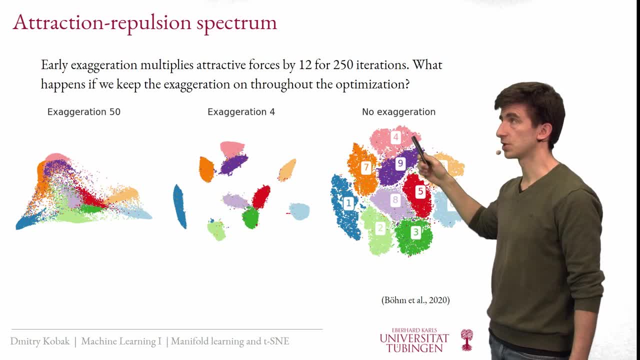 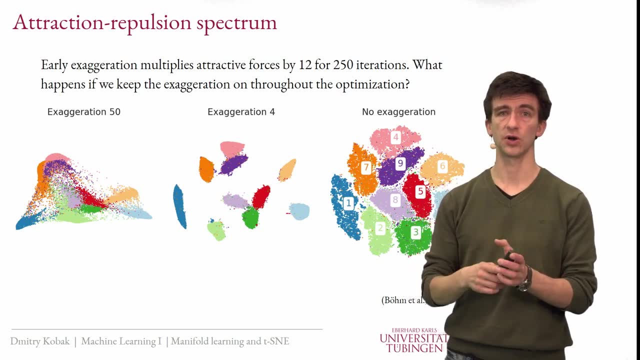 without any exaggeration. No, in the end I turn early exaggeration off and I'm left with this embedding. Now imagine that I'm running early exaggeration and then, after it's done, I keep on exaggeration of four until the end. 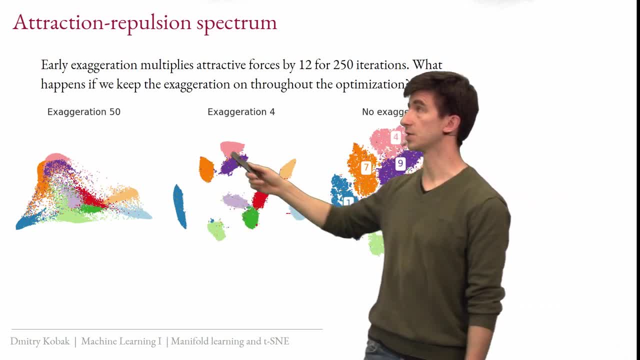 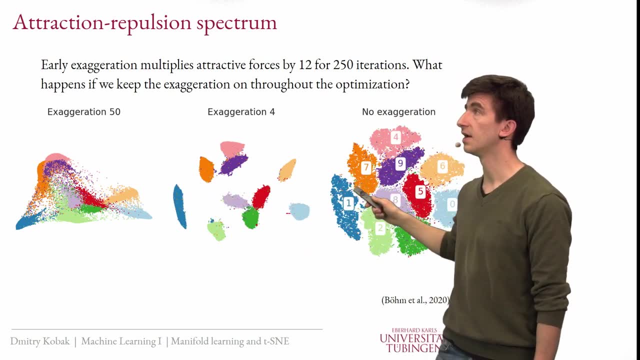 I will end with this embedding over here, And if I use exaggeration 30 throughout, I will get this embedding, This embedding on the left. So that's the spectrum of embeddings. here There's more attractive forces on the left. Attractive forces are stronger on this side. 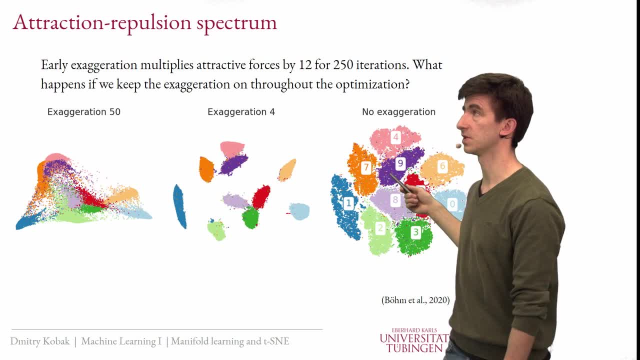 and the attractive forces are weaker, So the repulsion is stronger on the right side. That's why I call it attraction-repulsion balance, And it turns out that one gets very interesting embeddings along the way. For example, let's look here: 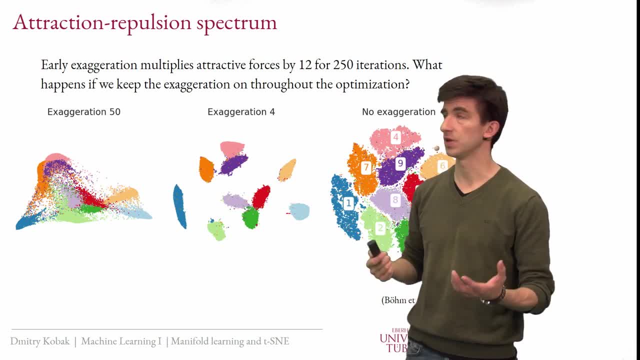 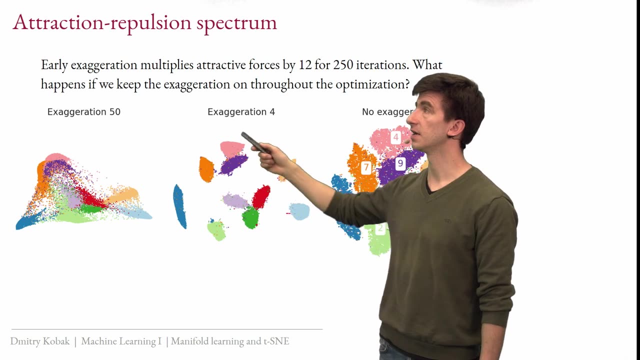 First feature is that there's a lot of white space. This can be useful to have- or I don't know- pleasing aesthetically or emphasize that these are different clusters. Another interesting feature of this embedding is that, for example, these three clusters are together. 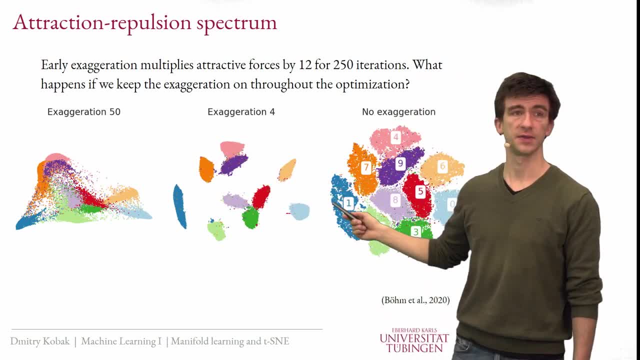 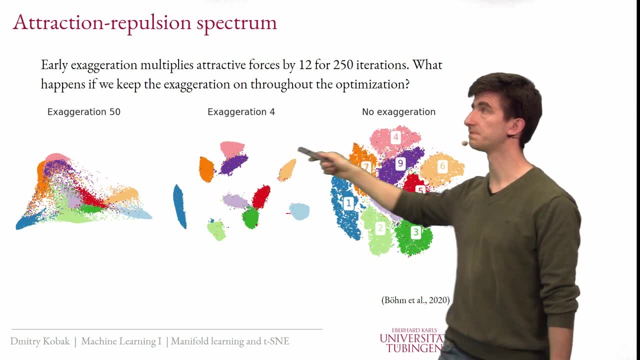 and these three as well. So if we look at what these three clusters are, then we see that this is eight, five and three which overlap in the pixel space, And the same is true for seven, nine and four over here. 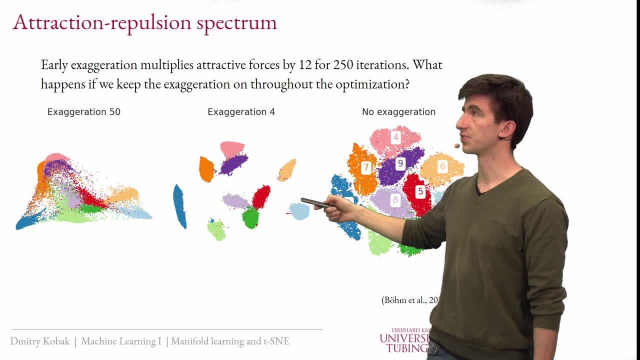 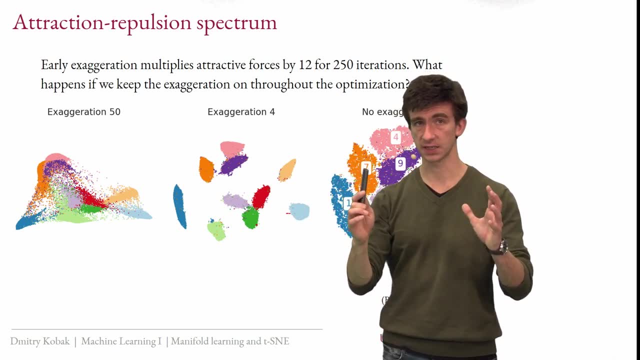 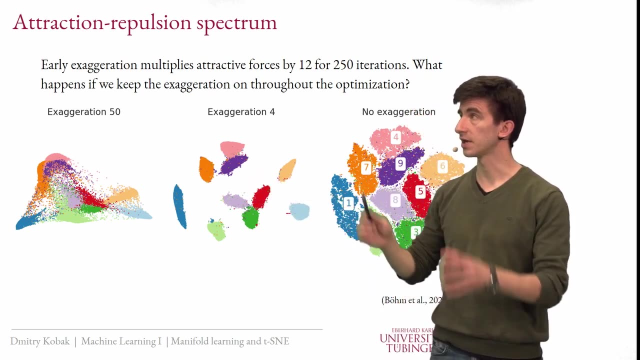 So we get larger clusters. This is a separation, but at the same time we see like larger groups of clusters that are connected by these nearest neighbor edges, They actually attract together stronger and collect in these larger groups And this makes a lot of sense. 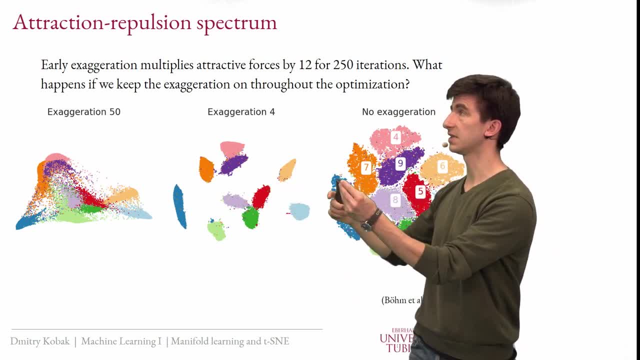 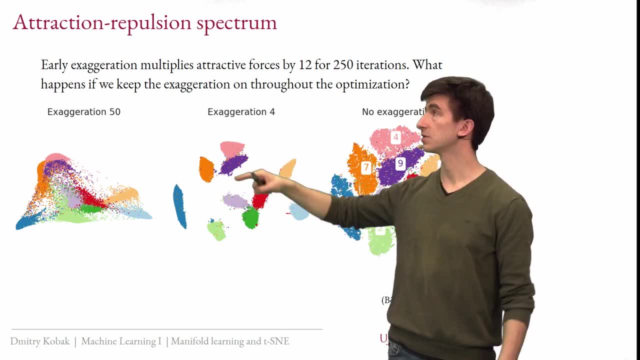 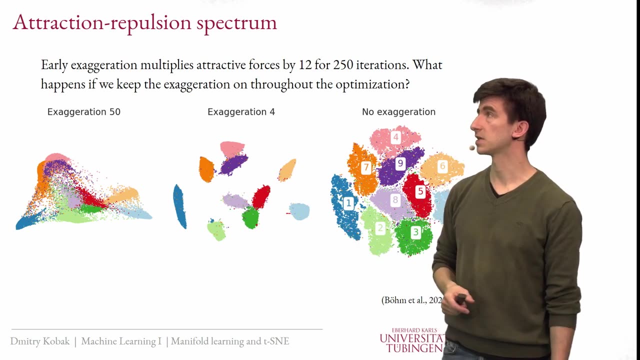 We increased the attraction here, right, So everything becomes denser. Points get closer to each other. These two digits, they feel also increased attraction. So they basically glue together like that: Okay, and the rest somehow balances out with repulsion. 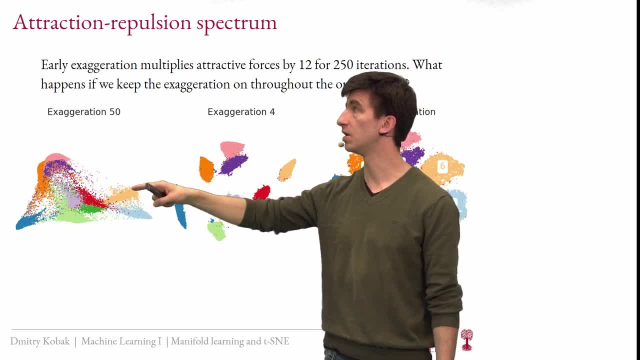 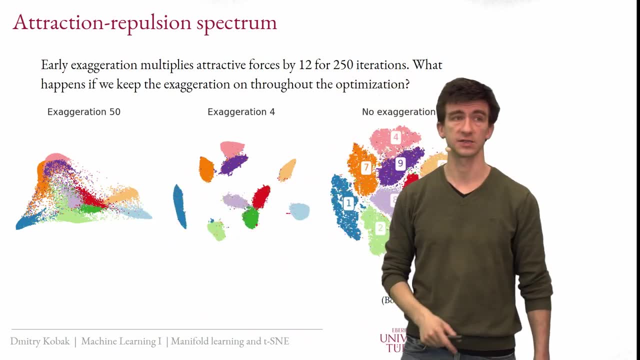 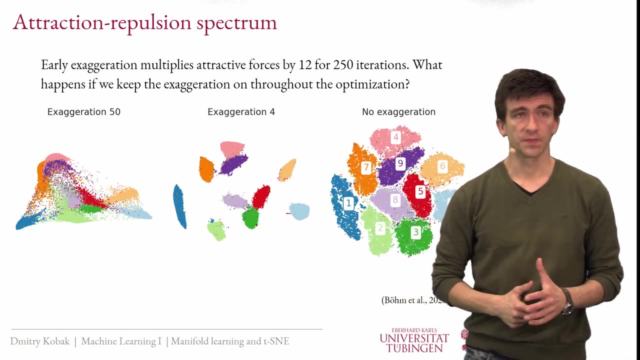 But if we increase the attractive forces even more, then all of them, all digits, will feel at least some attraction and will glue together in something that looks like that and does not have white space in between anymore. So we analyzed a bunch of different data sets. 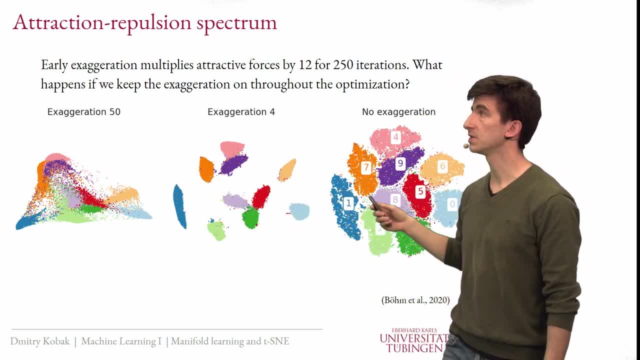 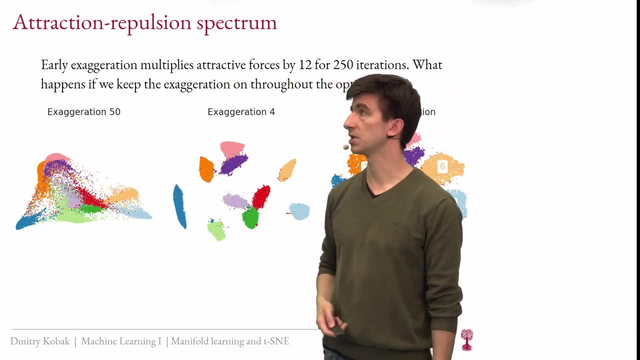 which you can look at. This is preprint from last year and showed that this always happens And you always get more. So we interpret this as having more continuous structures here on the left and more discrete structures emphasized here on the right. You don't have a lot of continuous structures in the MNIST data. 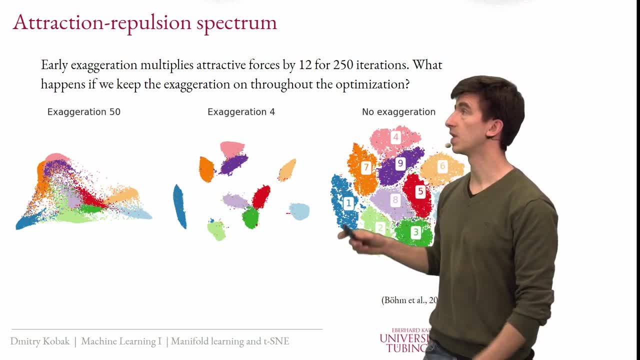 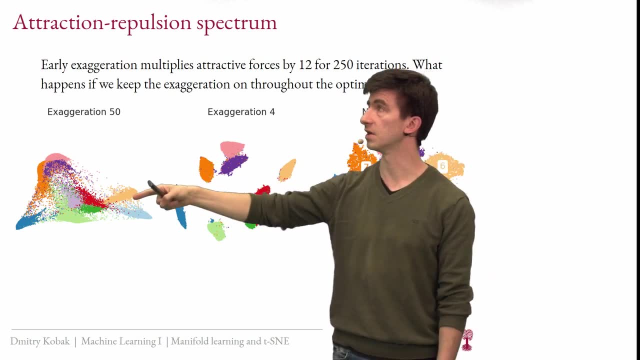 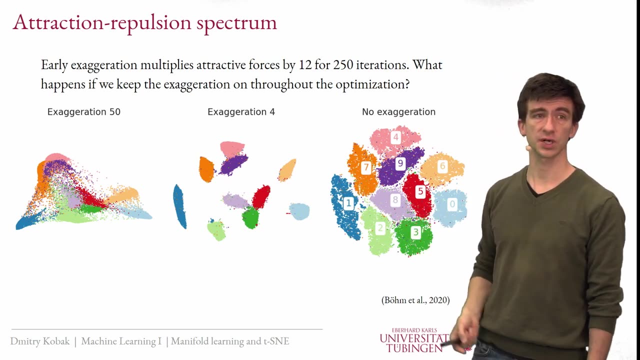 So I will show on the next slide another data set where this is clearer. But already in MNIST it's clear that we're getting at least more like a larger scale structures emphasized here when we increase the attraction, Whereas you can say that this emphasizes some very local structure more precisely. 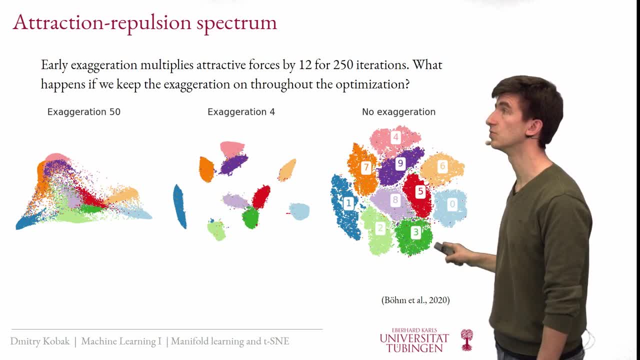 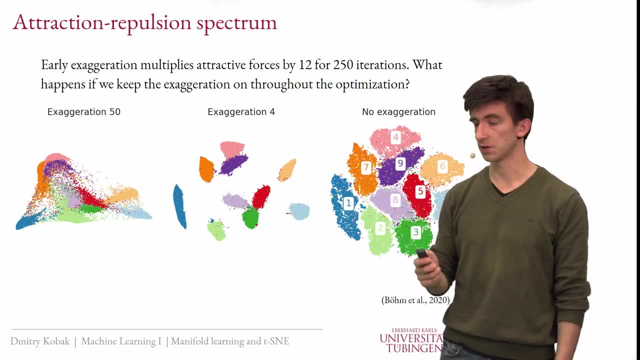 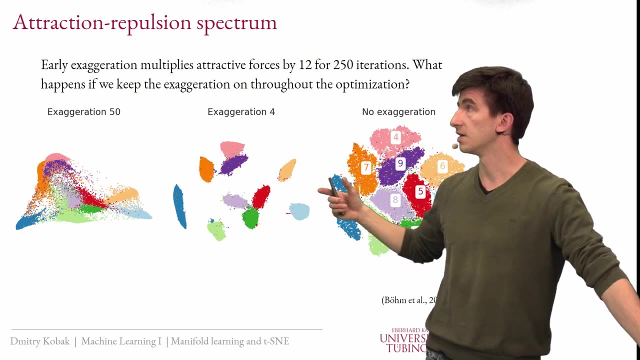 For example, the threes seem to split a little bit in two different groups in this embedding here, And this is something that is completely lost over here because attraction is stronger. So one point is here that actually this is an interesting hyperparameter, At least empirically. it produces useful embeddings often. 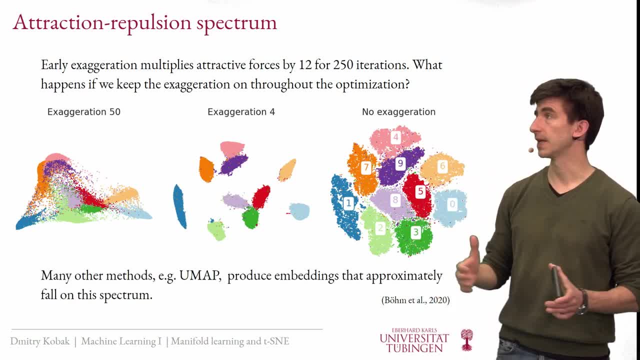 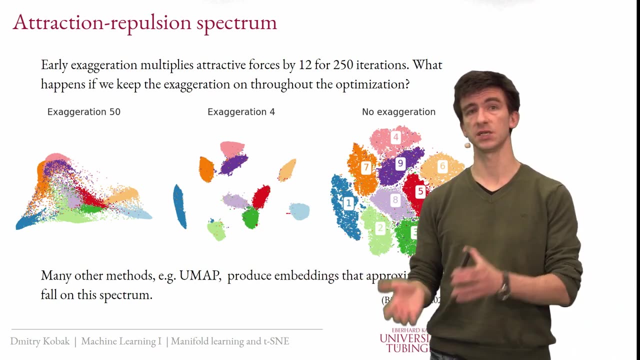 But its separate point is that it turns out- surprisingly maybe- that many or several other algorithms that were more recently developed. in the last several years they produced embeddings that are very similar to somewhere on the spectrum. So UMAP, for example, is a method very related to t-SNE. 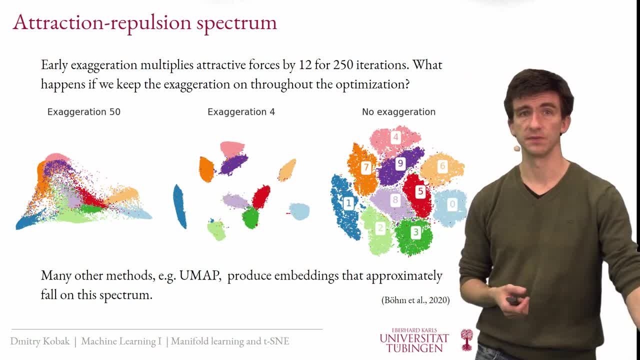 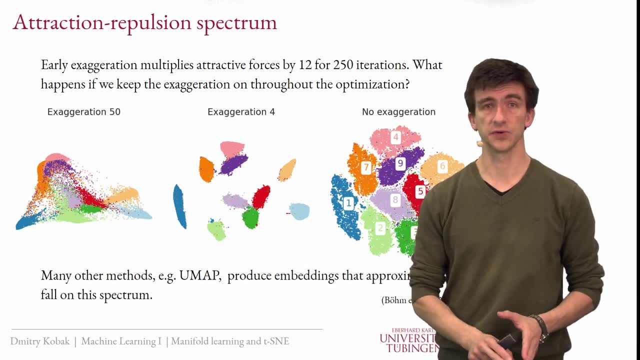 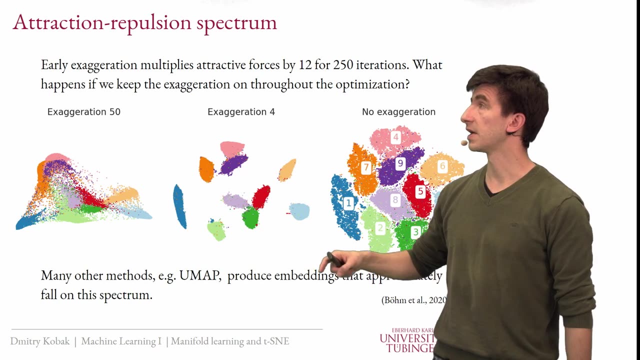 but it works very differently. It involves some stochastic optimization and so on. I'm not going to present it in detail to explain how it works. It appeared a few years ago and became very popular in some fields, for example in single cell. community uses UMAP a lot now. 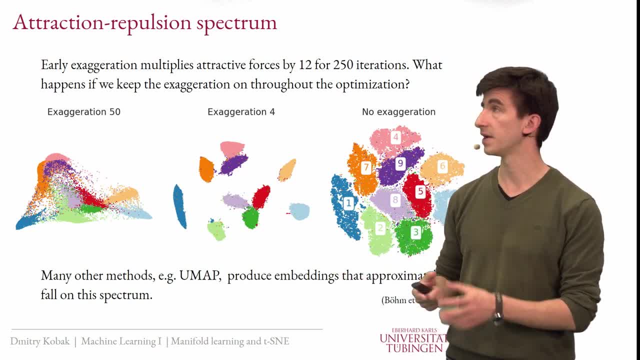 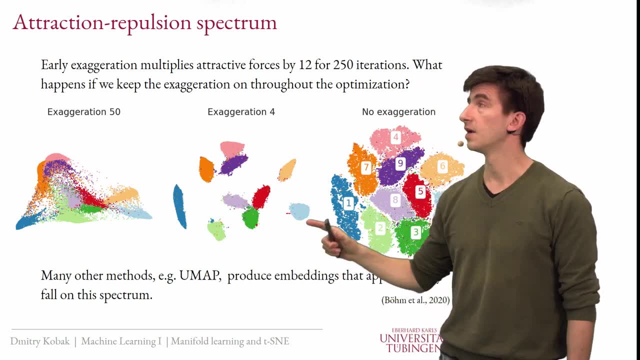 So it works differently. but once you run it and you look at the embedding, it turns out that UMAP of MNIST looks almost identical to this picture. That's basically UMAP of MNIST give or take, And this happens not only for MNIST. 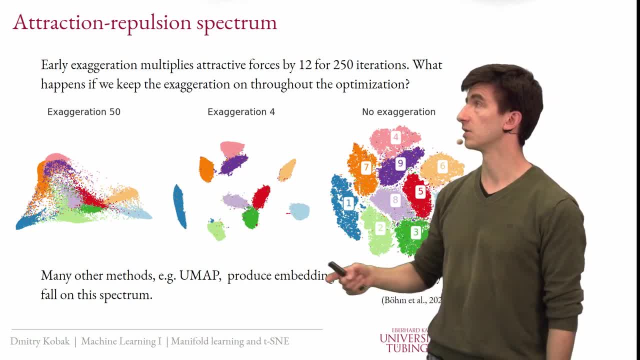 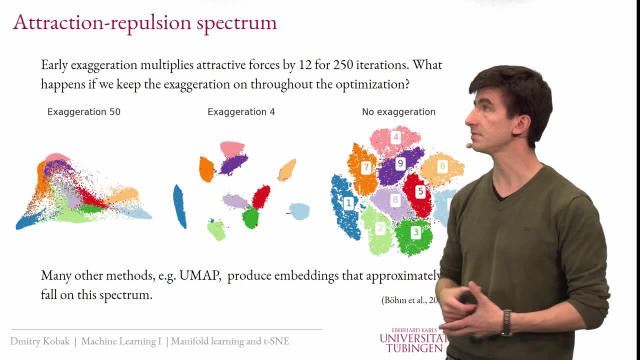 but across the range of very different datasets, And one can analyze it mathematically- the loss function of UMAP- and show that actually it does look very similar to t-SNE, but attraction is stronger, And this is true not only for UMAP but for several other methods. 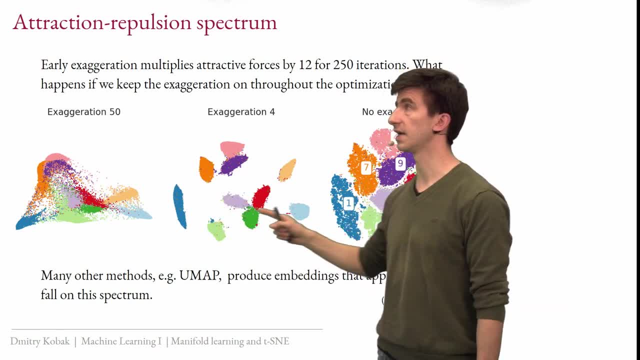 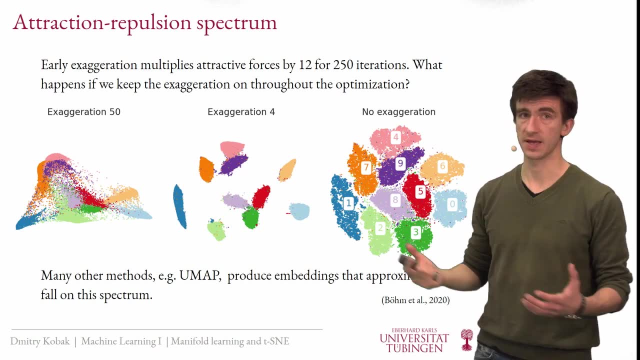 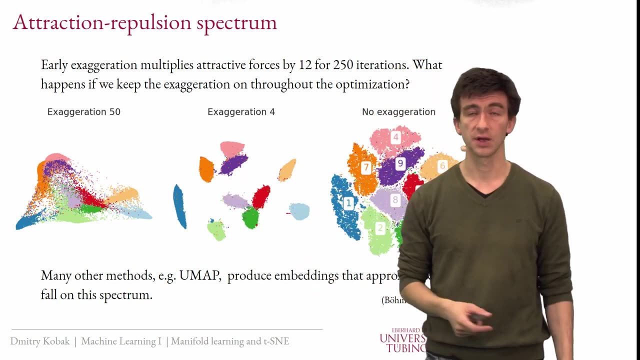 We see that actually they produce outcomes that are somewhere on the spectrum, always to the left of t-SNE. For the methods I know, some correspond to exaggeration 4, maybe some other methods correspond to exaggeration 30, but they live on the spectrum. 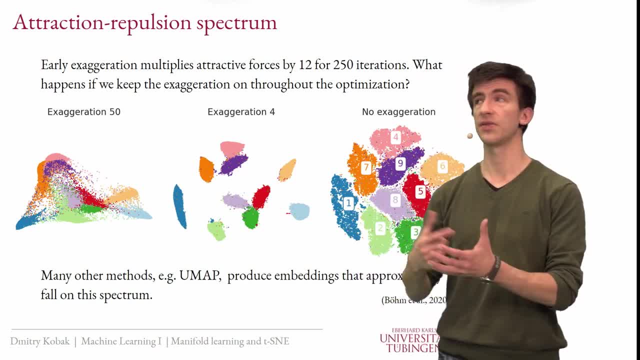 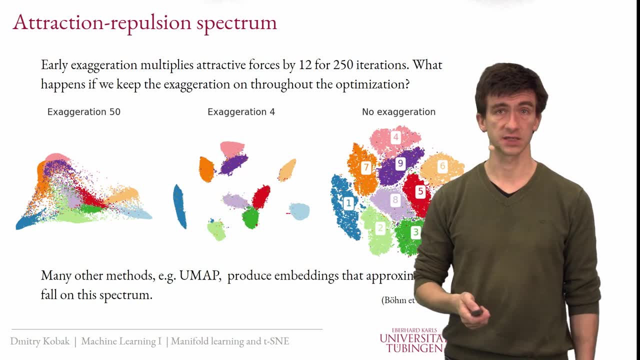 So that's pretty interesting, even though the methods may be pretty different. But in the end that's the, that's the meaningful family of embeddings that one seems to be getting here with different algorithms, And here's my last example for today. 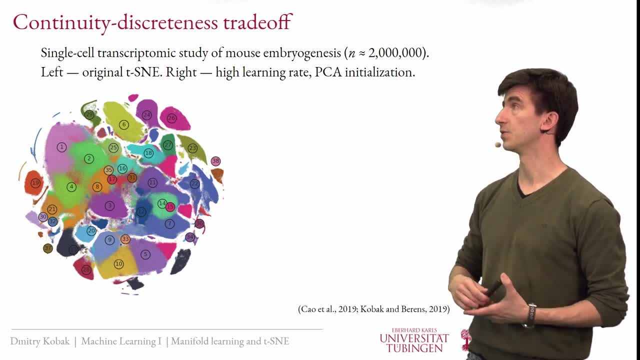 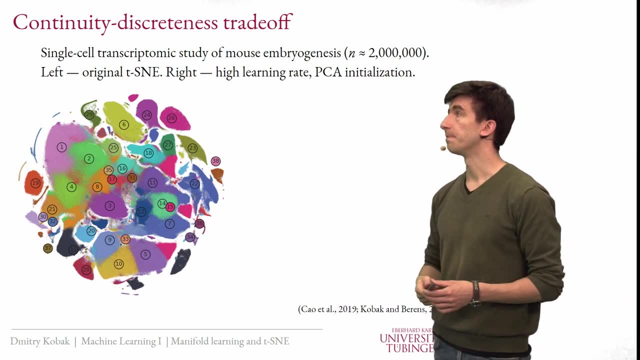 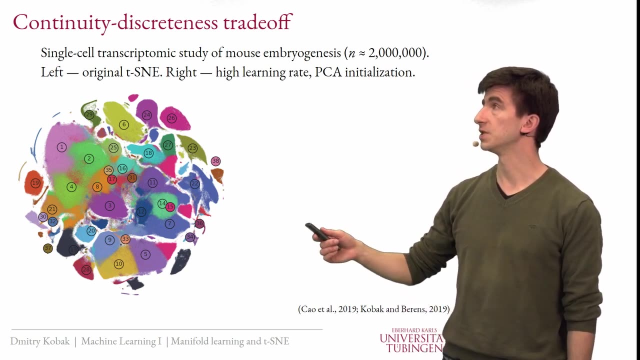 This is a very large single-cell transcriptomic study with 2 million cells. Cells come from mouse embryos during development, So that's the original citation and we use this dataset in that paper to play around with for t-SNE And here. 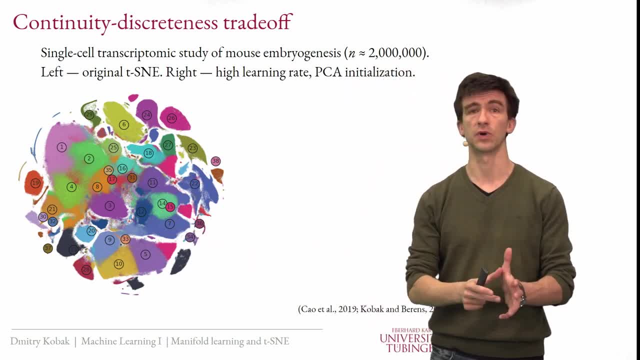 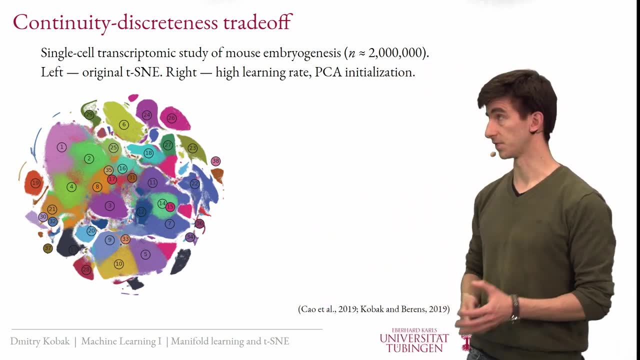 I'm showing you the t-SNE plot that is actually taken from the original paper. So original authors did t-SNE. That's their t-SNE. They also clustered the data in a bunch of different clusters and that's the colors that I'm showing here. 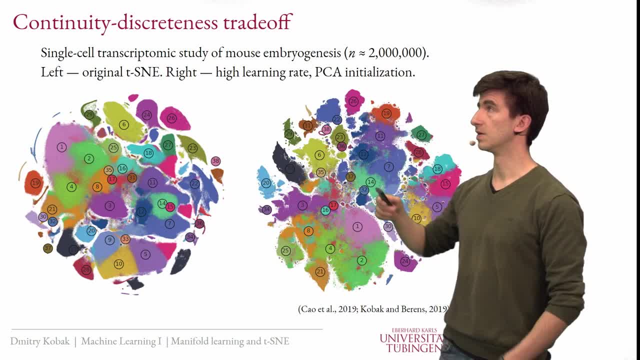 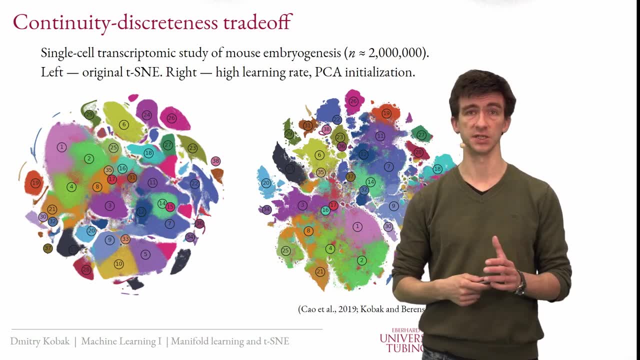 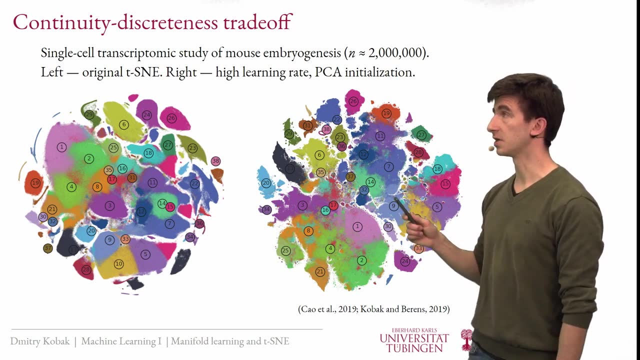 If one does the t-SNE using high enough learning rate and the PCA initialization- so high enough learning rate, as I briefly mentioned before, is needed for the early exaggeration to work properly- then one gets a picture like that. And if you look closely at this, 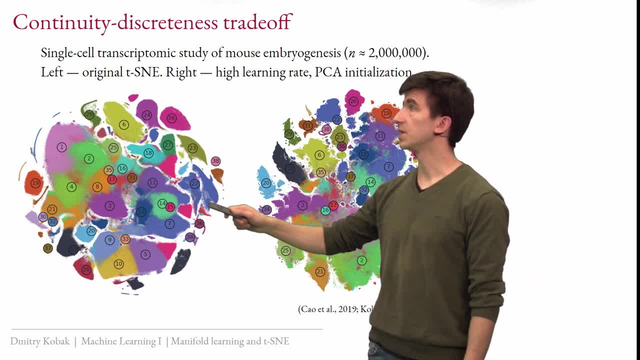 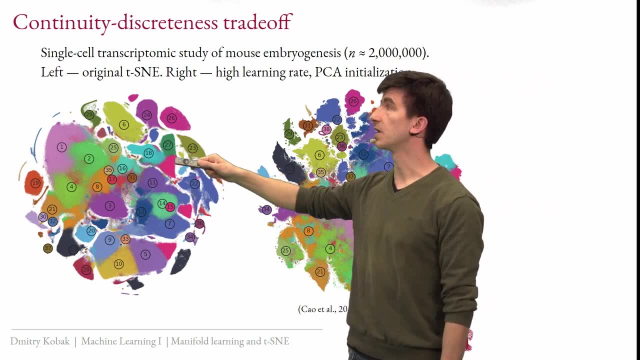 you will see that this is a much better result than on the left. For example, there is this pink cluster over here, number 15, I think, which is here split in three parts: one, two and three. They belong to the same cluster. 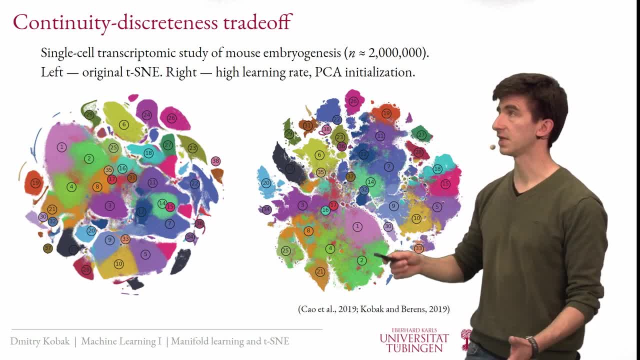 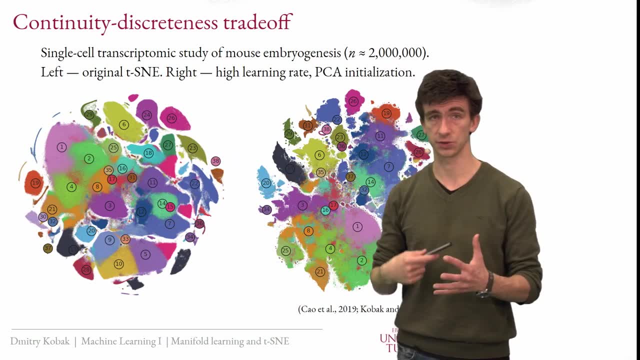 but they appear as three different parts here. This doesn't make sense and that's the bad. local minimum, The early exaggeration was not strong enough or the learning rate during this phase was not strong enough for these to collect together. So if we set the hyperparameters right, 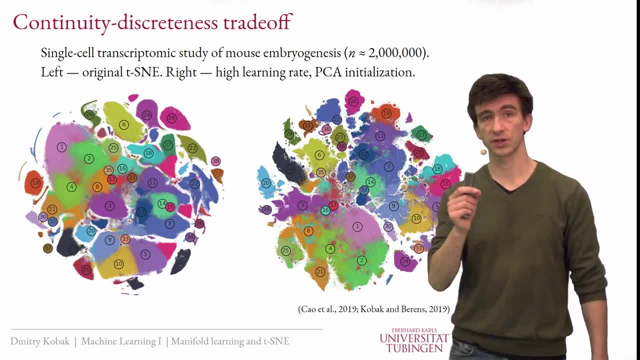 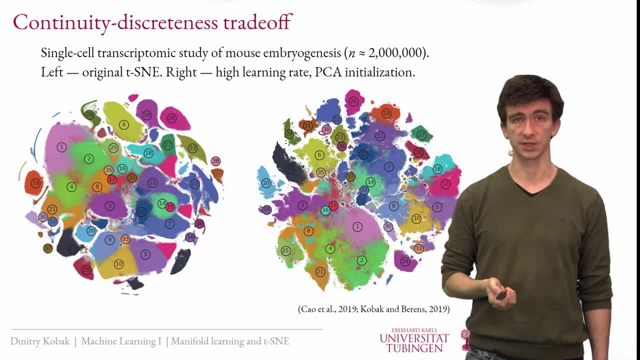 then we get this result, which is much better. But that's not the most interesting part here. The most interesting part, I think, is what happens if you increase the exaggeration here: the final, not the early exaggeration, but the exaggeration overall. 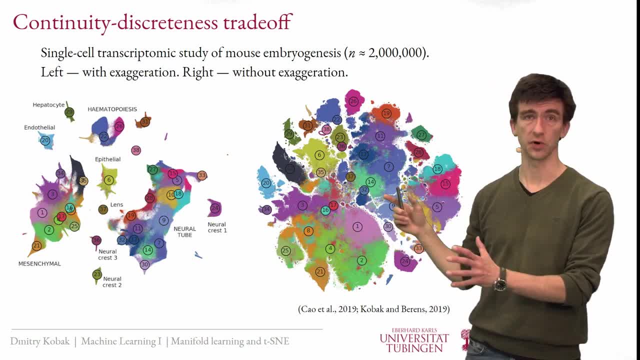 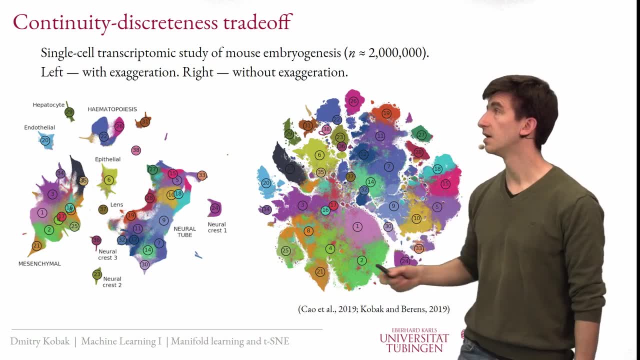 and then we get this thing. So this is, let's say, the default t-SNE, with no exaggeration in the end, but the hyperparameters, the optimization parameters, set correctly, And this is what you get if you use exaggeration four. 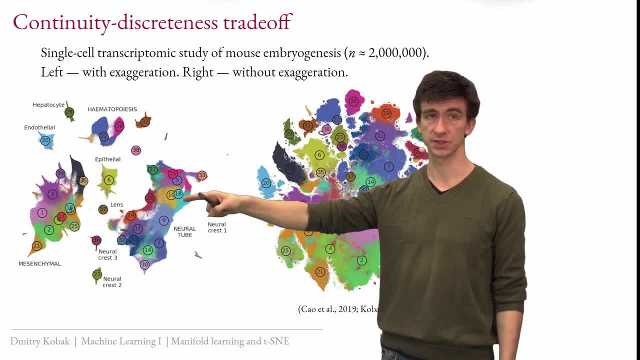 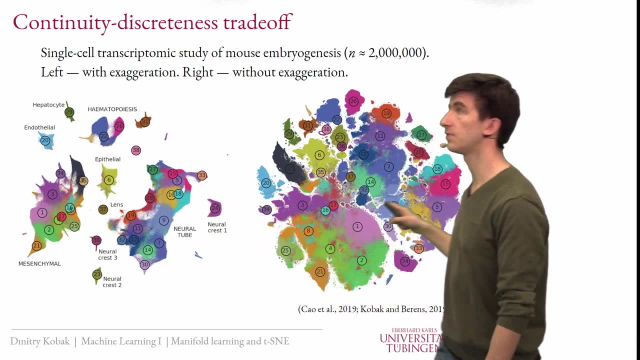 And, incidentally, if you use UMAP for this data, you will get a very similar result to that. So, and what happens here is that there are larger structures here appearing, So here, if you look at this, you have no idea that there is maybe two very large continents in this data. 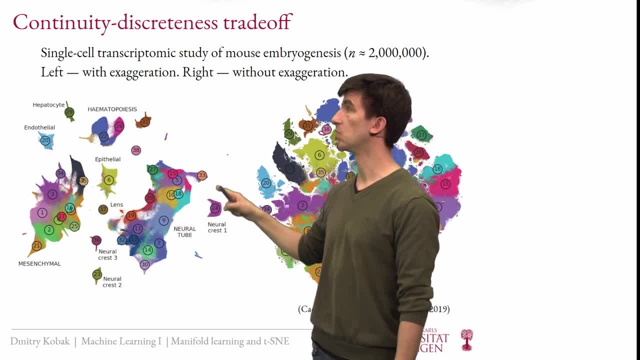 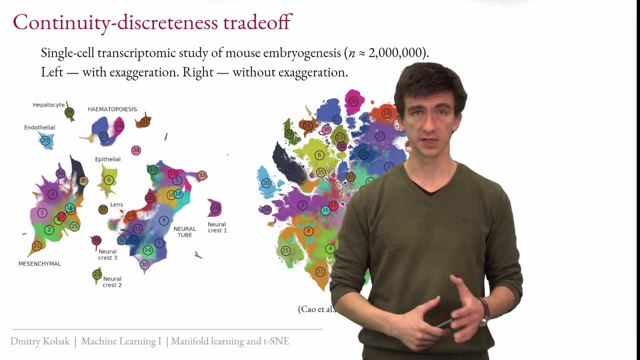 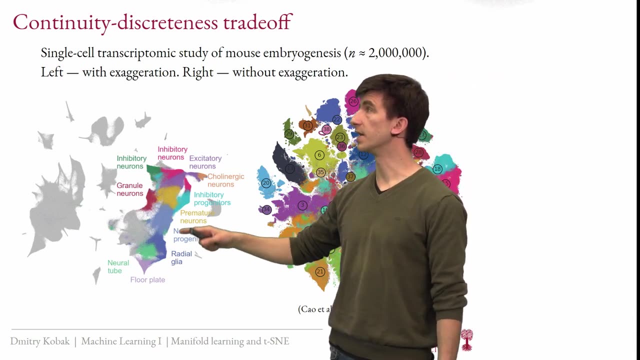 whereas it's super apparent in here. And if we look at this, this slightly larger continent, then these are actually cells that correspond to neural development in the mouse embryo And, moreover, if I show you the labels for all clusters that have something to do with neurons, 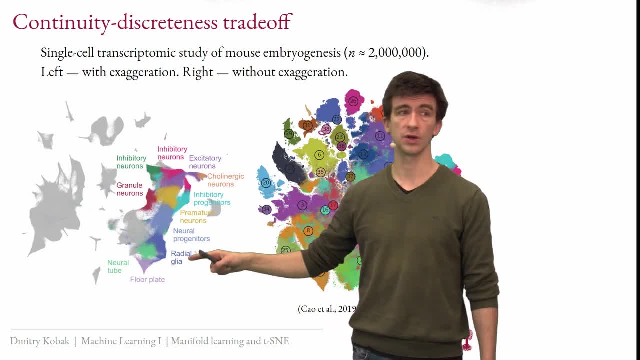 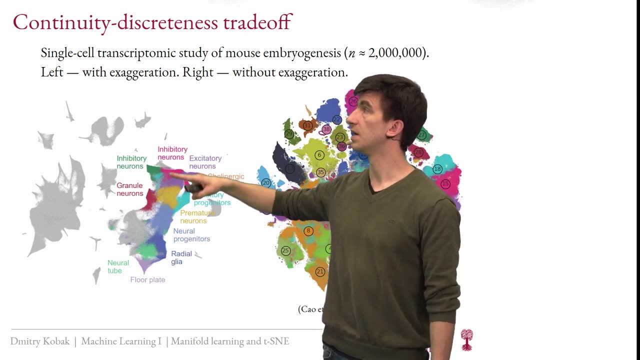 you will see that there is a progression from a very early so-called glial cells that then give rise to neural progenitors, then later develop into mature neurons. So you can see that there is a neural development from the bottom up here to the top. 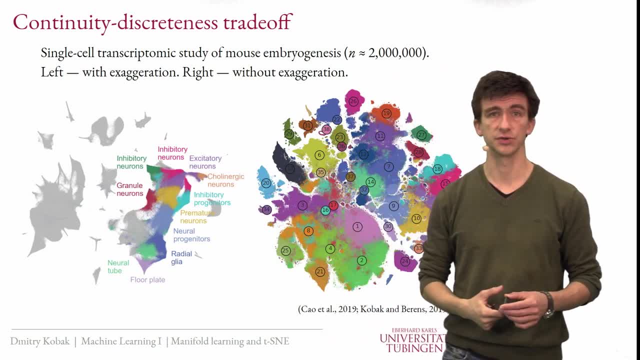 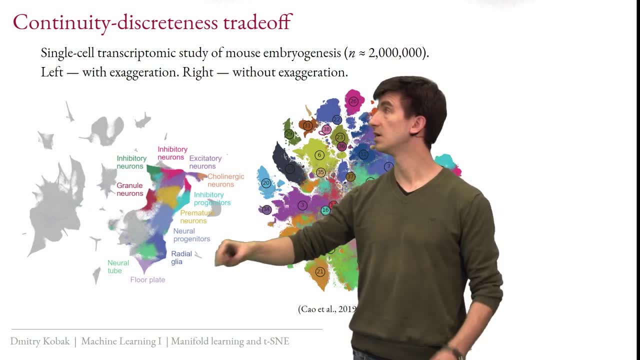 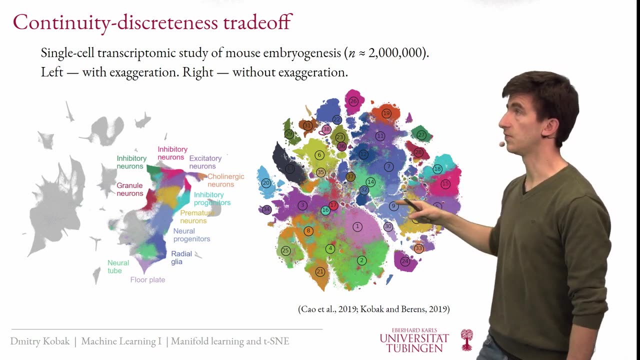 and that's just the progression of the cells during the mouse embryo genesis. So that's pretty cool that we see this one-dimensional time axis essentially in this embedding, And the interesting thing is that you cannot see it here If you know where to look. 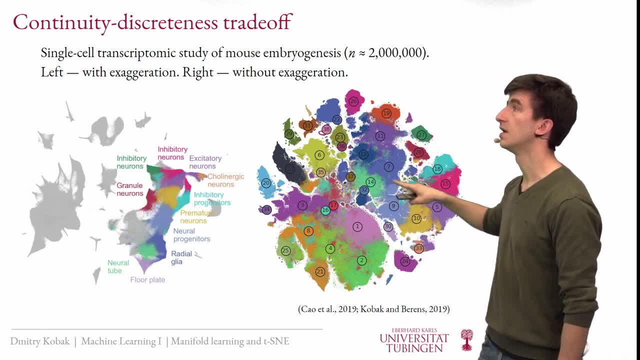 then you can see that in fact, this progression starts somewhere here and then goes like that to this orange cluster and on top here. So this is this time axis of neural development. But if you don't know that, you will never see this here. 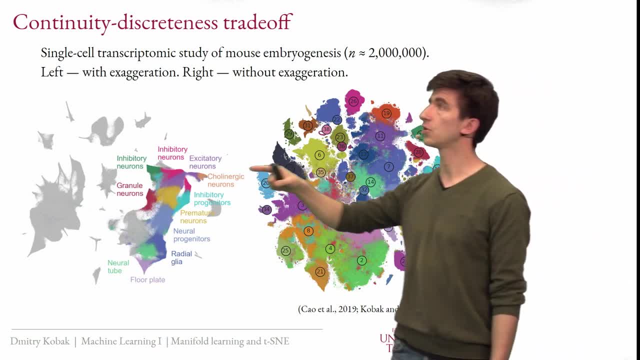 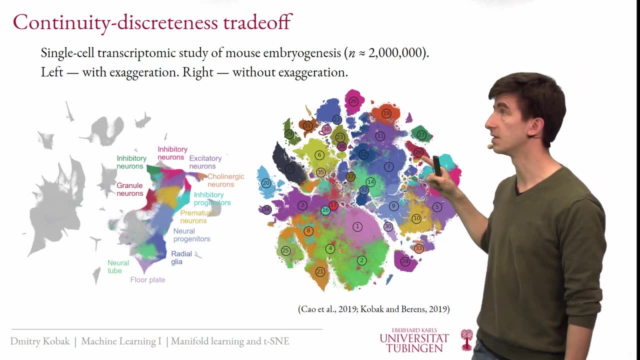 On the other hand, some things can be seen on the right that cannot be seen on the left. For example, there are all these small islands here, which I don't know if they are biologically meaningful or not, but the data suggests that there are some small fine clusters in the data. 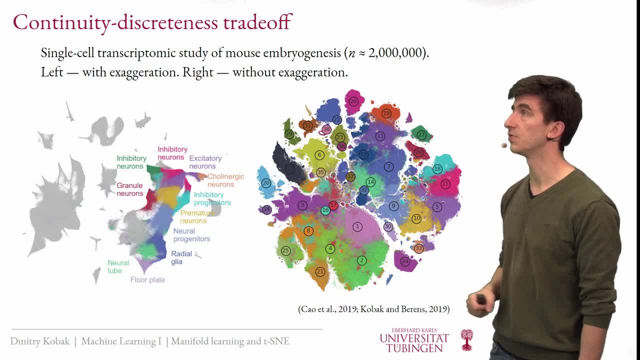 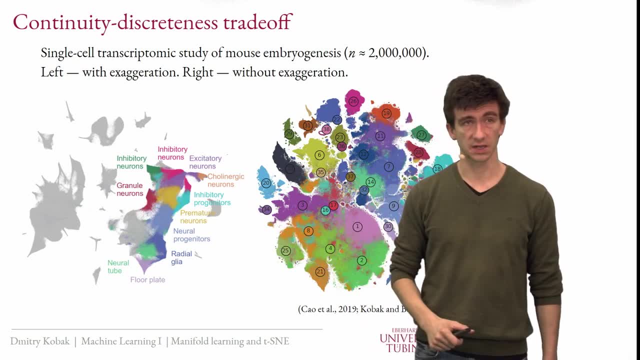 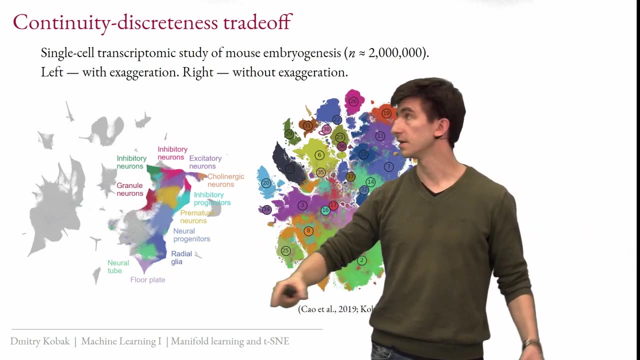 that that one sees in the actual default t-SNE over here, But here, with increased attraction, this is just gets collapsed together. So you don't see fine clusters anymore, but you see actually larger scale structures. That is interesting, And in this case 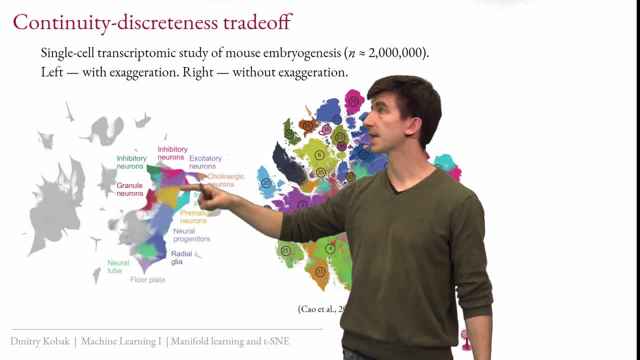 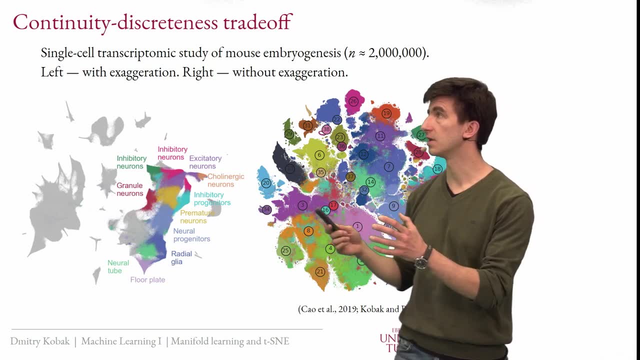 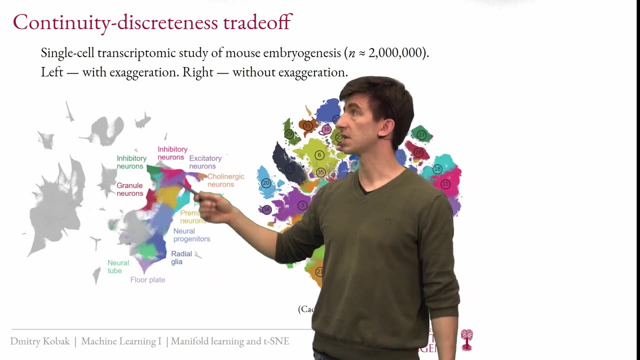 we know from biological knowledge that a priori knowledge that there should be this continuous sub manifold in the original data. So I think the way to think about that is the continuity, discreteness trade-off that one gets with higher attraction. You emphasize continuous sub manifolds with higher repulsion. 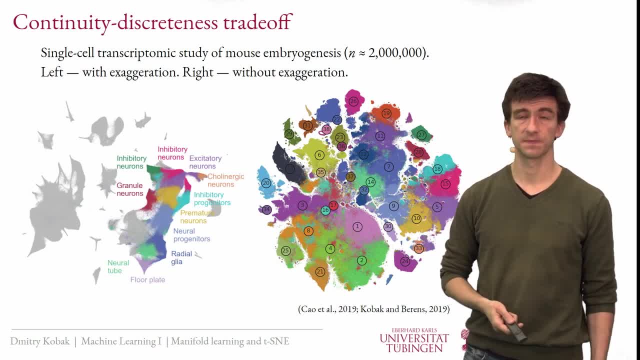 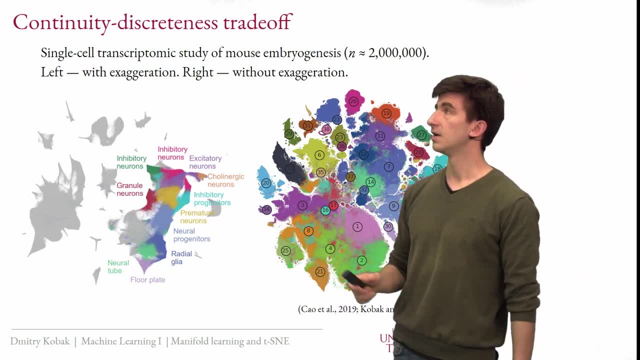 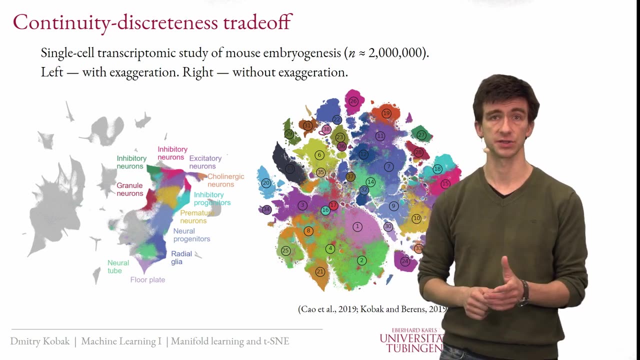 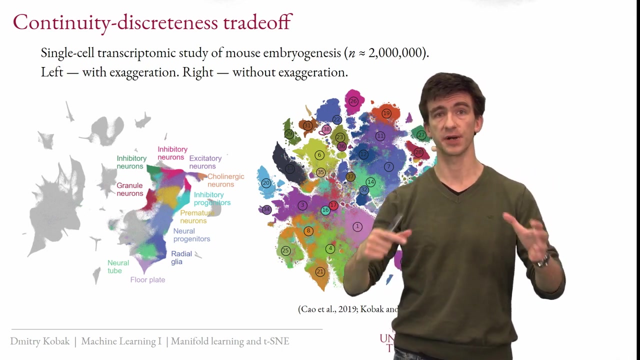 You get more cluster structure emphasized. And I'm going to end here on this slide, but I will say in the end that actually I think this field of two-dimensional embeddings and visualization of complicated, high dimensional data- by complicated I mean data that have some maybe continuous sub manifold in it-